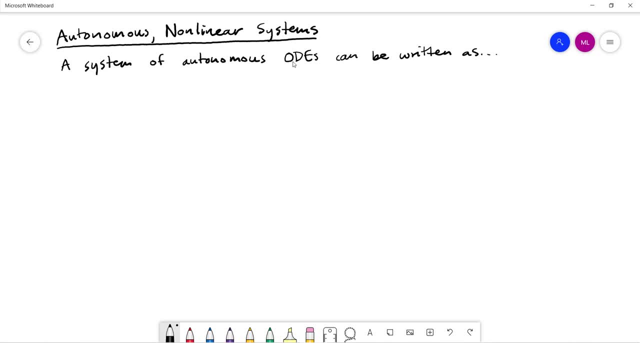 So and again. just a reminder: autonomous simply means that the functions that show up are not explicitly. there's no coefficients that are explicitly a function of the independent variable, just of the variables that we're actually trying to solve for. So basically, in this case we have a dx dt that 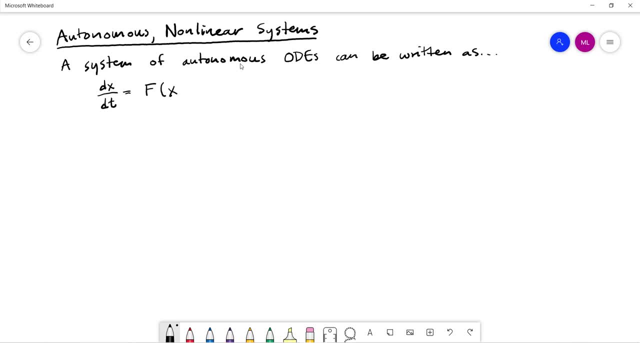 we're trying to solve for and that dx dt is given by some function, potentially, of x and y, And we also have a dy dt that we're trying to solve for and that's some other function of x and y. but what makes them autonomous is, you'll notice over here, these two functions do not. 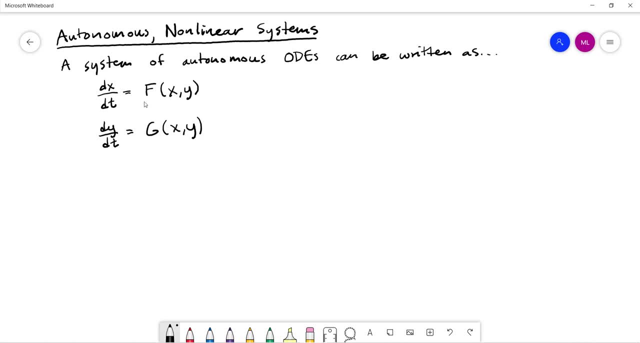 explicitly depend on t anywhere. they're only functions of x and y, which are also the variables we happen to be trying to solve for. so that's what makes it autonomous if this equation is linear. so if the f and g turn out to be linear equations. so if it's linear. 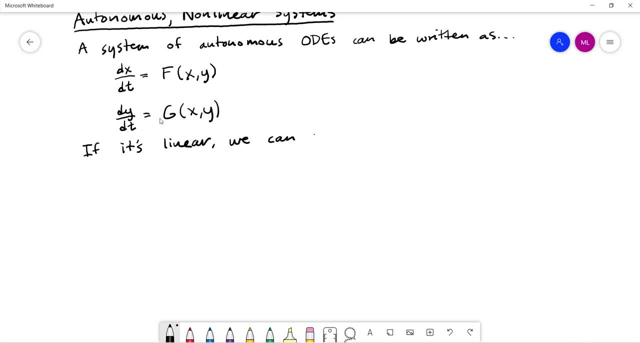 we can write this much more simply as, basically, dx, dt, where that x is now the vector x, containing both x and y, equals a times x. so these are the types of problems that we were doing in the previous sections. so this is our matrix form of that equation, if it's non-linear. 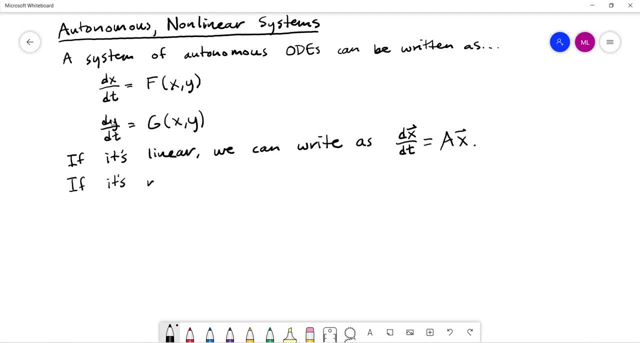 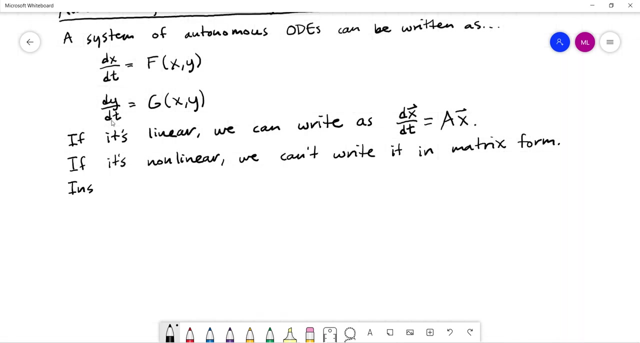 you. so if our system is nonlinear, we can't write it in matrix form. it's not that simple. the best we can do is write it as follows: so we can still kind of use vectors to make it a little bit shorthand, but it's not going to be a 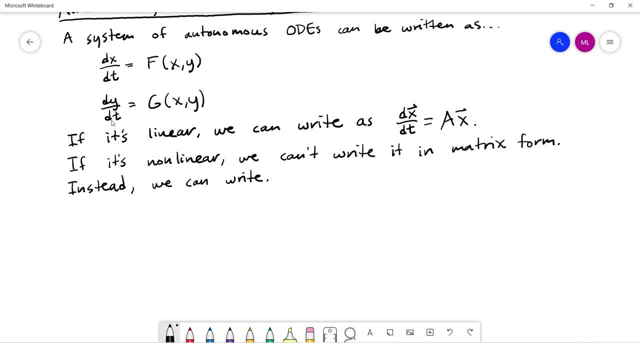 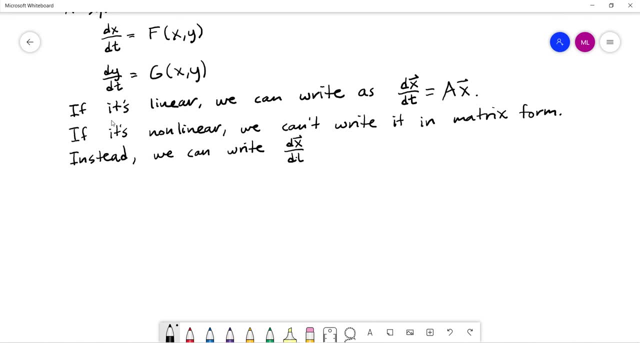 matrix we can write basically that are now. we'll just do it on the same line here. DX, DT is equal to. this is going to look kind of weird. a vector F of that's a function of the vector X, so a vector function of a vector variable and this: 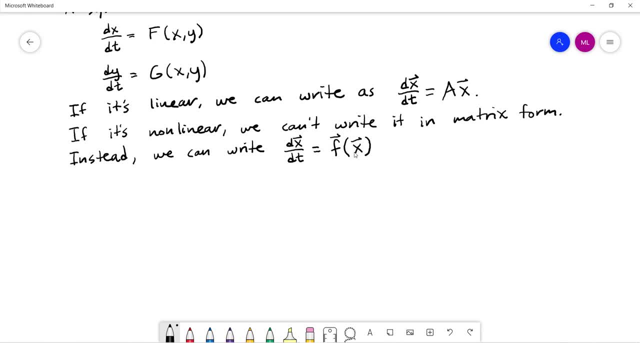 can get confusing. I don't want to go a ton into this, but what I really want to do is: I want to make sure that we have a vector function, that's a function of a vector variable, and this can get confusing. I don't want to go a ton into this, but what I really want to do 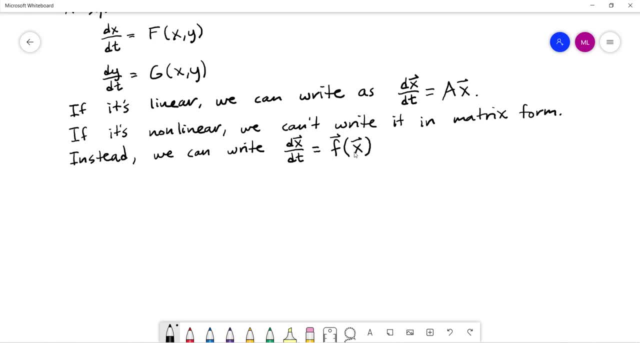 is break it down into a way. the only types of problems that we're going to be looking at are a little bit simpler than this, so we can write it like this: if it's what we call almost linear, this is gonna be what we're gonna focus on, so 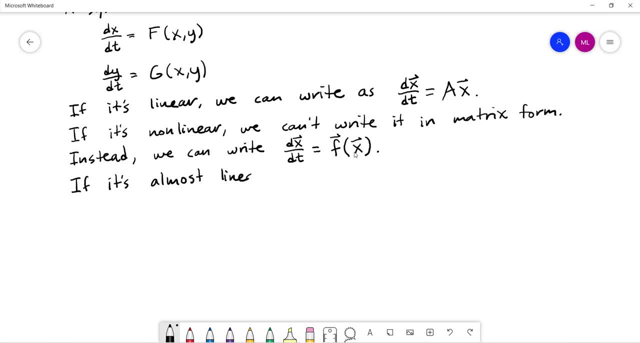 if it's almost linear. what we can do is basically break the F into a part that's linear that looks like this: that can be written using a matrix plus a part that's nonlinear. so if it has some parts that are kind of linear and some parts that are nonlinear that go into into the whole thing, and again we'll 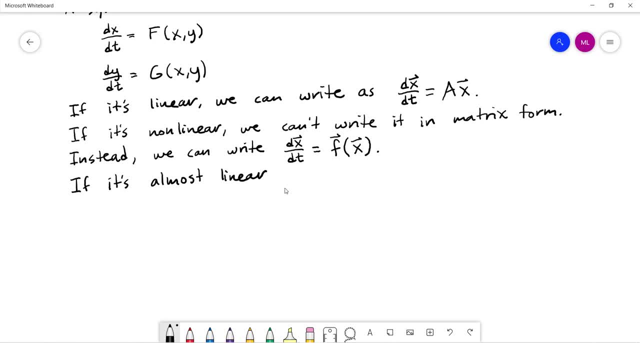 look at an actual example of this later. but if it's almost linear, we can write that DX- DT is gonna be equal to some portion that is linear plus some other portion. I'll call it G of X. so this piece looks like the nonlinear piece that we 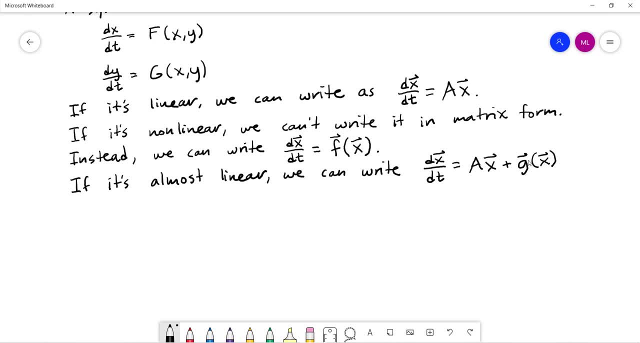 have up here, but maybe we've broken this down into two pieces apart. that is linear, and then this is the trouble piece, that's giving us the nonlinear terms, where this term is small, near any critical points that we have. so where G of X and really, if you want to think about it, we're talking about, like the 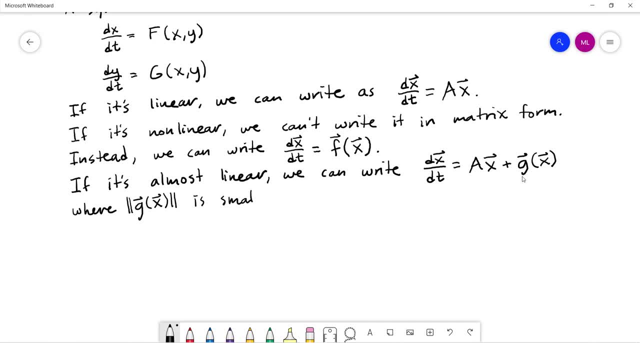 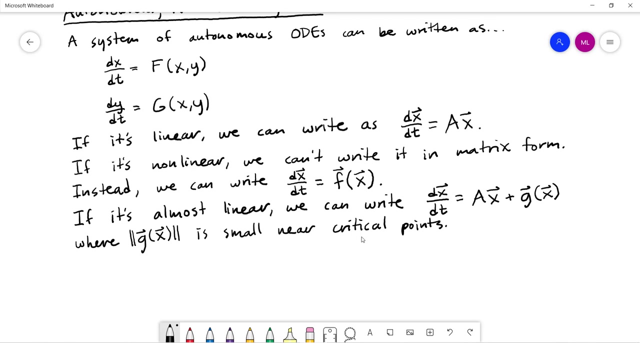 magnitude of G of X is small. here the critical point- and you'll remember this term, critical points- showed up early on when we were dealing with autonomous equations that weren't systems. basically, critical points, also called equilibrium points, are essentially points where the right-hand side, essentially, is going to zero. so 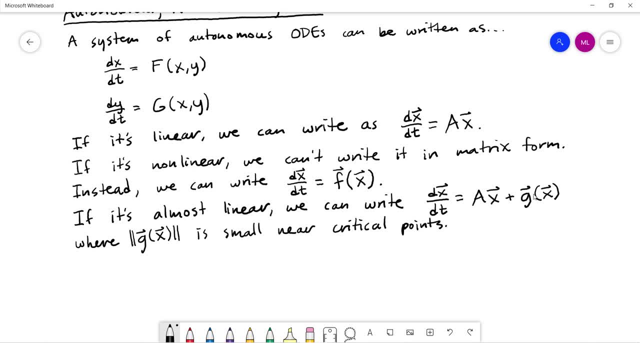 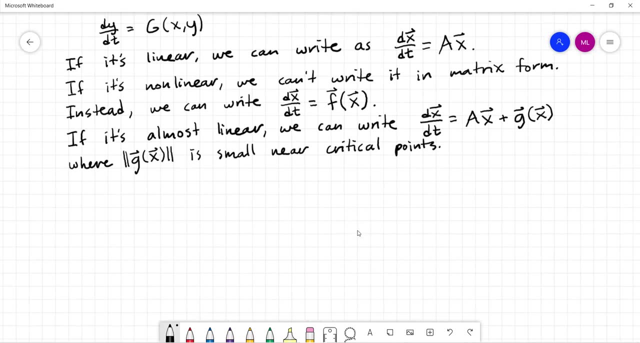 that's kind of the idea here: when, when is this side going to go to zero? that's going to be the what we're going to call our critical points, and so let's get a sense of how we can actually handle these problems. so let me give you 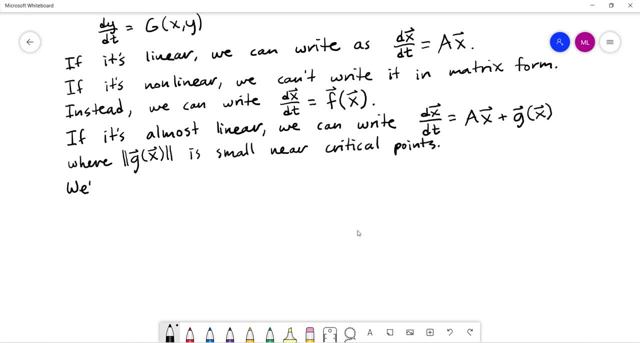 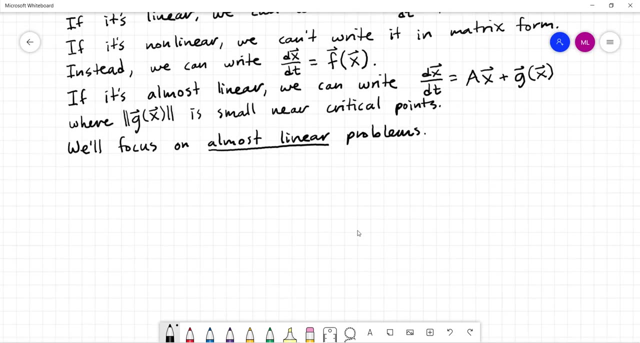 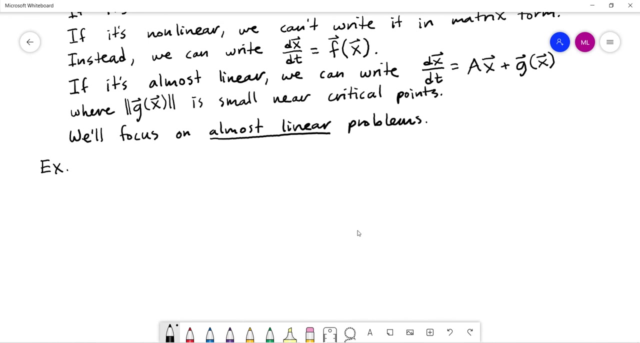 an example of an almost linear problem. so we'll focus only on these almost linear problems, and there are a lot of them. so almost linear, okay. so, for example, let's say I've got something that looks like this: it's dx- dt equals something, dy- dt equals. 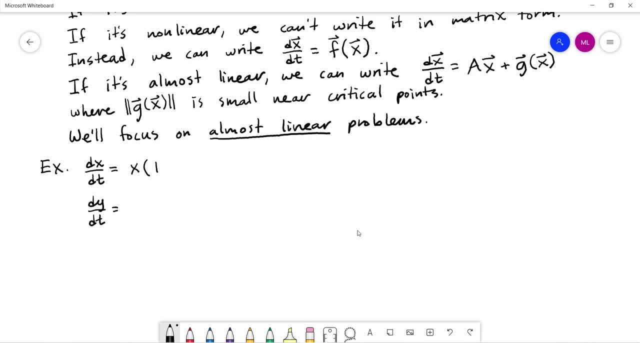 something. and let's say that dx dt looks like x times 1 minus y and that dy dt looks like y times 2 minus x. notice this is non-linear. if we were to actually distribute through, this, first term is x minus xy and the second one is 2y minus xy and you can see the non-linearity. 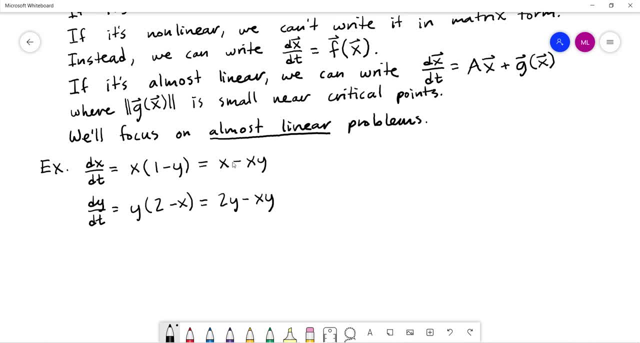 right here. it's not some function of x or some coefficient times x plus some other coefficient times y. instead we have this combination, this xy term, where they're mixed together. so this is that term, that's the non-linear part, whereas this part over here is fine, this part is linear. 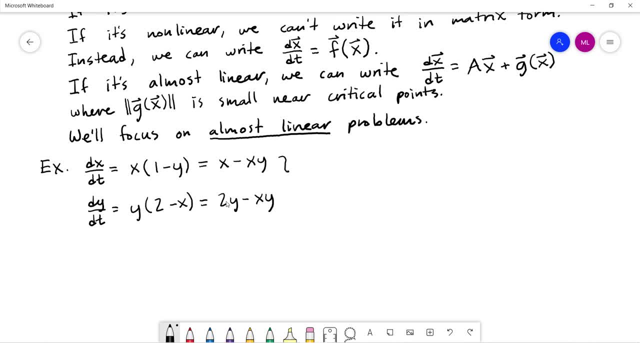 so we could think of writing this, you sort of interchangeably, as essentially dx dt. we could write it as dx dt and dy dt. let's put it in matrix form. so there's, our vector of the two derivatives on the left is equal to. we're going to have some matrix times xy. 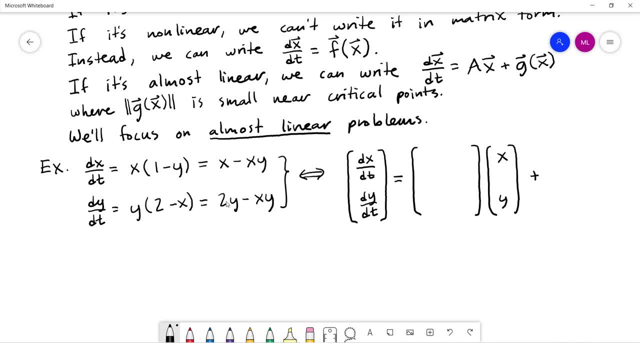 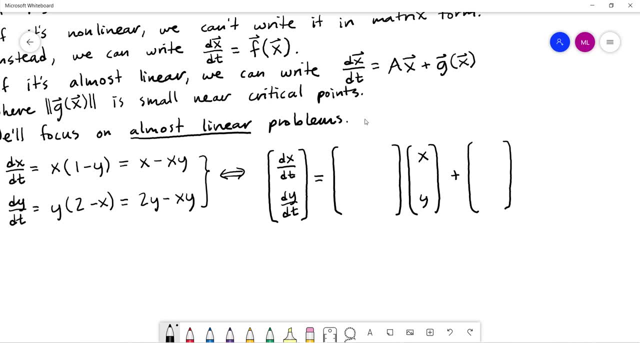 plus some other term. that's the non-linear part. so let's see 84.9. 7.ountיyyx lighting anyone anywhere? observe, this is what we need would be our min dx of this form. that's standing in the middle over here. but check this out a little quickly. your way to fill in the blanks. so all i've done is generically write it in this form right here. so my dx dt vector is this: a is waiting to be filled in my x vectors right here and this is my vector that is a function of, again, the terms in the vector x. so this is my g term over here. if we look at it, those non-linear terms are both negative xy. so i'm just 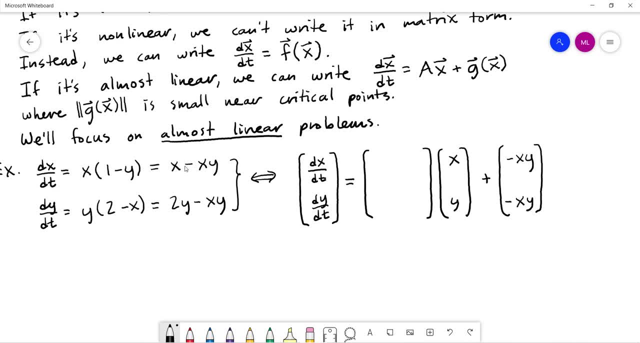 going to write that in, and here's the negative xy. here's the negative xy. i've accounted for series six, so x times y minusangles, so i'm just going to write that in. here's the for this portion of the equation, and now I need to account for this portion which we said was. 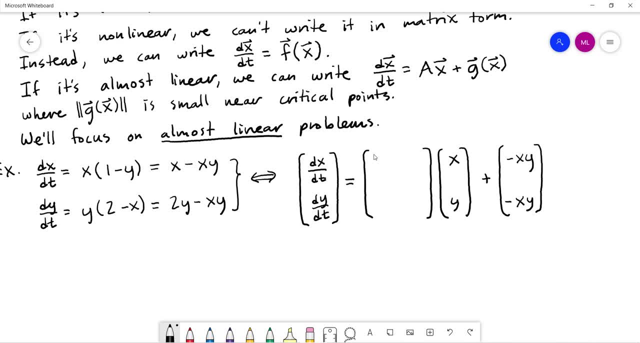 linear, So I want to. when I do this matrix multiplication on top, I want to get dx dt equals 1 times x, 0 y's. there's no y's by themselves up here, so 1 times x plus 0 y's. 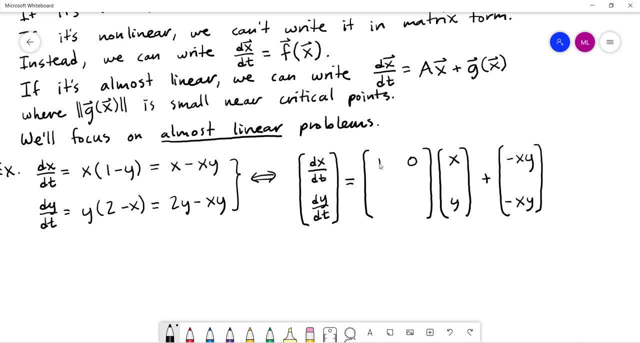 so that means I need a 1 here and a 0 here and now. my multiplication would be 1x plus 0, y plus negative x, y, and I would get all the terms that we've got. We have our plus x. 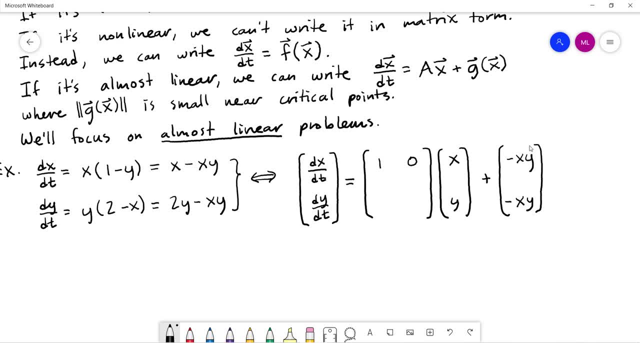 there's no y's and we have our negative x- y showing up here. So just to be totally clear, right? this term is what gives us this when it hits this and this term over here is this term over here and you'll notice that basically there is- you could think of plus 0 y showing up there. 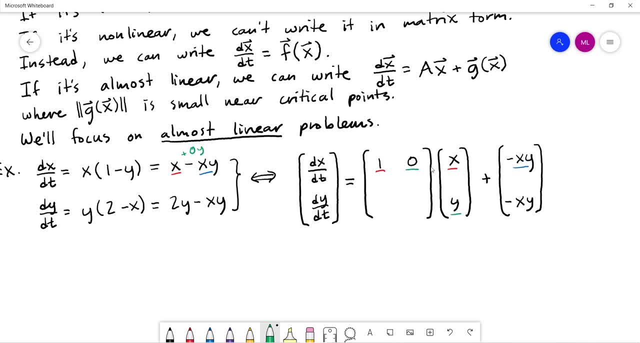 there is no 0, there is no y, and that's the result of this. Okay, for the bottom one, it's very similar. I need to have 2 y's but no x's. so that means I need 0 x's, but I do need 2 y's. and now this multiplication: the 0 will hit the x, the 2 will. 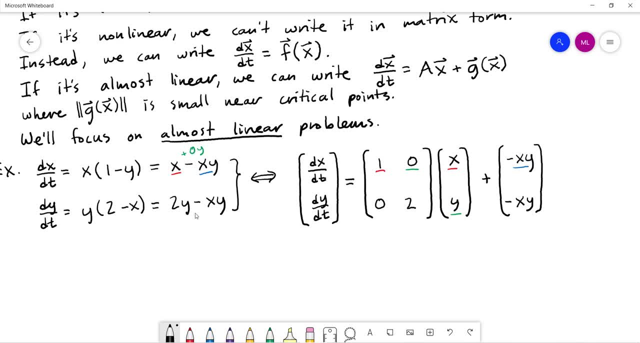 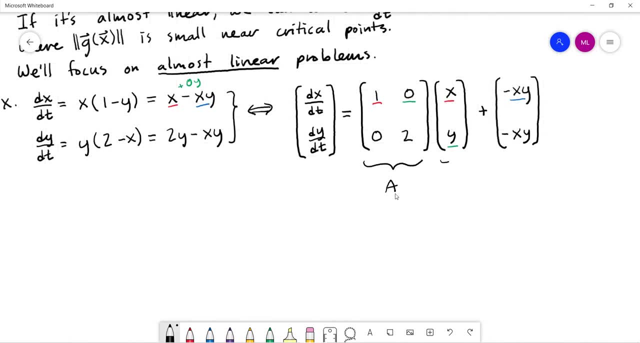 hit the y and then we'll subtract x, y and I will get exactly what we have written right here. So this is the setup. This is my a, this is my x vector, this is my vector g. that is a function. 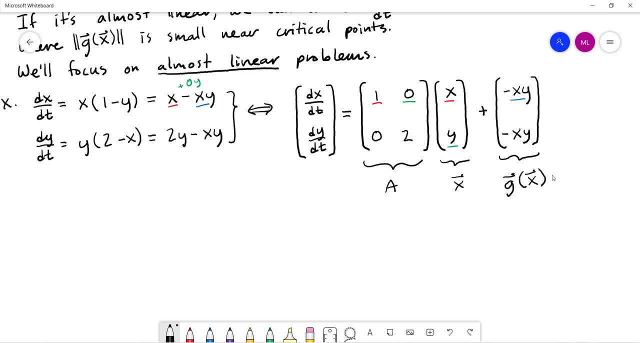 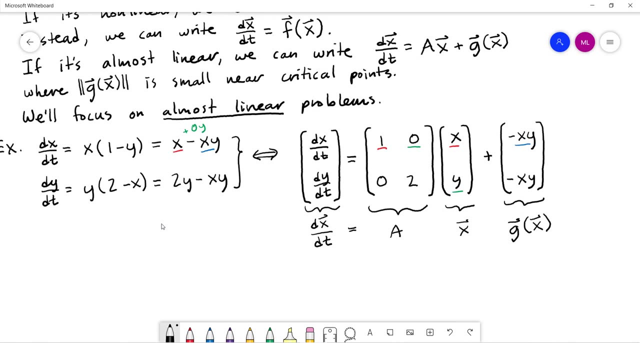 of the terms that show up in our vector x, And on this side this is our dx, vector dt. So that is all of these terms. We've written it in this form, So this is an example of what we're talking about. All we need for this to be almost linear is for these terms to be small, near a. 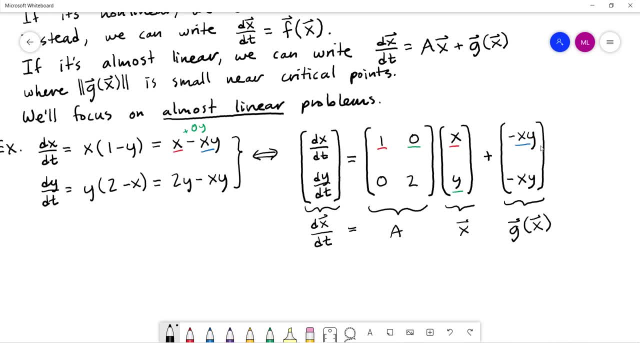 critical point And in this case, an obvious critical point is going to be the origin. And, sure enough, near the origin these terms get very small, very quickly. Okay, so we just need to find if there's any other critical points. So the first thing we should do 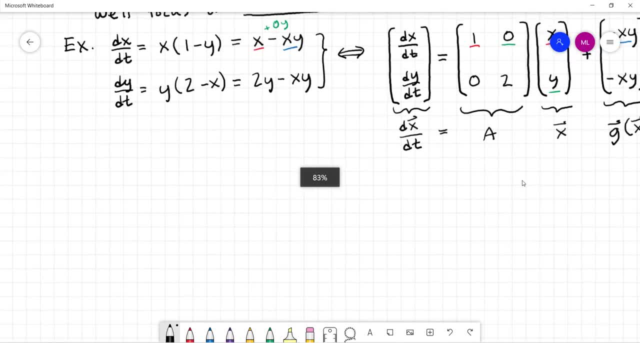 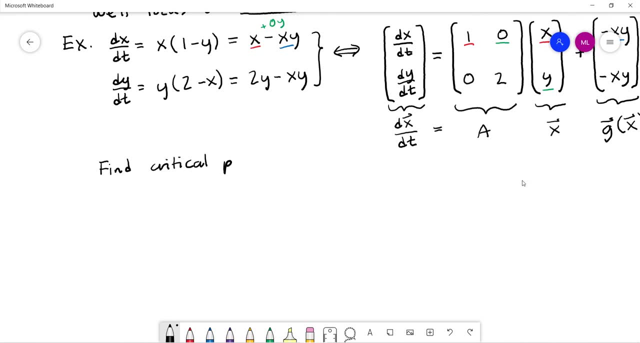 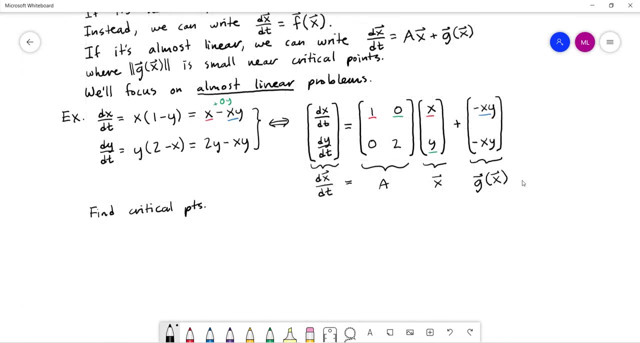 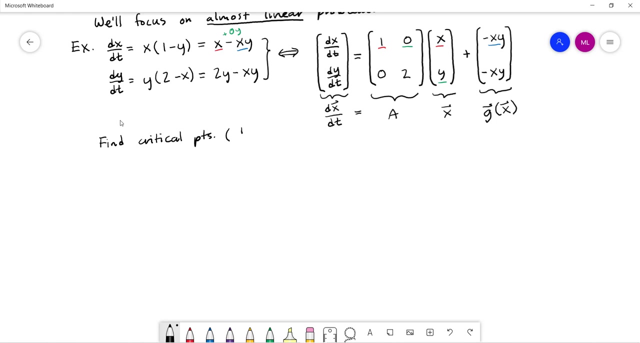 is figure out where the critical points are. So find the critical points. Okay, I just mentioned 0,. 0 is going to be a critical point, But all I'm looking for is again meaning. so when I say critical points, we want dx, dt, that vector, to be equal to 0, or, in this case, 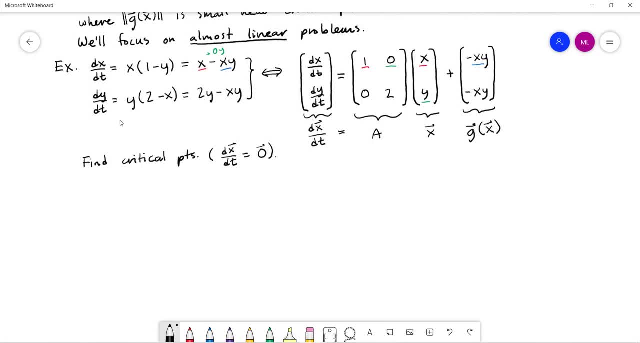 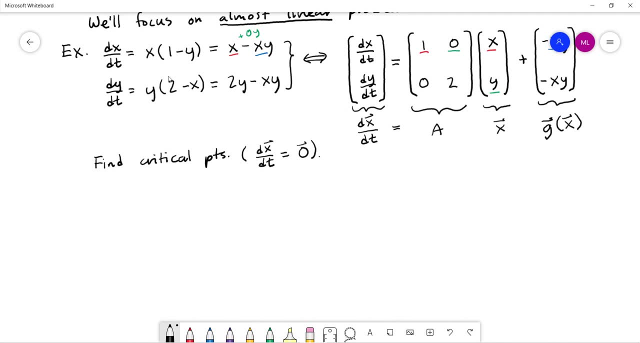 the 0 vector. So basically, I need to solve this equation up here and force it to look like 0.. So where are these critical points? Well, if I want both of these terms to be 0, right. what we're saying is: 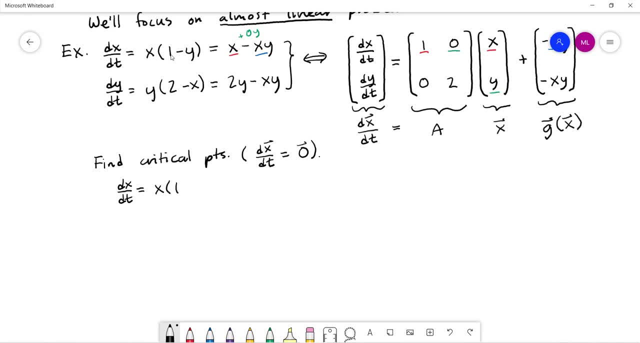 we want dx dt which happens to be x times 1 minus y. we want that to be 0.. But we also want the dy dt which is y times 2 minus x. we want that to be 0 as well, And it's easier to use the factored version. 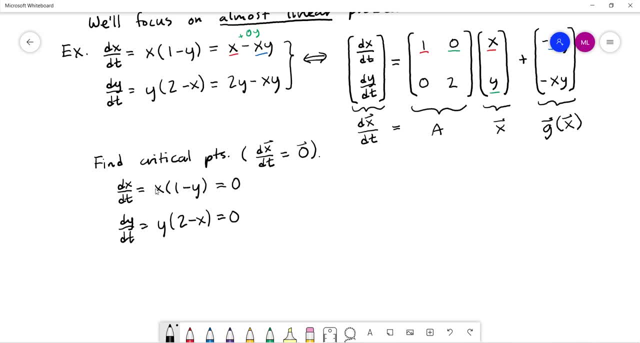 here, as opposed to the one where we've distributed through, Because now we can use the fact that if you have a product of two terms equal to 0, then either of those two terms can be 0 to make that happen. So this first. 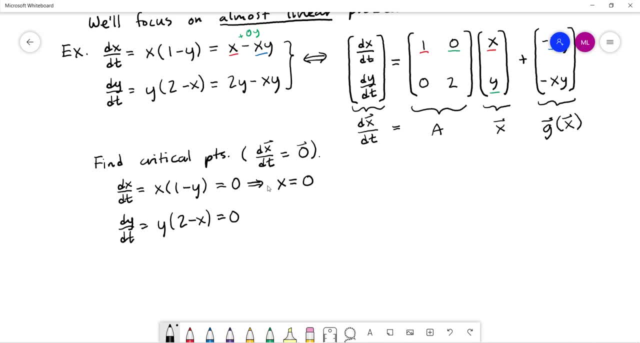 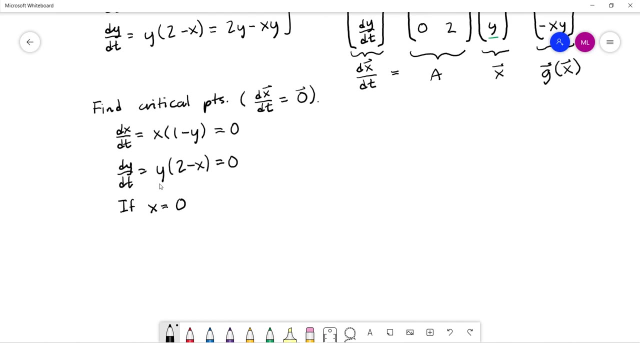 one implies we have one case if x is equal to 0. So there's a couple of possibilities. Let's write them out like this: this might be an easier way to see it. So let's do if x equals 0. So if x is equal to 0, that automatically makes dx dt be equal to 0. 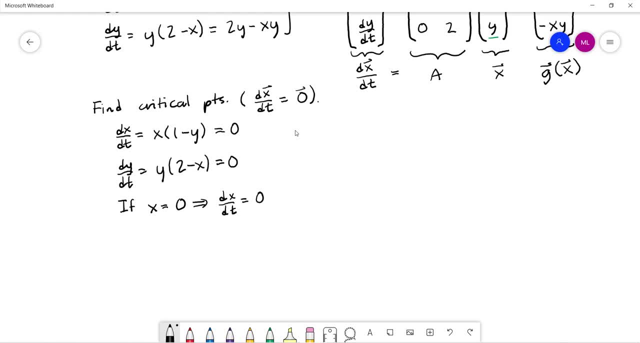 So we've got that term satisfied. dx dt is 0, as we wanted it to be, by making this term 0.. If x is 0, then that means down here: dy dt equals y times 2 minus 0.. All right, so I've just plugged. 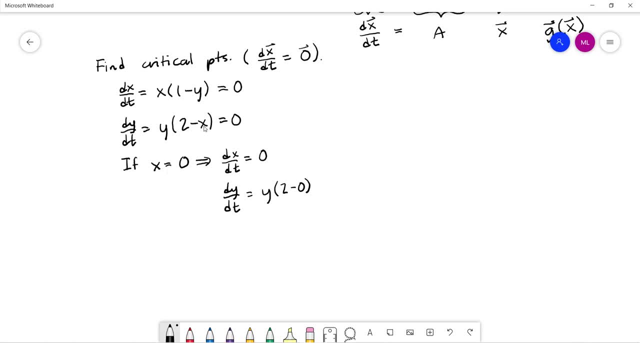 in. we said if x was 0, well, that means I need to plug in 0 for x here, And what I'm left with is y times 2 minus 0. Here's my program. So I've got y equal to 0, y equal to 0, y equal to 0. And so on. So here's my problem. So we're going to simplify all these terms and we're going to 不ли, λ, y, if x is equal to 0, then we're just going to simplify all these terms. So we just have to. 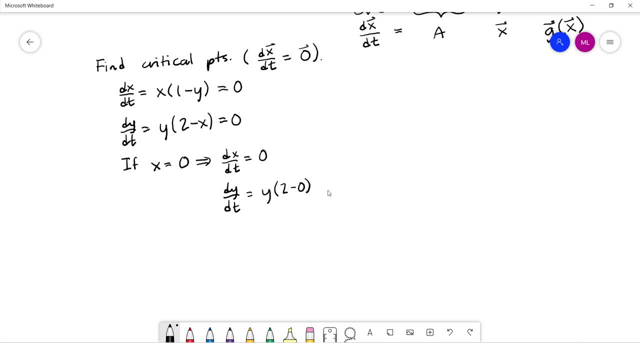 multiply our linear method following multiple parameters, including y and Kerry's, And if we multiply all the food points, my y times 2 minus 0. How do I force that to be 0?? Well, the only way to make that 0, so that's. 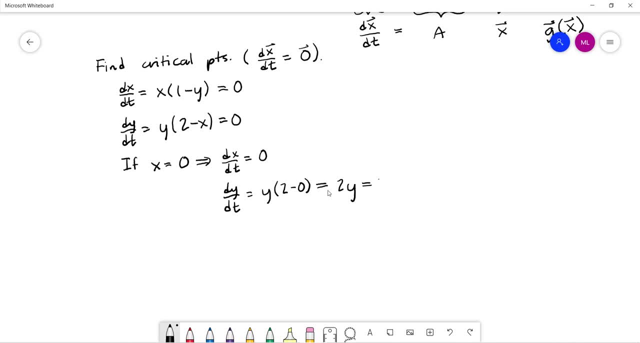 equal to sorry, equal to 2y. that has to be 0, which implies that y must also be 0.. So this gives me my first critical point, which I mentioned a minute ago, is the origin, the point 0, 0.. There's. 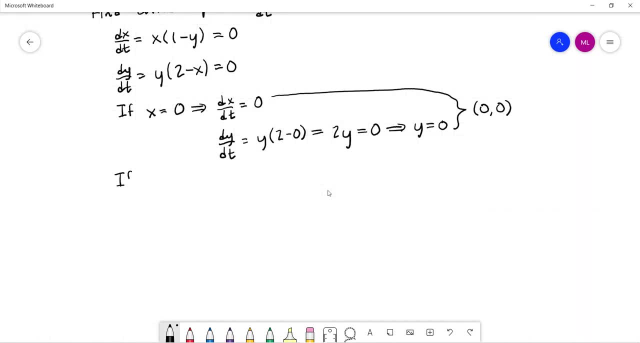 one critical point, But that's not the only way to find a critical point. I can get this whole thing to be equal to 0 not only by setting x equal to 0, but also by setting 1 minus y to be equal to 0.. 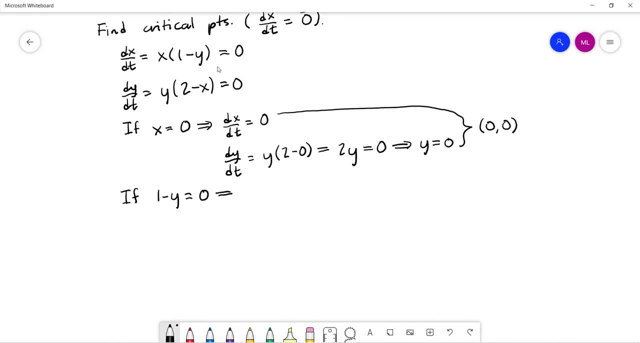 So let's set 1 minus y to be equal to 0, which would imply that y needs to be equal to 1.. And that would give us what we're looking for. It gives us that dx- dt equals 0. So we've satisfied, the top equation being 0, by forcing y to be equal 1.. That kills off this term. 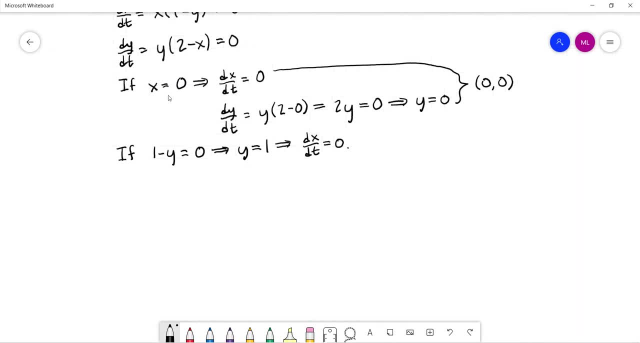 But if y is 1, then our bottom equation looks like: so what do we have down here? We've got that dy, dt is equal to y was equal to 1,, so 1 times 2 minus x, And we want that to be equal to 0. 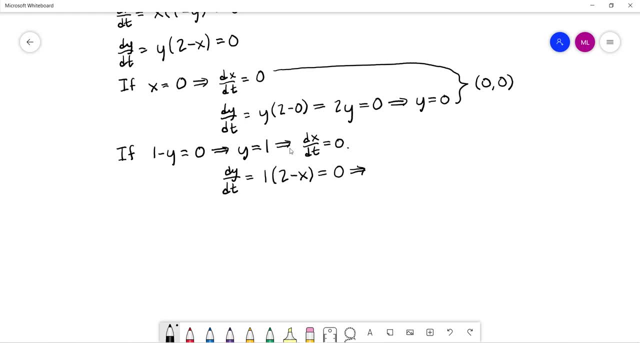 So if we're forcing that to be equal to 0,, it implies that 2 minus x is equal to 0, which implies that x has to be equal to 2.. And so this gives us our second set of information, right. So we had 0, x equals 0, y equals 0,. 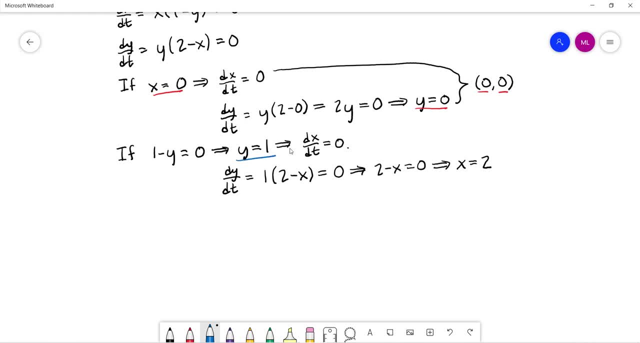 gave us those two, And now down here we've got y equals 1,, x equals 2, giving us a second critical point. So grouping those two together, we have the point 2, 1 is also a critical point. 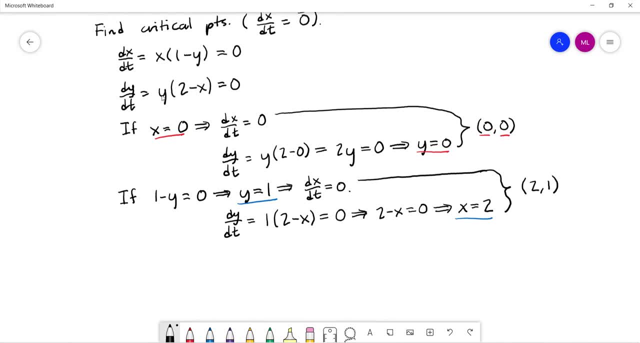 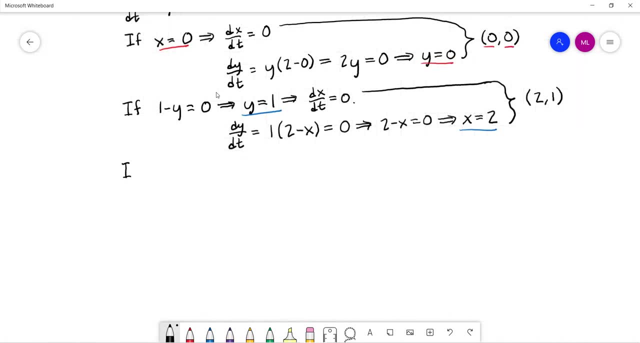 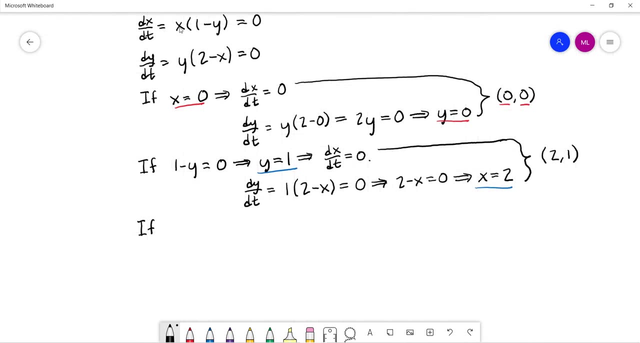 We could go through and try to do the same thing, starting off by setting y equals 1,, y equals 0, and setting x equals 2, and working our way backwards. So basically, to be completest about this, we would want to basically do: oh, So we've done the two cases where I forced. 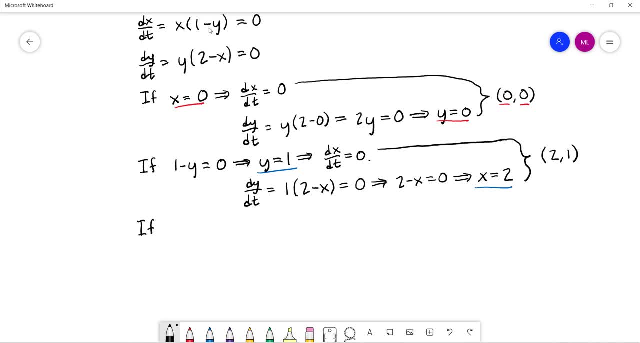 this to be 0 and see what happens, or forced this to be 0 and see what happens. Now I'm suggesting to make sure that we haven't missed any critical points. we also need to set this equal to 0 and see what happens, and this equals 0 to see what happens. So if y equals 0, that implies 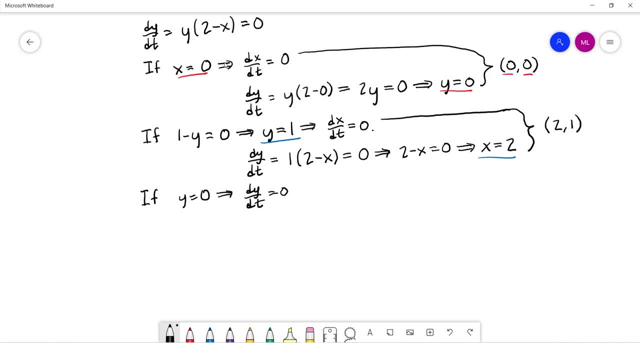 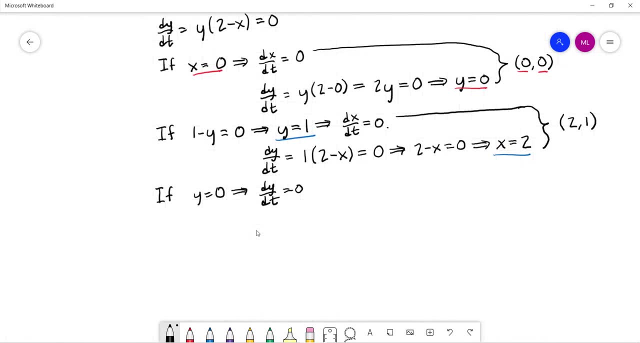 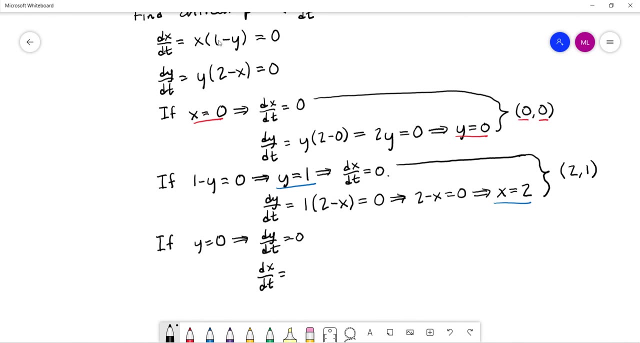 that the dy dt automatically will be equal to 0. on the bottom right, This bottom term will go to 0. And but if y equals 0, then on top dx dt will be. so if y is 0 on the top, I'm just left with x. 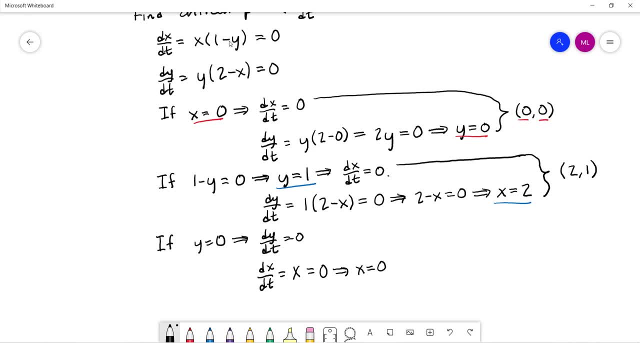 We want that to be equal 0, so that implies that x is equal to 0. And we get a repeated critical point that we'd already found: x equals 0, y equals 0. The origin: So we already found that one. It gives us a redundant piece of information. 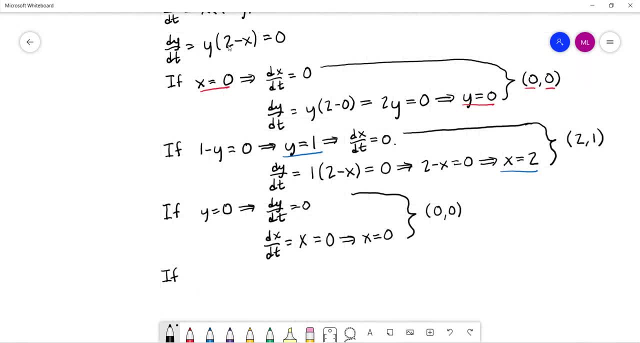 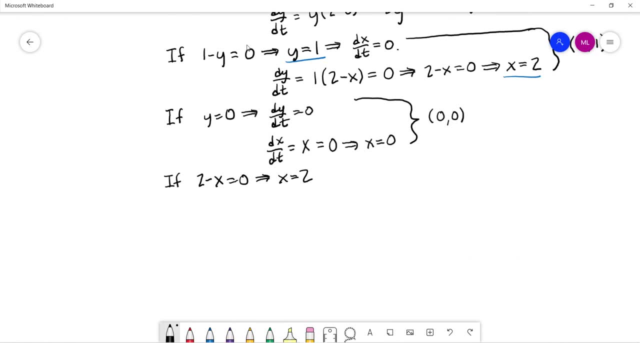 And, lastly, we would do the final case check to see that 2 minus x is equal to 0. So if 2 minus x equals 0, which implies x equals 2, which will give us that our dy dt equals 0, that's good. 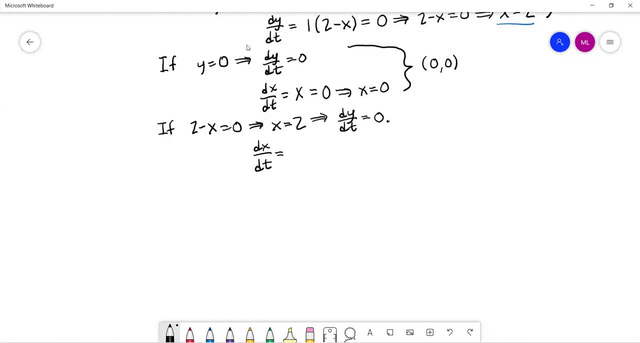 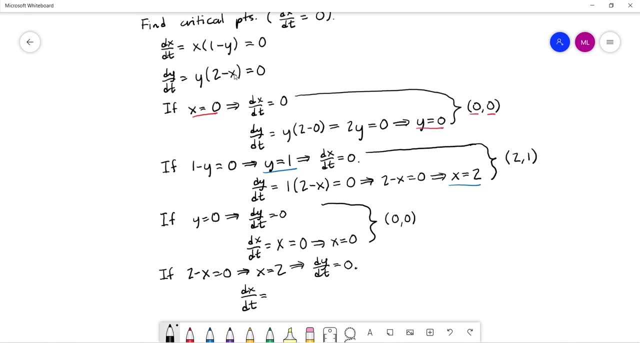 But what does it mean for dx dt? Well, dx dt would be equal to going back up, just copying this down. So again, I've basically forced x to be 2, which makes dy dt be equal to 0. What does that mean? happens up here. So if x is equal to 2,. 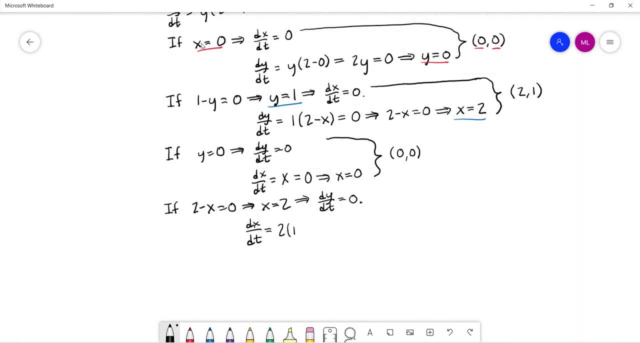 then we've got the top being 2 times 1 minus y, and that's supposed to be equal to 0. And that would wind up giving us that y is equal to 1.. And putting these together it would give us the point which, again, we've already found. So these two additional. 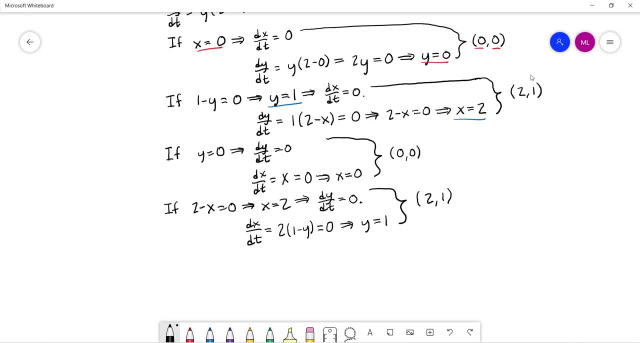 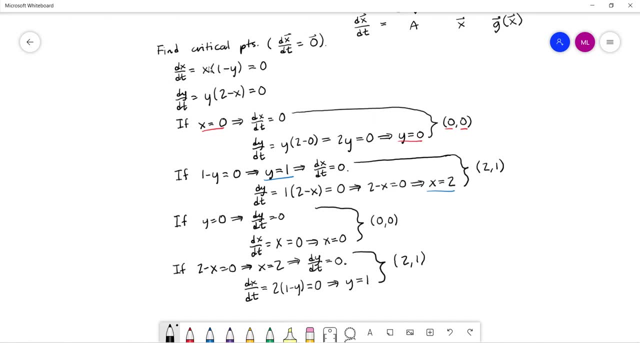 tracks that we looked at turned out to be redundant. They gave us critical points that we'd already found from other methods. But to be safe in general, you should check all four of these things if you've got basically a product set up the way that we've got here. 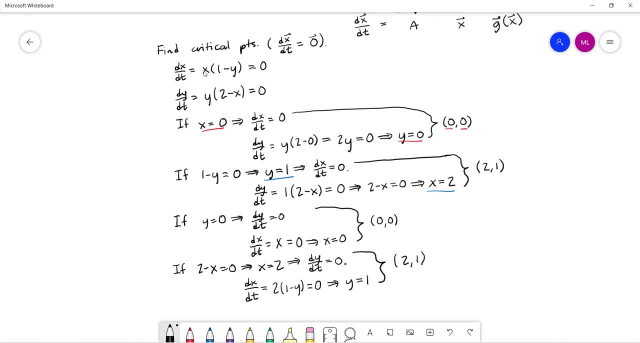 This times this, This times this, Force this one to be 0, and see what comes from that. Force this to be 0,. see what comes from that. Force this to be 0,. see what comes from that. And force this to be 0, and see what comes from that. And so there's our. 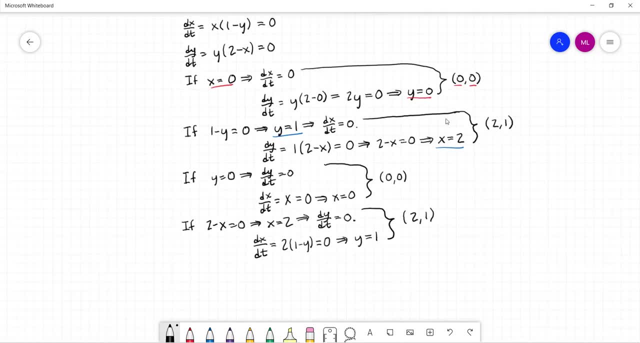 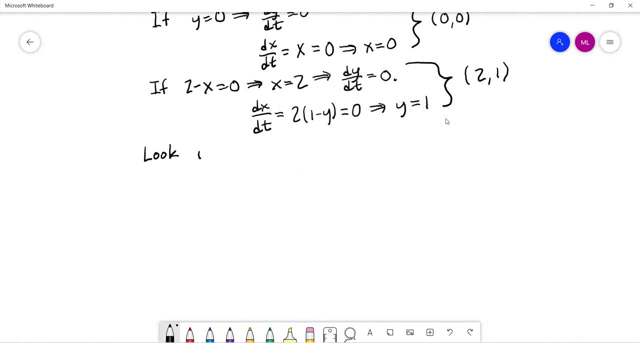 four cases. that led to two different critical points in this case. So we've got two critical points. Let's start by looking near the point. Let's see what happens at the point. So basically, we want to be close to this point, The easiest way to talk about what we mean. 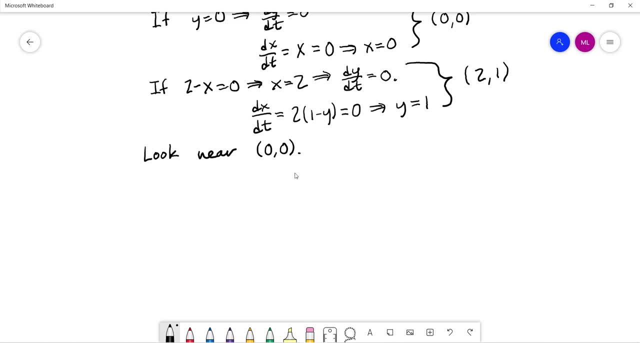 when we say close is think of it as sort of we want to be like in a range, We want to be in a radius, a small radius from this point- So let me put that into parentheses here- Think within some small radius, And for now we'll just call that radius r. 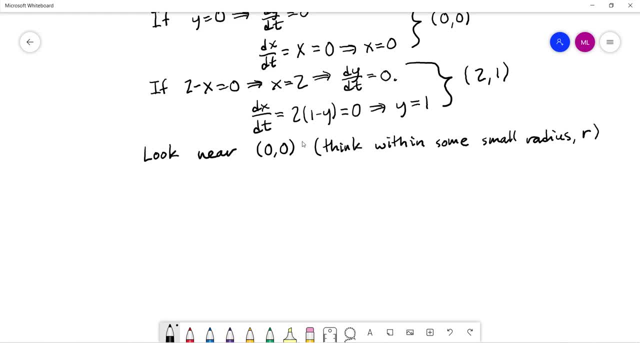 We'll see what happens, Okay. So basically, if we're doing this, I'm thinking about a r from this point. That should kind of remind us of polar coordinates if we're suddenly dealing with radius here. So we don't have to do this all the time, but I want to think about what's. 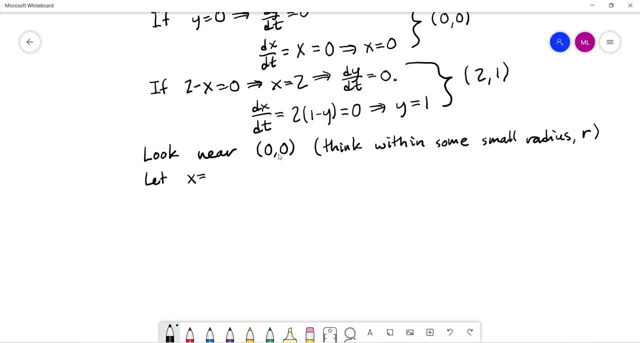 going on here. So I want to rewrite our equations in polar coordinates, just to think about what it's going to look like, So you may recall- hopefully you'll recall- that in polar coordinates x is equal to r cosine of theta, and y is equal to r sine of theta, And so I'm just wanting. 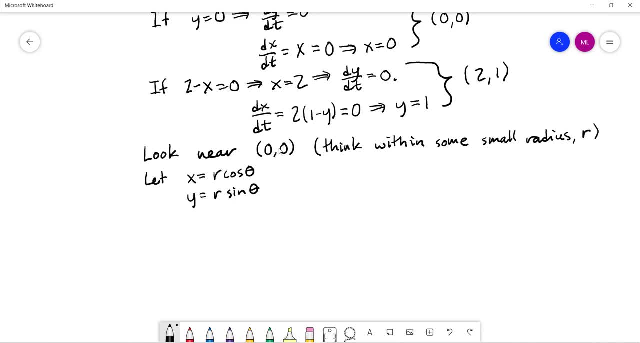 to pick all the points x, y, centered at zero, right, Here's how they're given: centered at zero, where this r is some small value, And so, if we can find a point, we just are looking for r to be small, letting r approach zero essentially. So let's let those be the way. 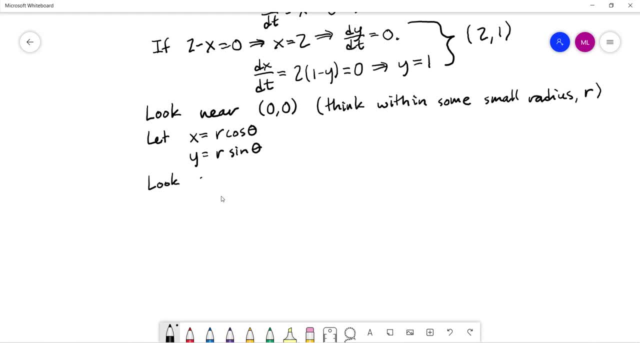 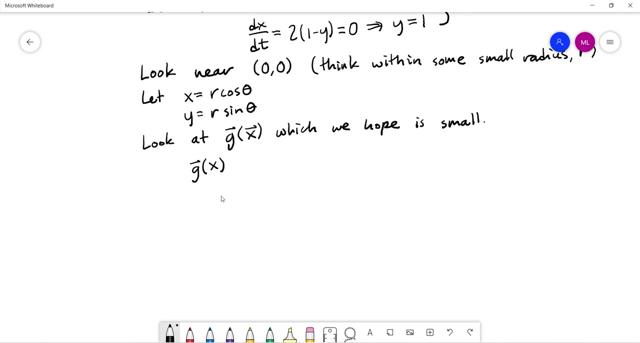 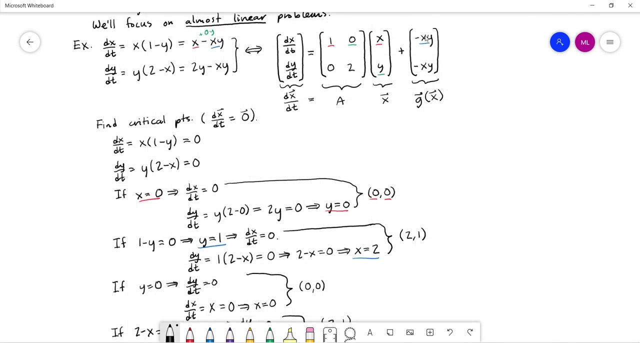 that we define our x and y. And now let's look at that term, g of x, that we're hoping is small, And let's see if indeed it is small. So basically, our g of x term looks like coming back up here. you'll recall, g of x looked like this, right? So basically, 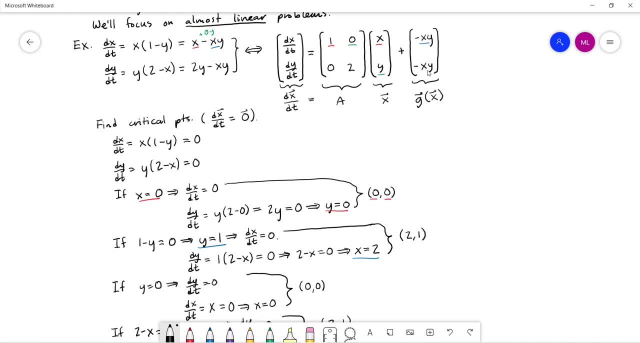 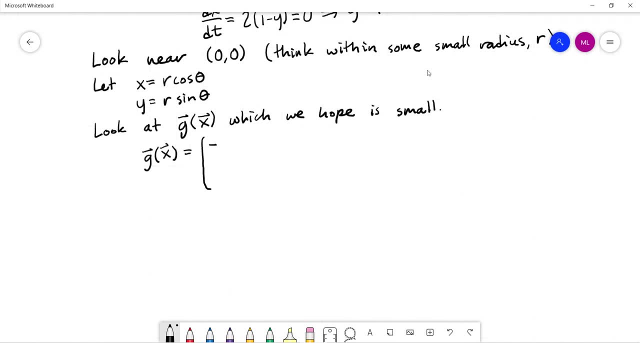 the terms that show up are negative x y and negative x y, So in both cases it's going to be two different terms. So we're going to look at the terms that show up and we're going to look at two different terms. On top we have negative x y, which means when I multiply my x and y, 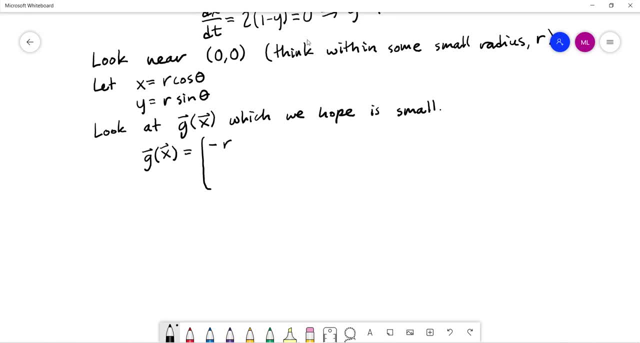 I'm going to multiply the polar coordinate versions. I'm going to get negative r squared sine theta, cosine theta, And again the top and bottom are the exact same thing. So we just get two of those, one on top, one on bottom. So there's what our g of x looks like. 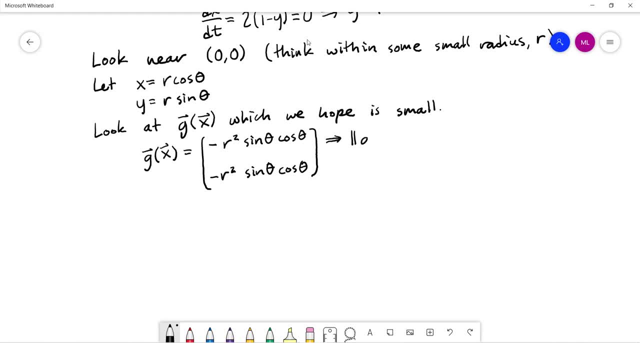 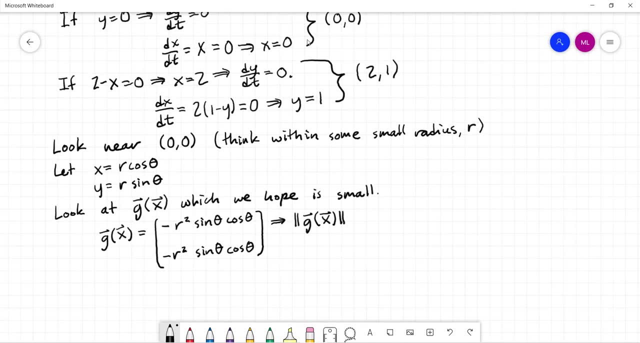 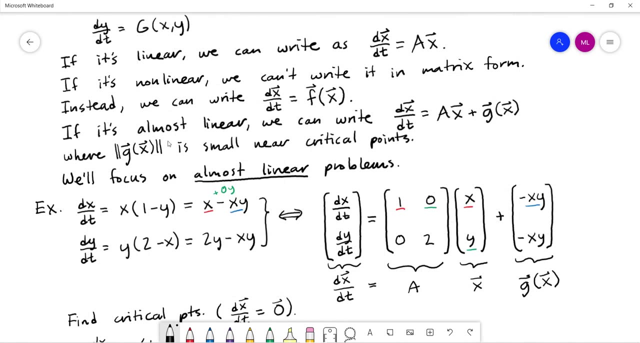 I want to figure out what is the magnitude of that thing, because that is what we were hoping would be small. Look at g of x, which we hope is small. But remember that what we're actually interested in is finding the magnitude to be small. So how do we find the magnitude? Well, 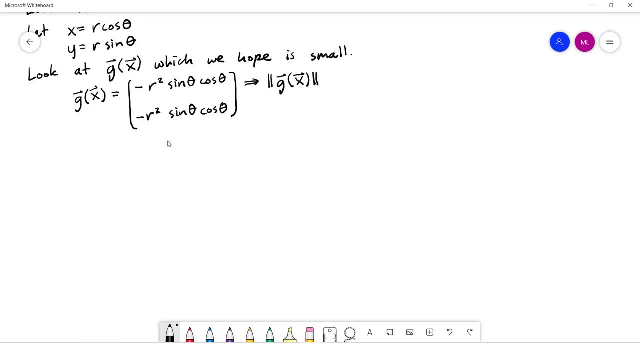 we find the magnitude basically using the same way that we always find the magnitude Basically on any vector. hopefully this is something that you'll recall. if I want the magnitude of some vector v, where v is equal to the vector- maybe one, two or something like that- all you need to do is take the square. 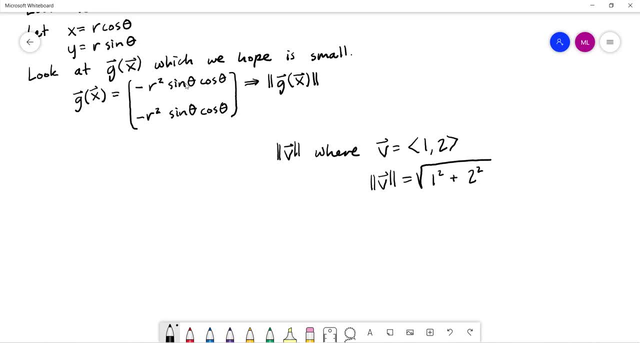 root of the sum of the squares of the components, and in this case you get what root five. so this is what we need to do. you've probably done it for numbers. we're now doing it to this vector here, so let me erase this, but that's all I'm about to do is take the square root of the sum of the squares. 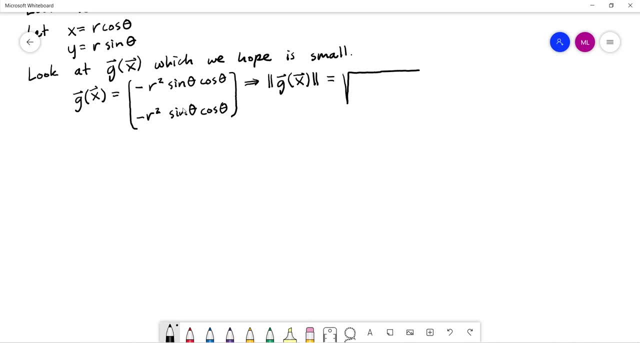 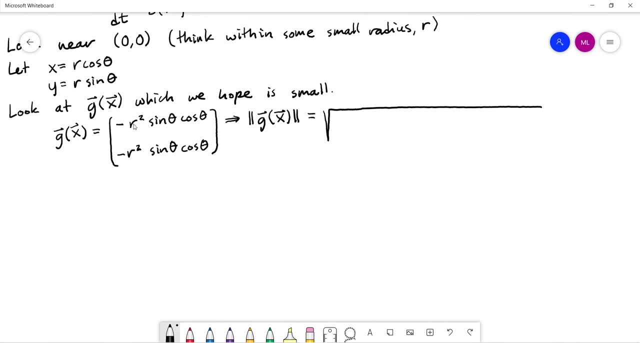 so the magnitude is going to be the square root of the sum of the squares of this thing. so I need to square this term and square this term and add them together. I'm just going to put a two in front because I know I'm going to get two of them once I add them together. I'm going to get this one plus. 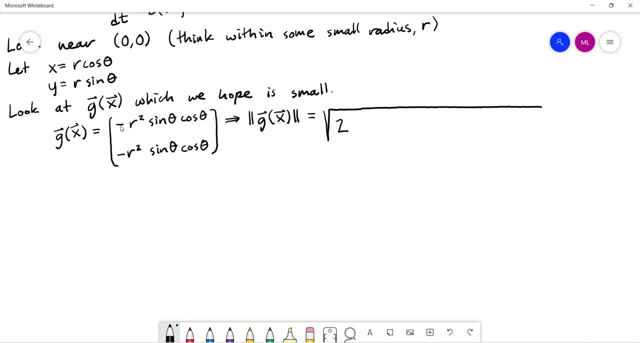 this one, so let me just write it once to save a little space. I also know when I square things, these minus signs are going to disappear, so it's going to be positive, and when I square this I'm going to get r to the fourth um. so 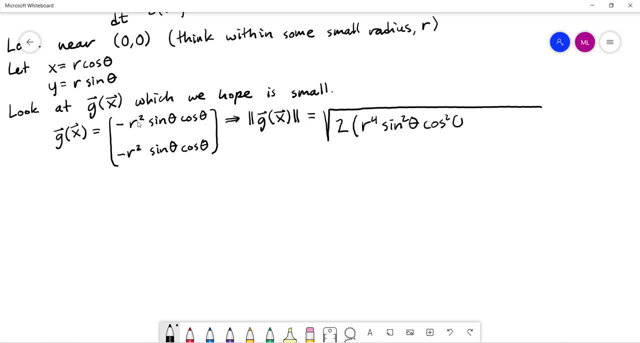 and again. basically, I would have gotten two of these, one plus another, so I've just shortened that, preempted that by writing that I have two of them. explicitly change one plus one to a two. okay, uh, so this is basically what we've got in this particular case. um, it's looking a little. 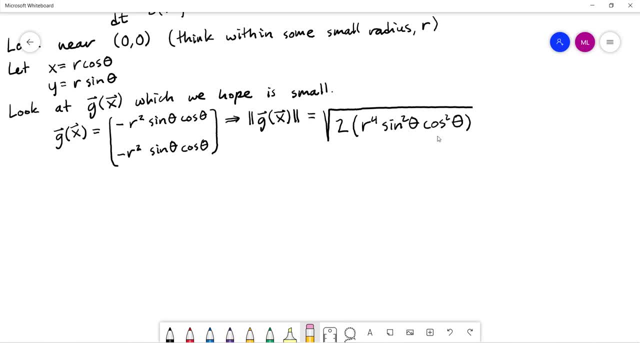 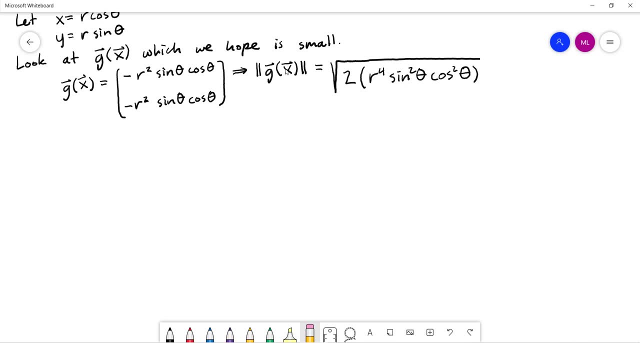 bit ugly, but we're okay with that. I also want to think about now, just thinking about the vector x itself. so let's we're looking at g of x and its magnitude. let's think about x itself and its magnitude. so now I want to look at x itself, just the x vector. what you'll recall is simply: 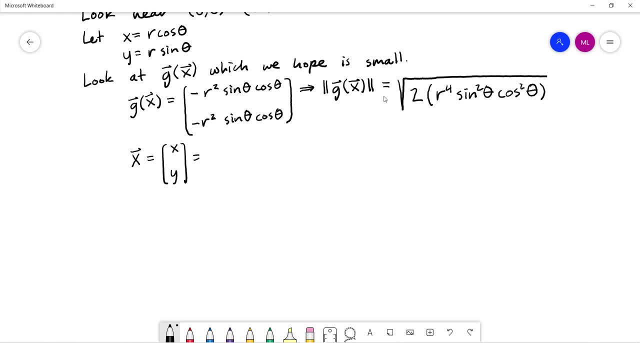 right x, y, so for us that's r cosine theta, r sine theta parameter. if you get that right and then simply write the general equation for x, so this is q times one minus x, z minus y minus y and the, you get the other five and you get this x star. 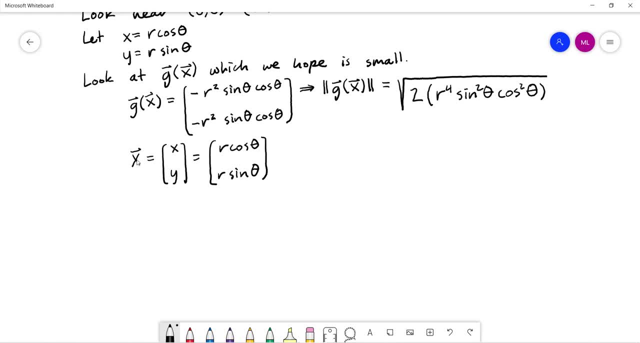 equal to minus x помощью. we're going to test our and finally in this approach, this: how many Electron? two processors, square root of theta plus an r? squared, sine squared of theta, and you'll notice I can factor out the r? squared and I'll have r? squared times, basically a cosine squared of theta plus a sine. 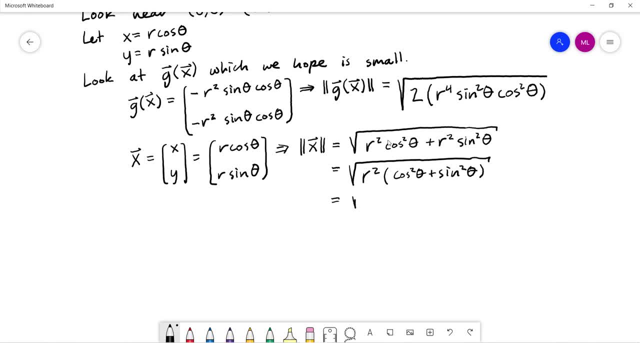 squared of theta, which is simply one, and we just have the square root of r squared, which winds up just being r. So the magnitude of our x vector is just r, and I'm interested in what happens to g of x when this magnitude of x gets small, So basically when r gets small in this case. So we just want to. 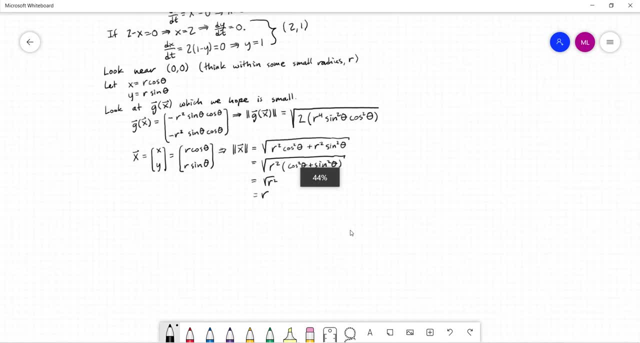 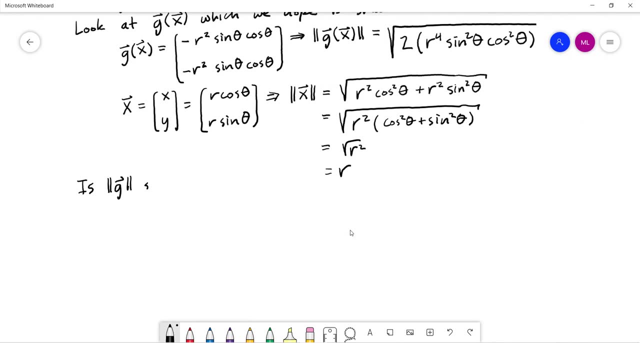 know. oops, let's come back here. so is the magnitude of our g vector small when the magnitude of the x vector is small? That is poorly placed. Let me see if I can move this so it doesn't have to be quite as tilty. There we go, Okay, Yeah, good. 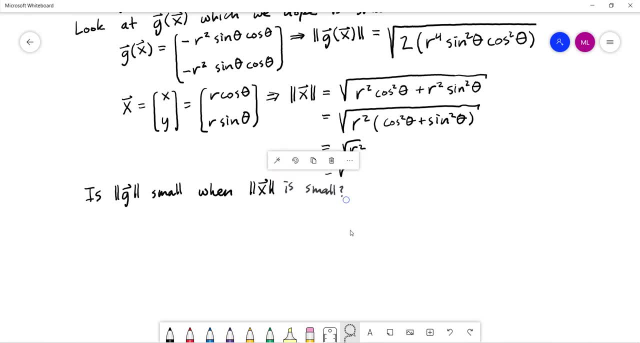 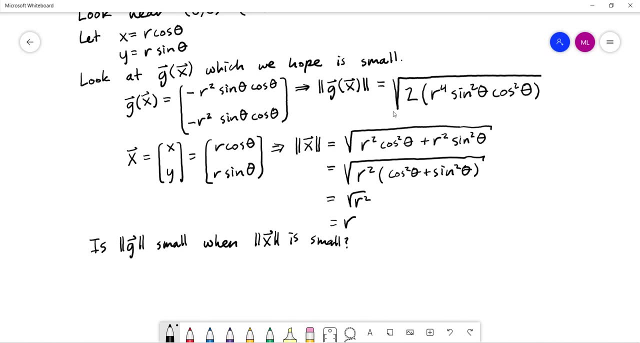 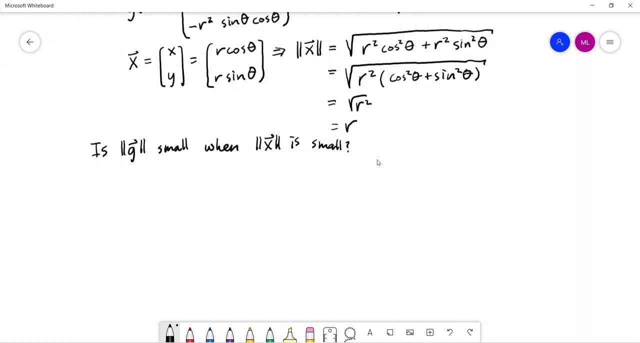 enough. Okay. So basically, right, we're trying to figure out if this is small near the critical point. Near the critical point is when we're near the origin. Near the origin is basically when this magnitude, which simplifies to r, is close to zero. So, basically, we just need to let r go to zero, right? 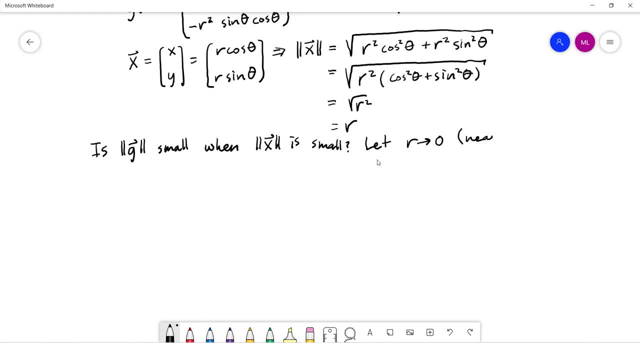 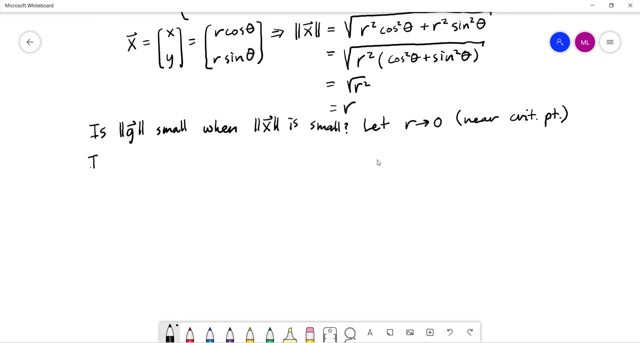 That's what it means to be near the critical point: zero, zero. So that first critical point, zero, zero, is the one that we're talking about. Okay, And so, basically, what I'm suggesting is, if you know, if we're- 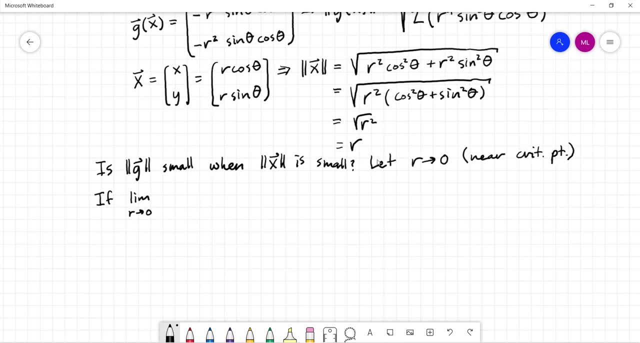 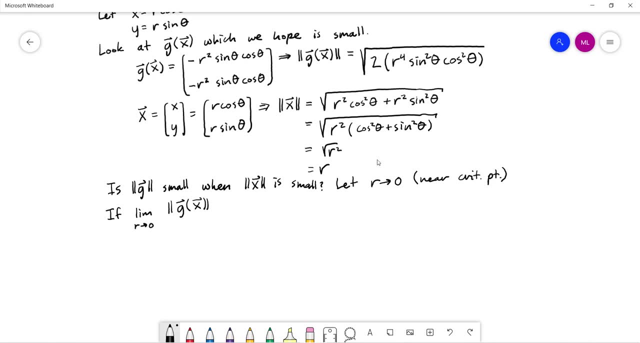 looking at the limit, as r goes to zero, of our magnitude, of our g, of x term. oops, too many little lines there. Okay, So I'm going to look at the ratio of that over x. So, basically, as we go towards, 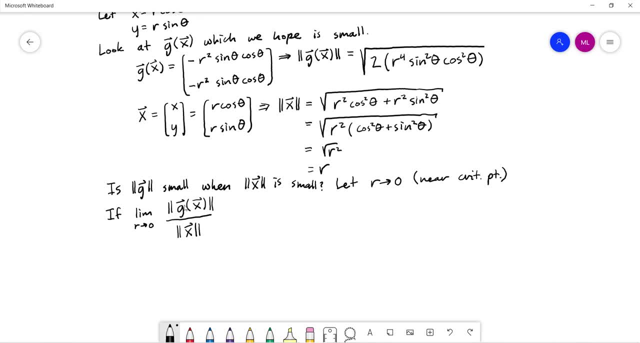 r equals zero, does this go towards r equals zero And in fact does this go towards r equals zero Even faster, so that this overall ratio is zero. So if this ratio is equal to zero, then basically what it's suggesting is: our g vector is. the magnitude of our g vector is: 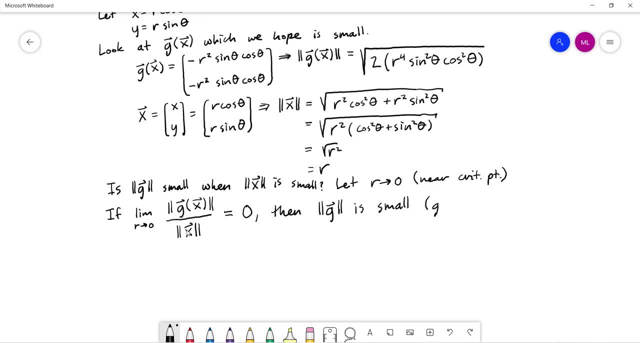 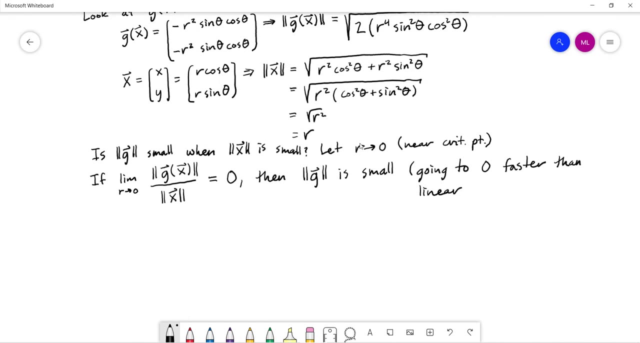 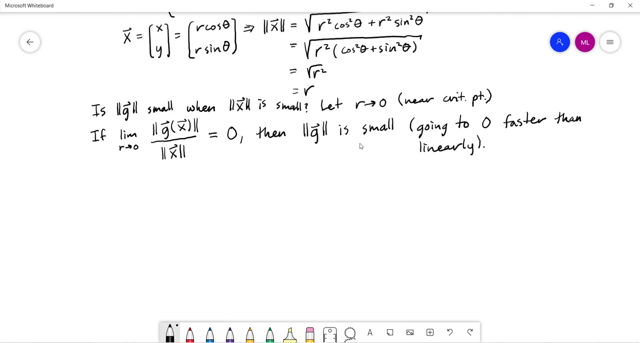 small right Going to zero, faster than essentially over here r, which is just linear, So faster than a linear, Okay, And that's all we need. Then our- let me actually clean this up a little bit- So going to zero. 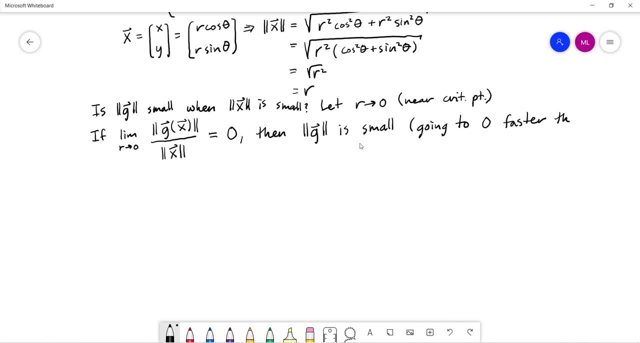 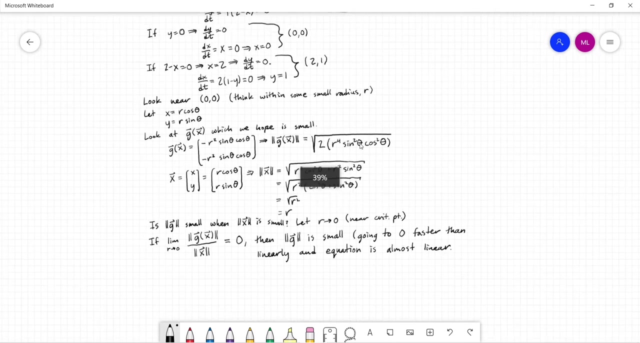 faster than linearly, faster than linearly, And the equation is almost letter, almost linear, So that's linear. Okay, so let's just step back and just take a big picture. All I'm wanting is for something to be almost linear, even though it's technically not linear, because we have these. 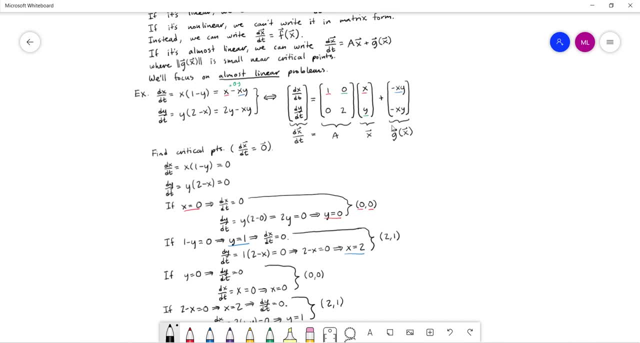 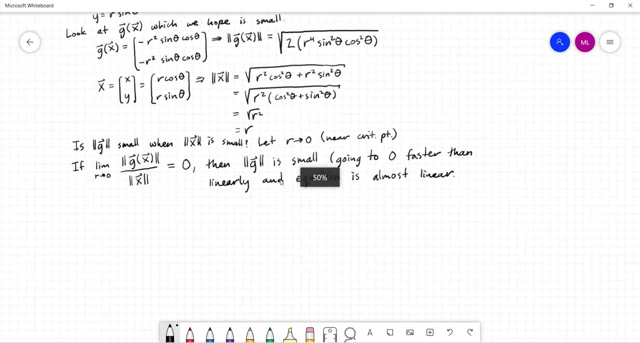 nonlinear terms. I'm hoping that near the critical points, these nonlinear terms become unimportant, that they're tiny compared to everything else. So basically, I want this to be large compared to this. These are the linear terms, And so if this term, the nonlinear term, is small, meaning that 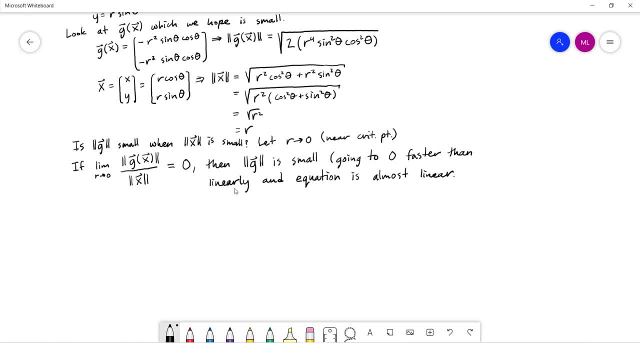 it goes to zero faster than linearly, faster than the linear terms, then the whole equation will be almost linear. So all I need is this term to go to zero faster than this term which is going to zero linearly, And that will mean, if this ratio winds up being zero, that means that this is going. 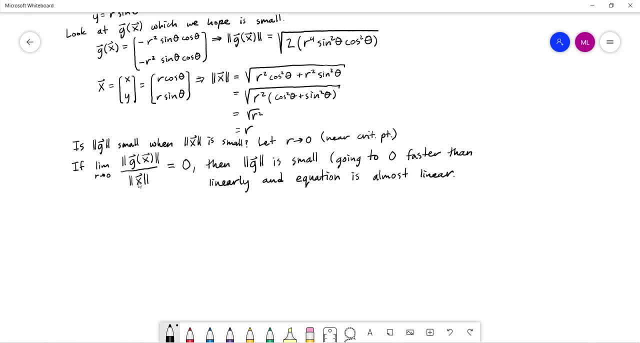 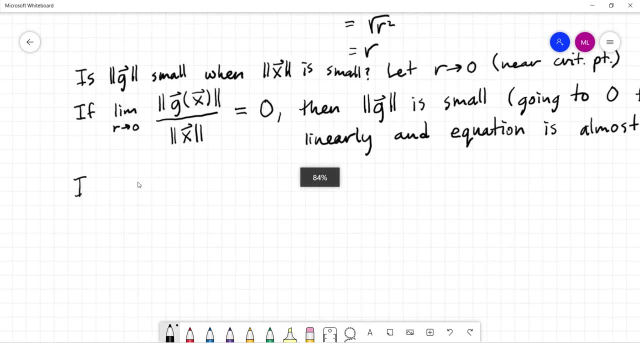 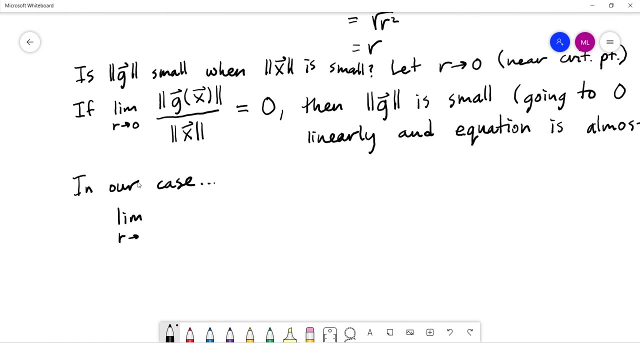 to zero much faster than this, And it's basically a much smaller term than the linear terms. So that's all we need to do. Okay, so for us let's zoom in. In our case we have the limit, as r goes to zero, of our g of x term, That magnitude. 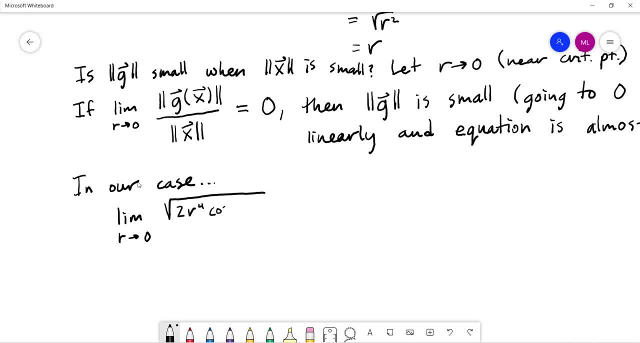 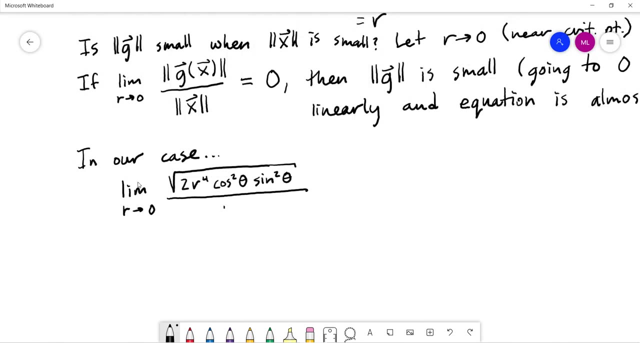 was the square root of, I think, 2r to the fourth cosine squared of theta, sine squared of theta. If I remember correctly, something like that, And on the bottom we just had r, is what we wound up with. We can kind of tell what's going to. 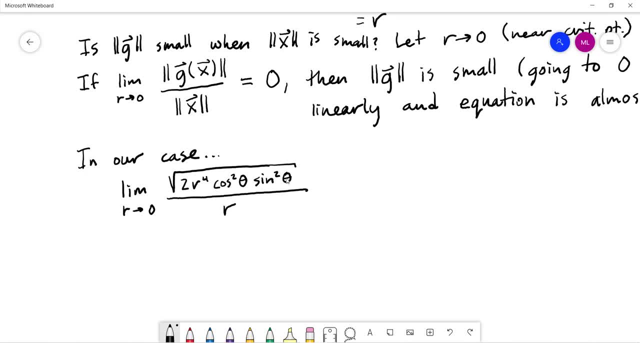 happen up here. Forget about the values of theta between sine and cosine squared right. We could do a little bit over here. One thing you can think about is that, right, the biggest that sine and or cosine is ever going to be is one. So let's just say hypothetically that both We found a magic. 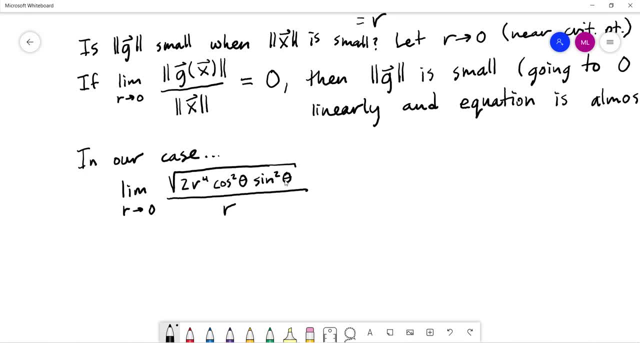 that somehow made cosine be one and sine be one doesn't exist, but just hypothetically. No matter what, one of those two is going to be smaller than one. in real life, For any theta you pick, they're going to be smaller than one. But what it suggests is that this top term is necessarily less than or. 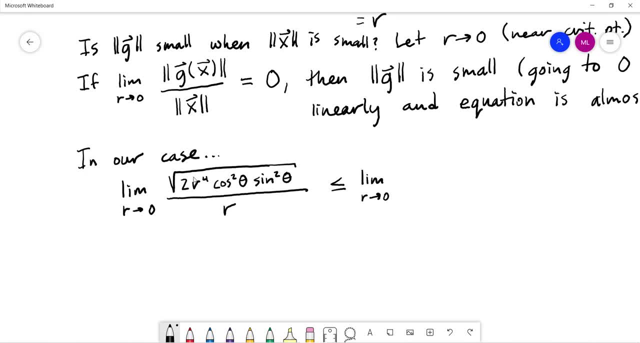 equal to the following. So the limit is: r goes to zero. on top, That's going to be smaller than the square root of 2r to the fourth, And on the bottom we still have our r. So this inequality is coming from an argument about the sine and cosine, The biggest that either of them independently could be. 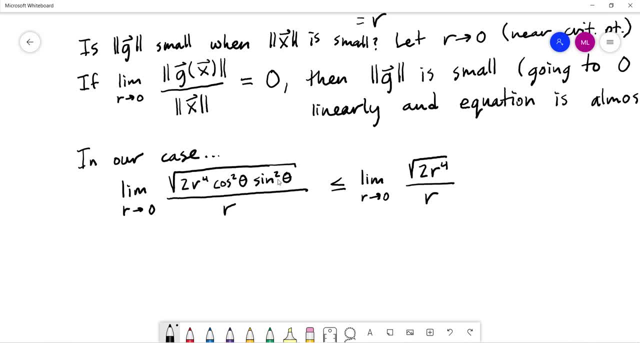 is one, and they can never be one at the same time, but just for appeasement's sake, let's say that they somehow are. At most, this term could be 2r to the fourth times these other coefficients that, as we've said, are always going to be less than one when we multiply them together. 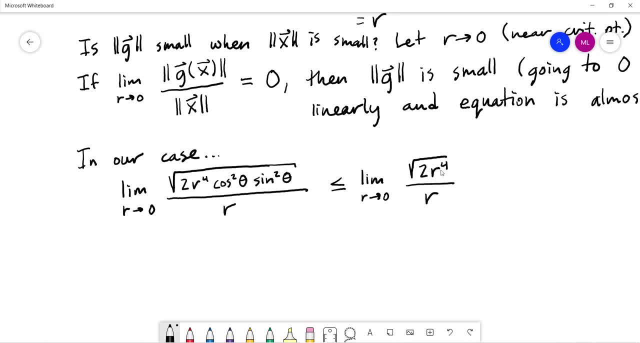 So, basically, I know that this term is less than this term, but this term itself. I'm going to simplify that We're going to have the limit. as r goes to zero, We can break that root 2 out. When I take the square root of the other term, I get r squared on top, r on the bottom. I can cancel. 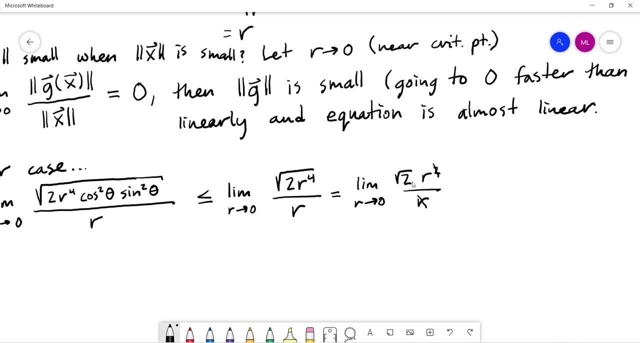 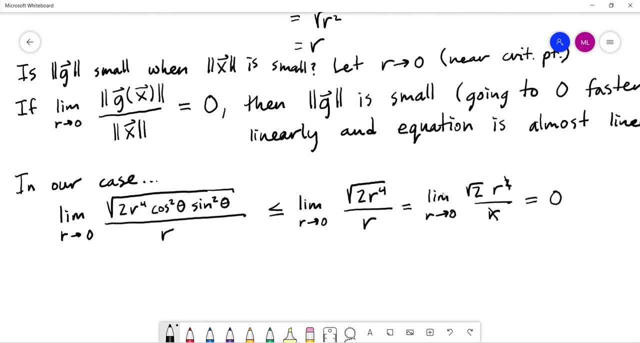 this. We just have the limit, as r goes to zero, of root 2r, which is indeed zero. So basically we can see: right, we have a higher power of r on top than on the bottom. This is going to zero, like. 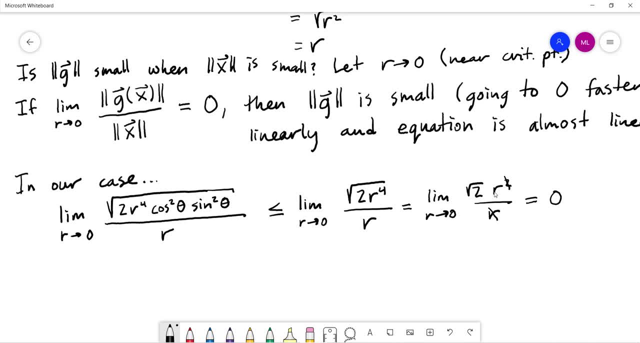 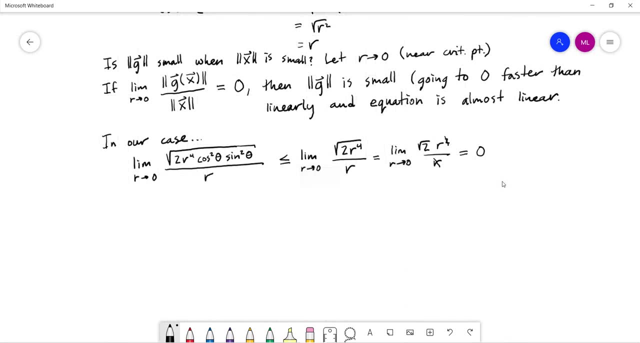 r squared On the bottom, we're going to zero, like r. Here it's going to zero quadratic, here it's going linearly and therefore the top is clearly going faster than linearly. So it's smaller than the other terms. Okay, so this tells us that r is indeed almost linear. So 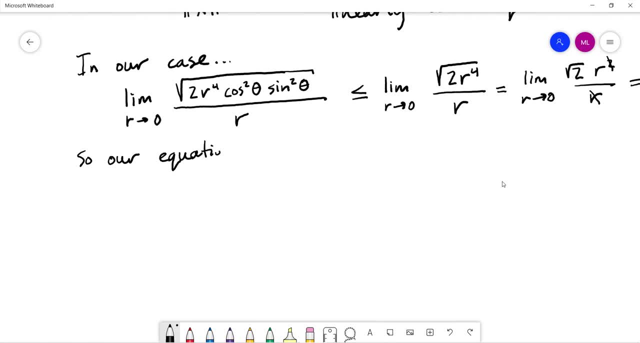 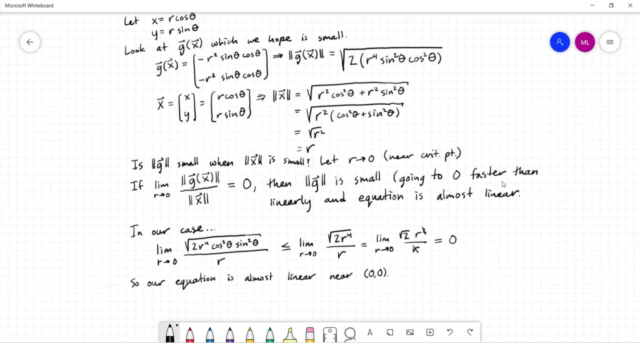 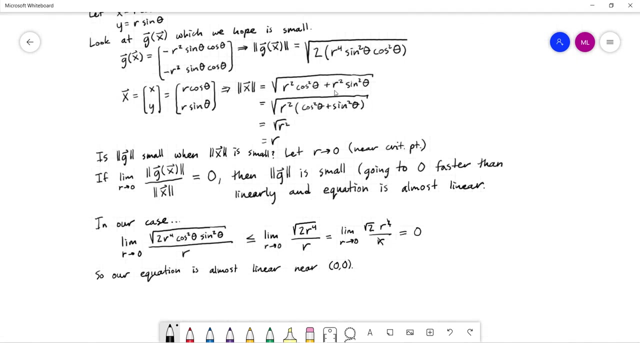 our equation is almost linear, near zero, zero. You can make the same argument. you'd have to do a change of variables to kind of re-center things around the point 2, 1, but it turns out the argument's very similar And you would basically rewrite things. 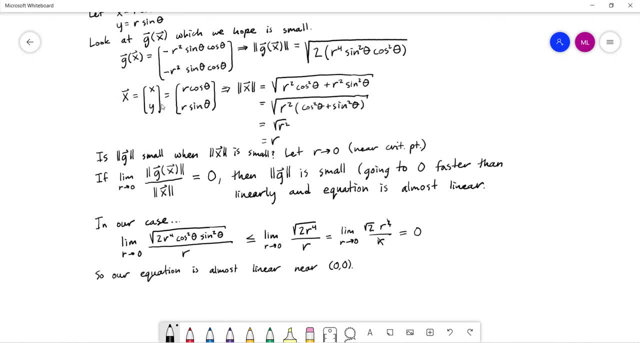 with a substitution over here to re-center things basically at that point, and you would get the exact same argument: It's going to be small there as well. This is not an argument that we in general have to go through on these problems. I just wanted to show it to you once, so you kind of get. 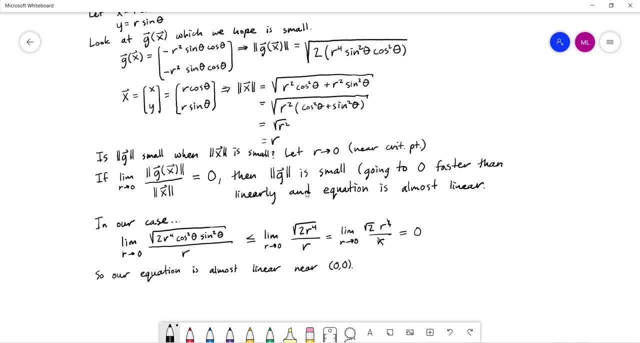 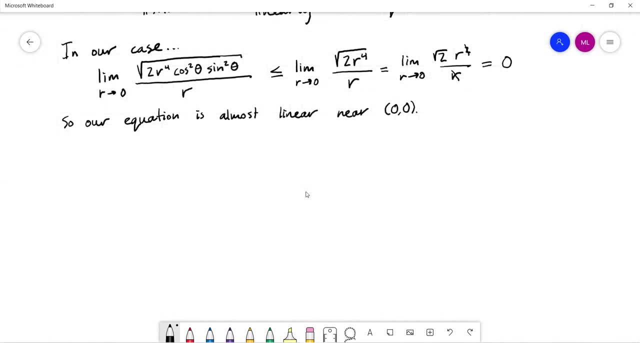 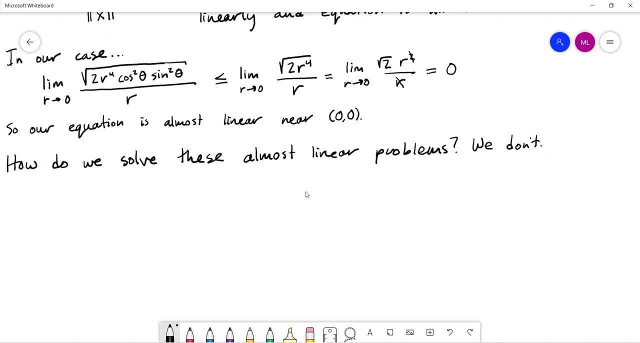 a sense of what the argument is of why these things work. Okay, so how do we solve one of these? How do we solve these almost linear problems? And the answer is basically that we don't. Instead, we do something called linearizing the problem. 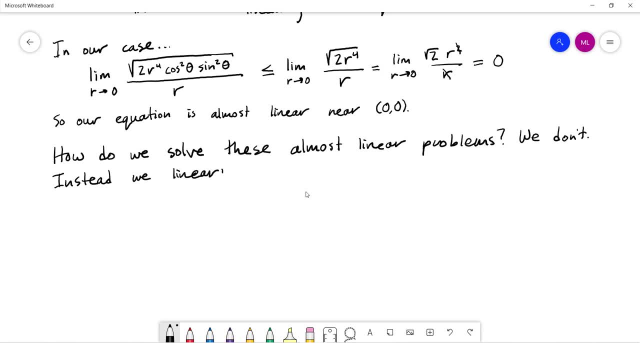 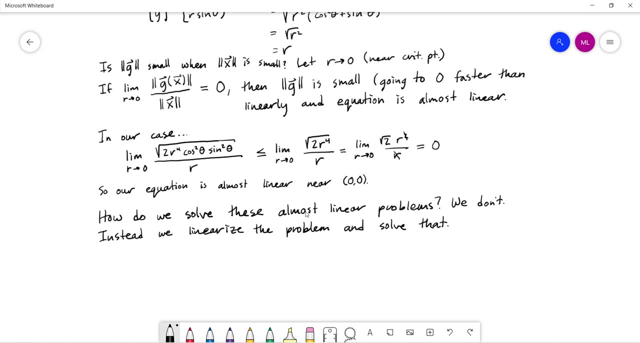 and solve that. And the idea comes from what we've been discussing. If our problem is almost linear, meaning the nonlinear term is tiny near those critical points, then near those critical points that nonlinear term is basically unimportant to the solution. So we can solve that And we can. 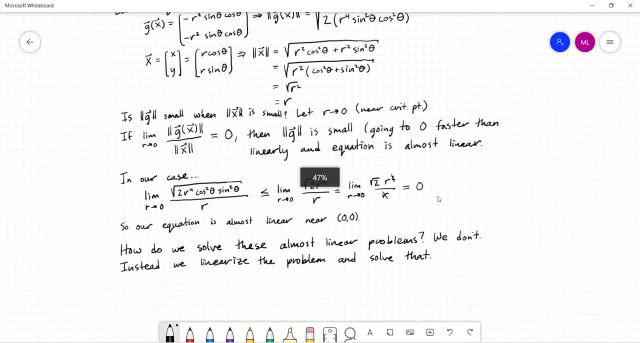 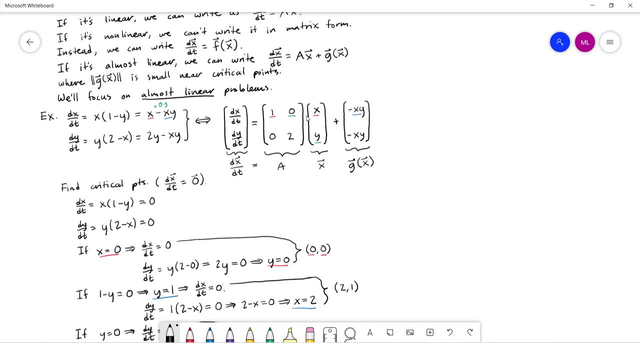 just call it the solution. It doesn't really affect things. The rate of change in our differential equation near those critical points. this part of the equation is going to be interesting. This part of the equation becomes irrelevant. It's very tiny. 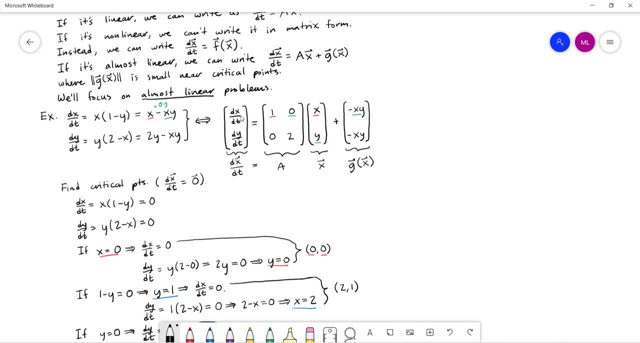 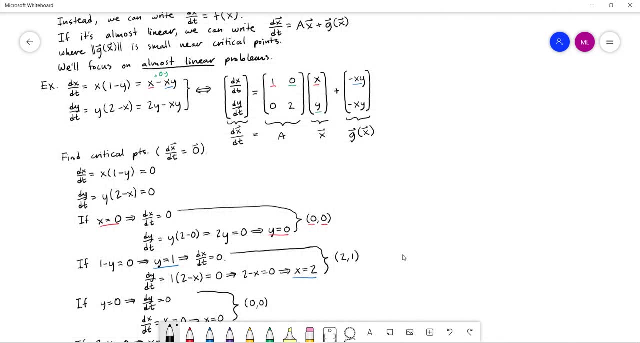 And if this is tiny, then it's not dramatically affecting our rates of change, our dx dt and our dy dt, which means it likewise won't very strongly affect x or y themselves. So linearizing is basically ignoring the nonlinear section by which we can string out the values of r, примерно. So linearizing is basically ignoring the nonlinear section by which we can string out the values of r, lumini, gummy gue. And if we say that we have a Square-Linux slip, then we'd end up nine delta, delta, delta t at number 0 and teta times e. 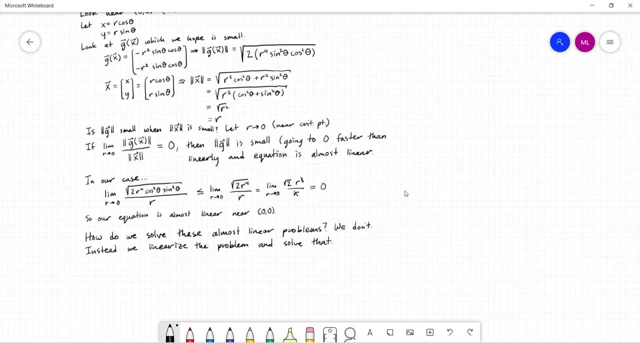 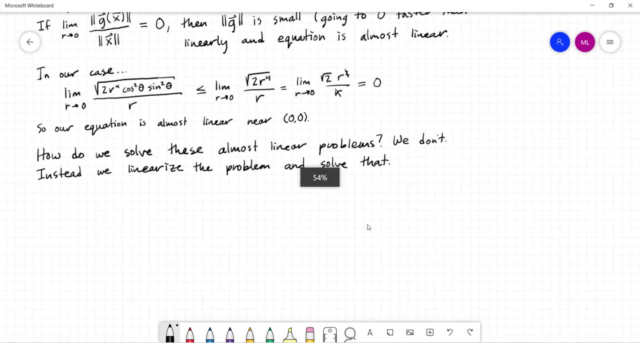 ignoring the nonlinear parts. That's the gist of what it means to linearize the problem. So how do we do this? So we're going to linearize the problem and solve that. We can only linearize near the critical points. There's the only place it'll be a good approximation. 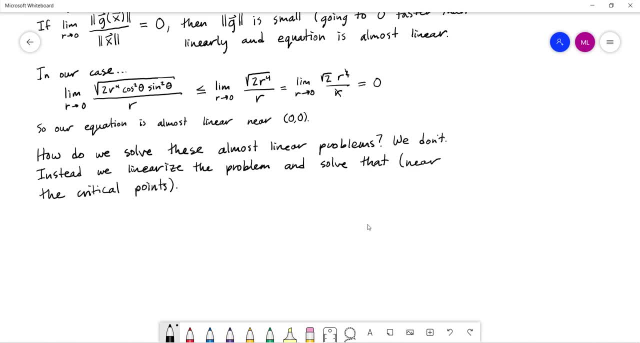 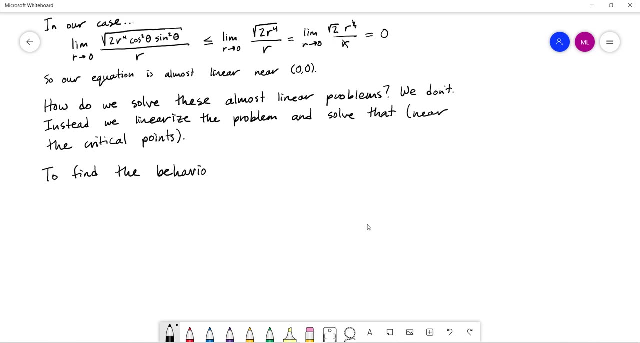 because those are the only points where that nonlinear term becomes unimportant. Okay, so how do we do this? Define the behavior of our system near these critical points? So, near a hypothetical critical point, let's call it x, naught, y naught. 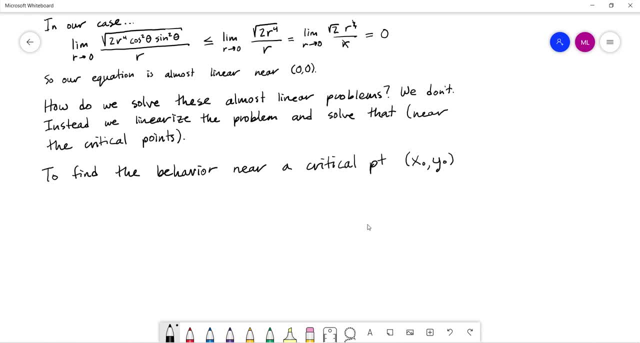 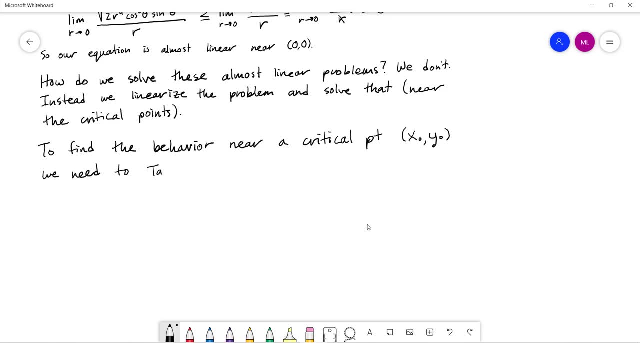 What we're going to basically have to do is tailor expand the original equation. All right, so basically we have to write the tailor expansions of our f and g functions, our capital F and g functions, that we had Equation. So again, let me remind you 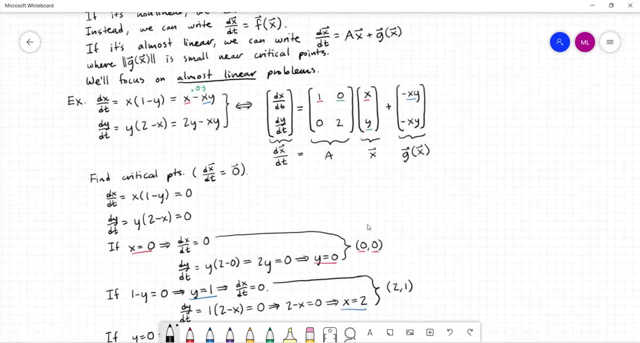 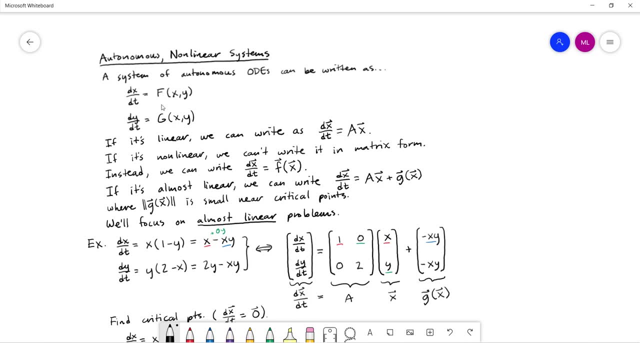 our original equation way, way, way, way, way back up here, right, Generically, we have to write the Taylor expansion of our f and g functions: This f and this g. these are the things that I need to basically find linear approximations of. 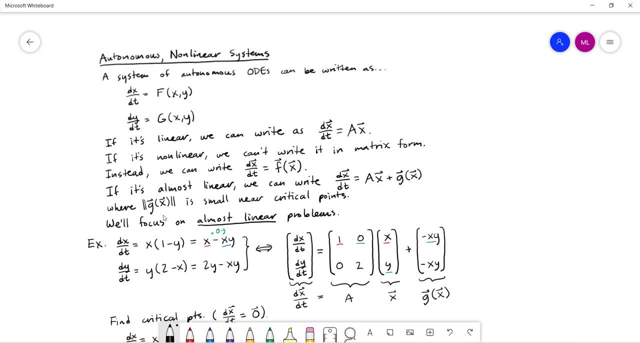 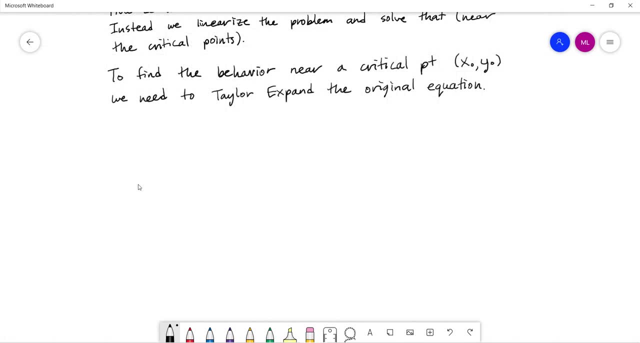 And to do that, we're going to tailor, expand them And, specifically, we'll go through an example similar to this one and see exactly how that works. Okay, so, for example, the f term. So let's say we want that f of x, y, We are wanting to. 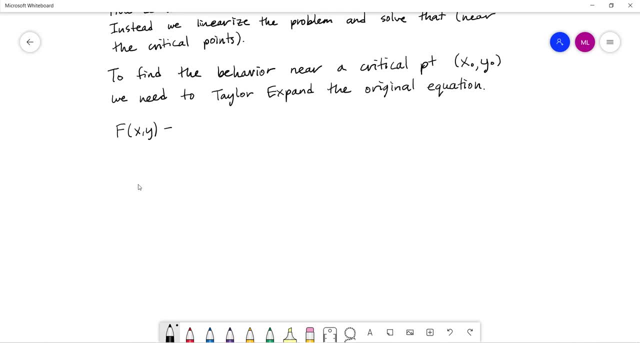 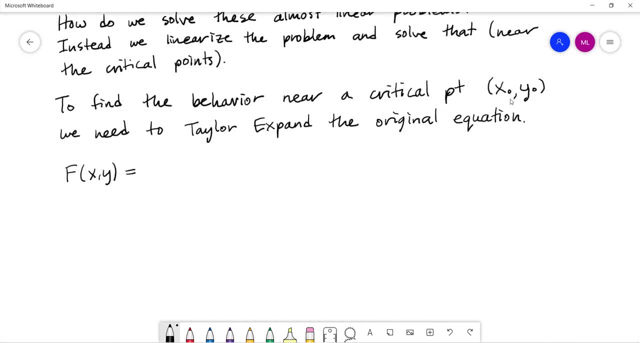 let's say we want to approximate f of x, y via a tailor expansion near the point x, naught, y, naught. So basically, we're expanding around the point x, naught, y, naught. What this requires us to do is a 2D tailor expansion, which is probably not something that you've done. 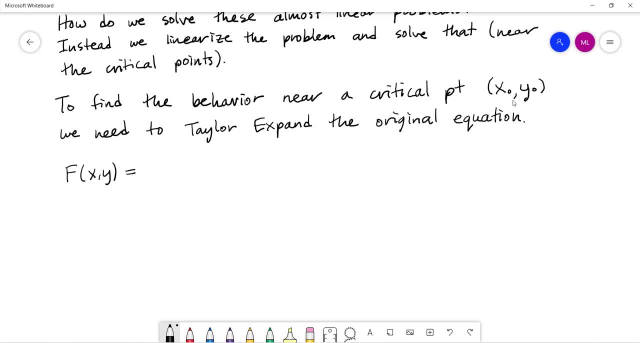 This gets touched occasionally. Some instructors touch it in Calc 3, if you've taken that, but most don't. So this may, or in fact is likely not, something you've seen. But a tailor expansion in two dimensions is likely not something you've seen. 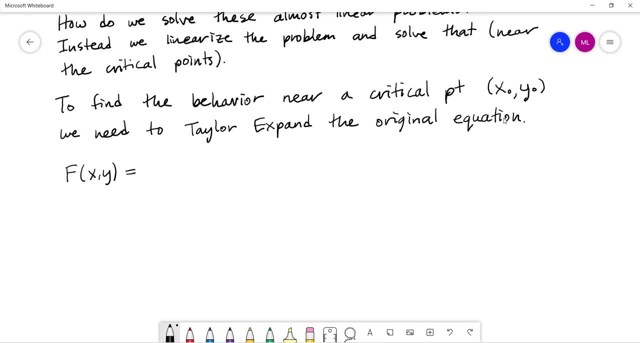 It's not any trickier than a tailor expansion in one dimension. Basically, what we have to do is start off with our constant terms, So you evaluate the function at the point of interest. So here's my order: constant term, right. This is basically. you can think of this as 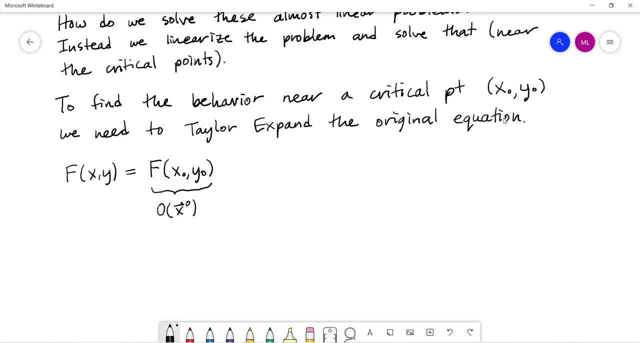 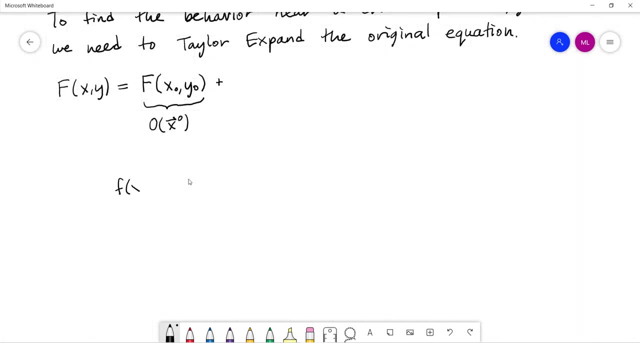 order of the x vector itself to the zeroth right. It's the constant term right. It's not proportional to x or y Plus we'll take the derivatives So normally in a tailor expansion right. So for a normal tailor expansion, if I wanted f of x, 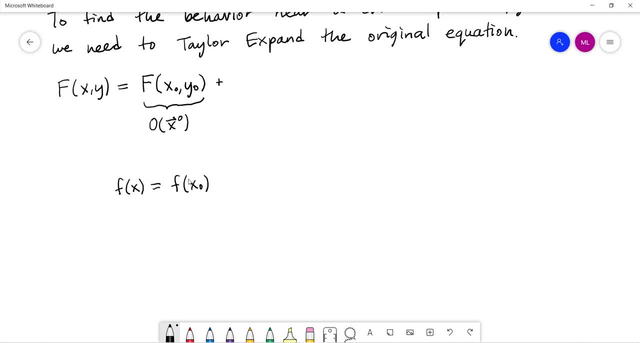 it would look like we'd evaluate it at the point x naught. Then we do f prime evaluated at x naught times x minus x naught, plus f. double prime of x naught times x minus x naught, squared over two factorial plus yada, yada, yada. We're doing the same thing here, but now these. 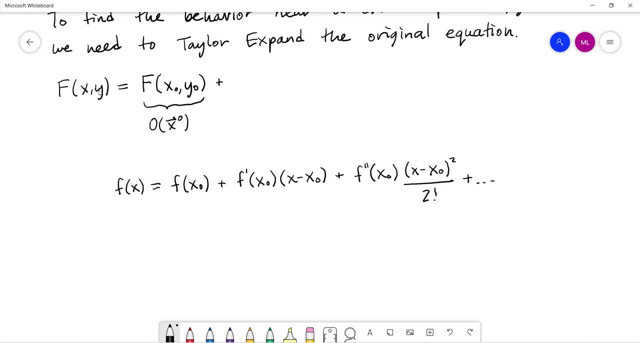 derivatives are ambiguous. So we're doing the same thing here, but now these derivatives are ambiguous. So we're doing the same thing here, but now these derivatives are ambiguous Because we have functions of two variables And in fact, we need to take derivatives with. 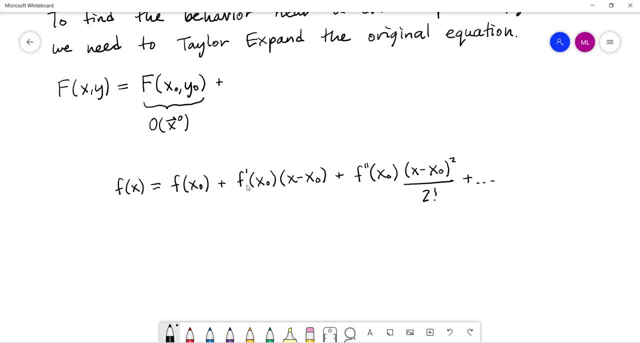 respect to both of those variables. So the first term is going to be the x partial derivative evaluated at x naught, y naught, So the rate of change in the x direction. we multiply that times x minus x naught. But we also need the rate of change in the y direction, So we do f of y. 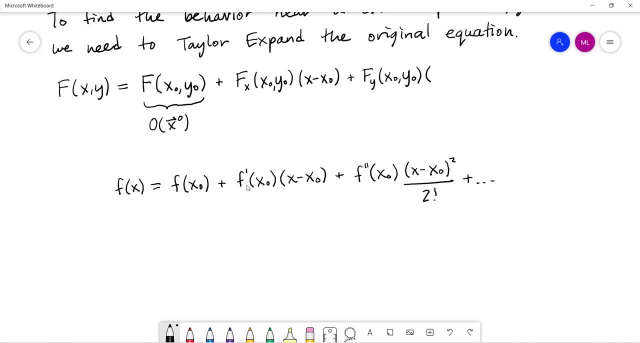 f sub y of x naught y naught times y naught, squared over two. So we do f of y, f sub y of x naught y naught times y naught squared over two. So we do f of y, f of y, f sub y of x naught y naught, squared over two. 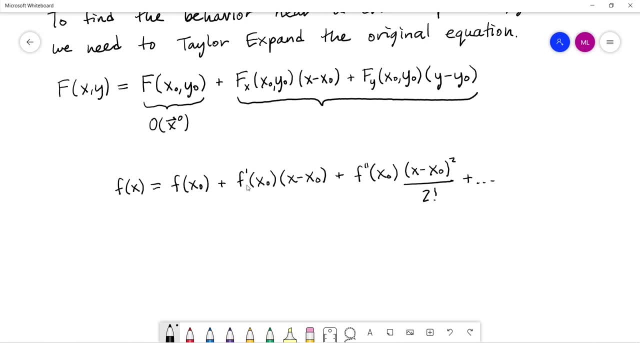 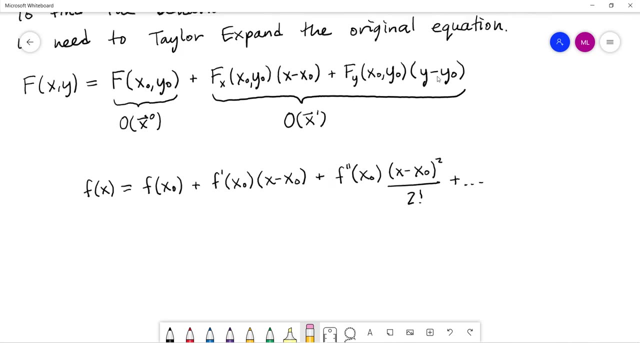 These two terms. they are both order, our x vectored to the first power, and what I mean by that is they are both linear terms in either x or y. After this would come the combinations of all the second derivatives, But there are a lot of different second derivatives. There's the x- x derivative, we find z, we find y, we find y, we find y, we find the two derivatives, but right, there's a lot of different second derivatives. right, there's the executioning, right there's the xx derivative, there's the f of y, y, y and y. 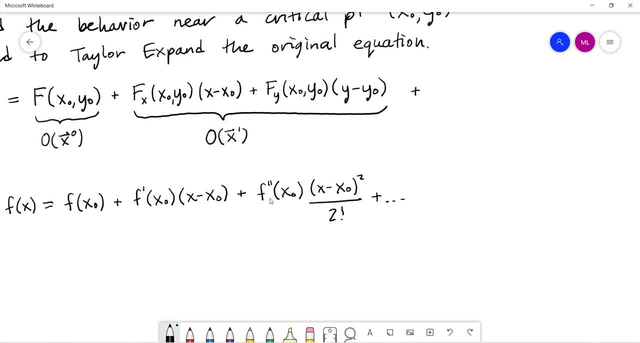 the xx derivative, the xy derivative, the yx derivative and the yy derivative, And we would have to account for all four of those over here. But luckily we would also wind up with either an x minus x naught squared term or an x minus x naught times a y minus y naught in the case of. 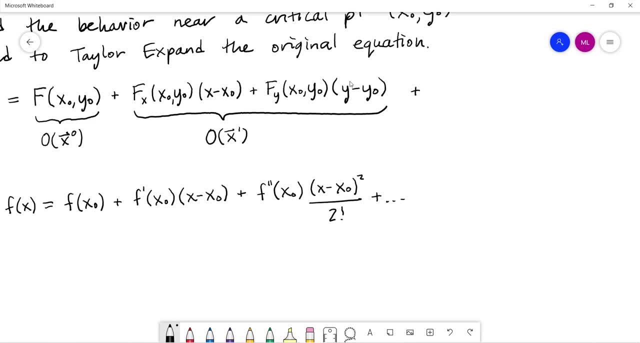 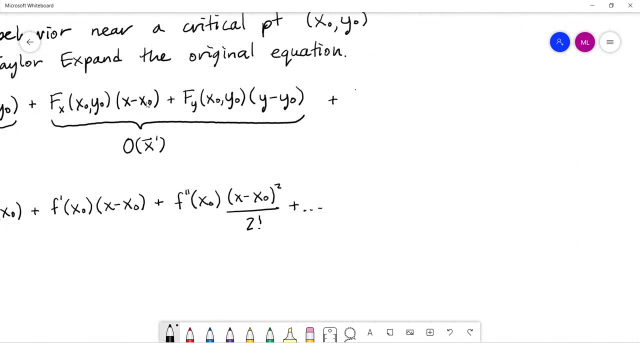 one of the mixed xy derivatives. So basically, right, the variable here matches the derivative that's being taken here, right? So this is basically a linear term in y matching the y derivative. This is a linear term in x matching the x derivative. Hypothetically, if I did the 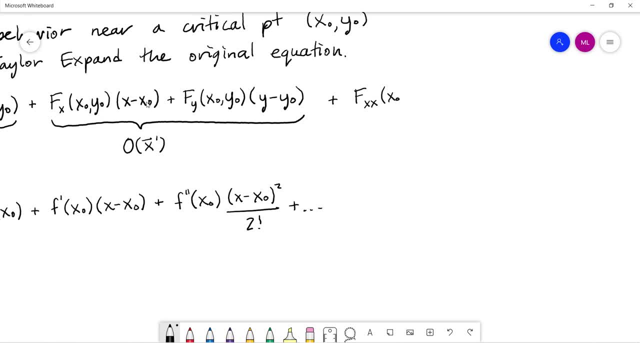 first of the next terms. so the fxx derivative. it would look like this: And I would have to multiply by x minus x, naught squared, And again we do over our two factorial and all of that. But notice, this is the only one of the many terms that will show up. We'll also have the fx. 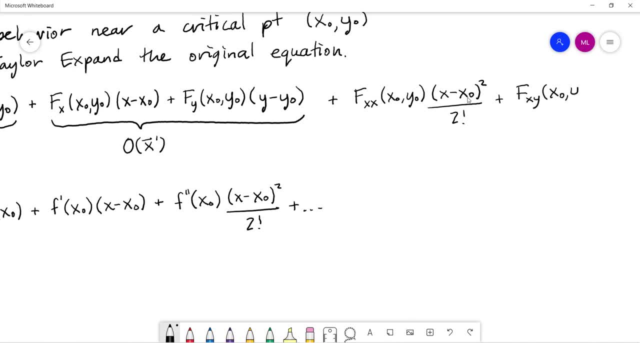 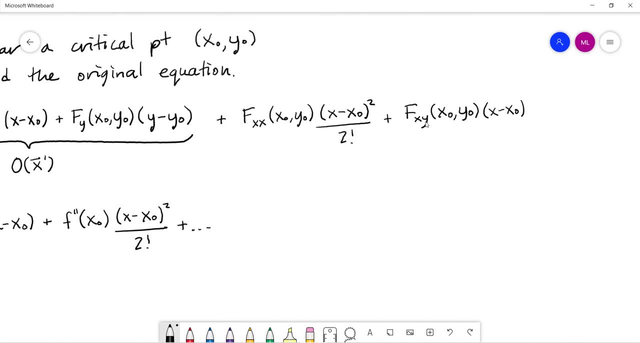 xy term And that would be of x naught, y naught, And because I have one of each derivatives, I'd have one x minus x naught, but I'd also have a y minus y naught And combined again. 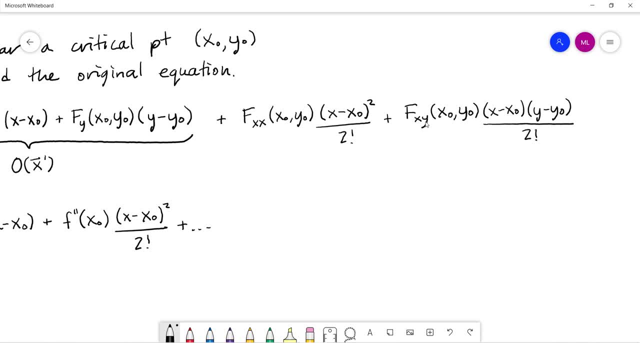 both of these. we've got to divide this by two- factorial, but we're also going to get two of them because we're going to have two mixed partial derivatives. So we'd have an extra two out here, plus we'd have the fyy term. 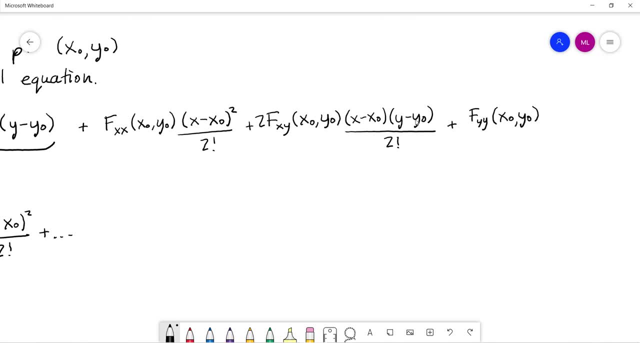 So let me just write this out, even though we aren't going to need this term, But this is what a 2D Taylor expansion starts to look like, Plus I'll then the cubic term. So all of these are the order x vector. 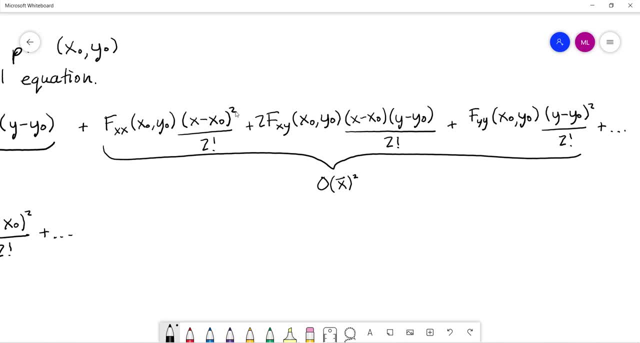 squared terms right. They're all the ones that are either quadratic in x, quadratic in y or quadratic in a combination of x and y. right Linear in x times linear in y gives us a quadratic sort of in the mixed xy variable. 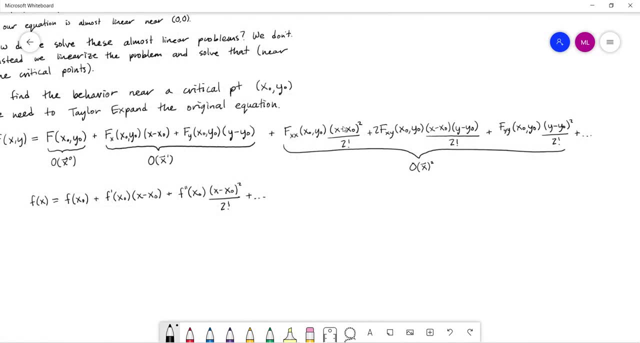 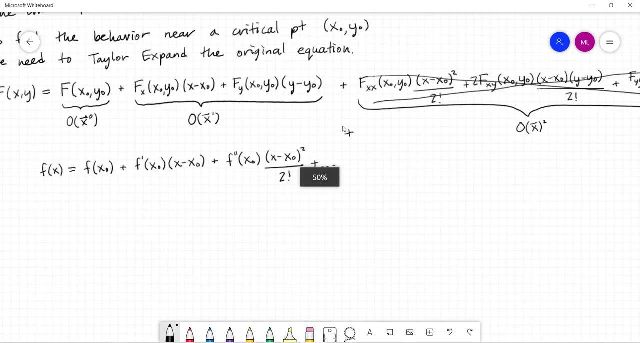 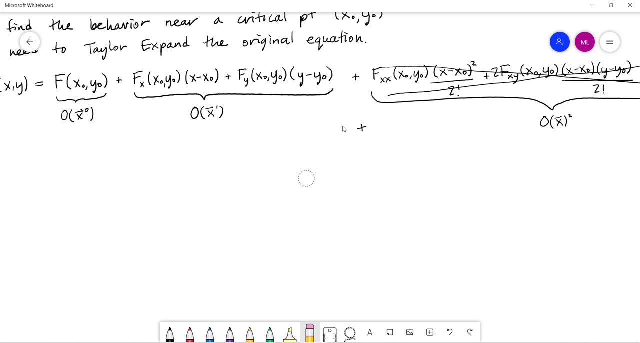 So these terms are the terms that we're going to dramatically simplify and say, instead of all of this, let's not write these out, Let's just say that these are, plus some additional term, And let me come down here and just erase our one dimensional Taylor expansion to get it out of the 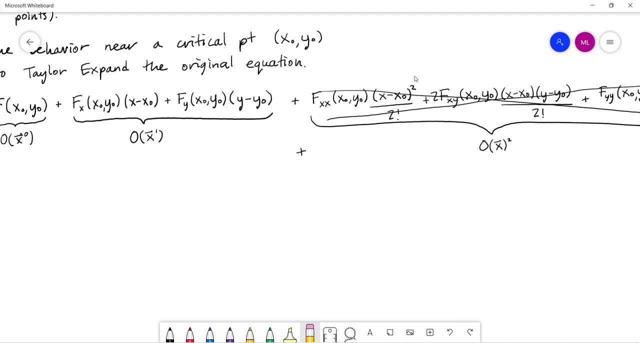 way, But clearly all of these terms are basically some function that involves both x and y and its higher powers of x and y. right, They're quadratic, So oftentimes what winds up being written is something like this. I'll call it Greek letter. 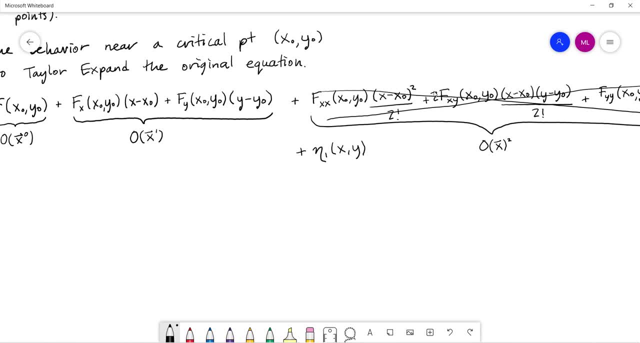 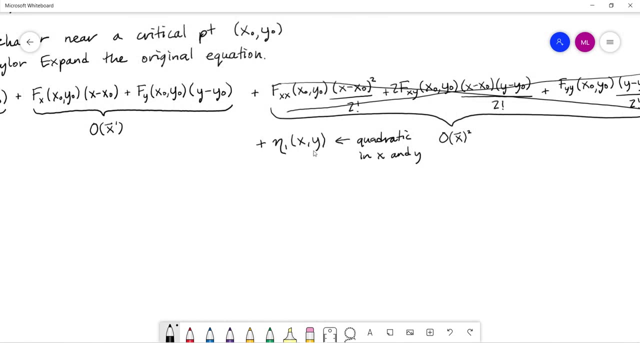 eta. we'll call it eta one of xy, And it's again quadratic in x and y. So just keep in mind, instead of writing this whole term out, I'm just saying we're going to add this term And this. 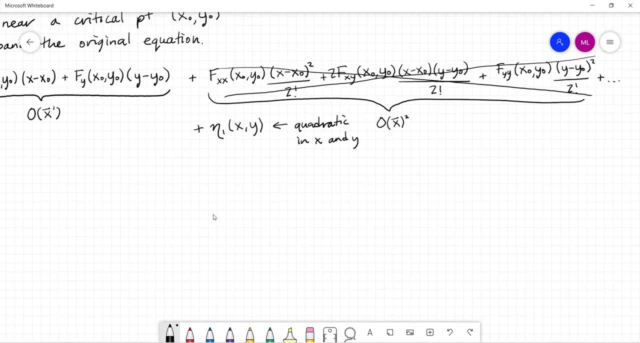 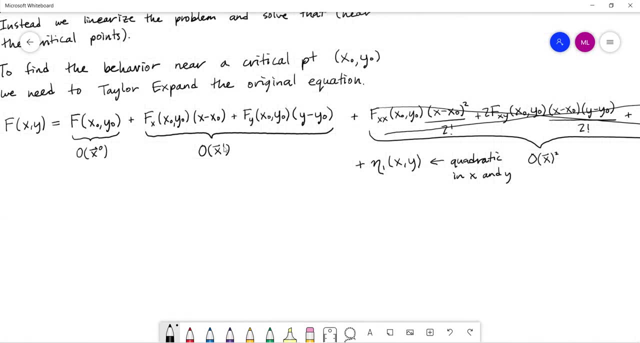 term is going to include these quadratic terms plus the cubic term, So it's basically the whole round off error after we've kept our constant term- our order zero term- and our linear term- our order one term. So these are the only terms that we're keeping for. 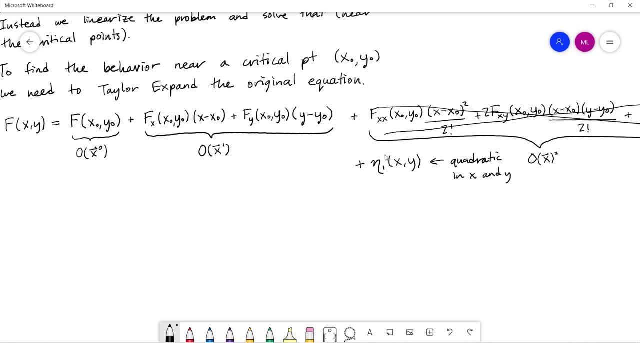 our linearization. everything else is quadratic or higher, So this highest order of this term is quadratic. we're just going to condense all the rest of it. this is all of our round off error, And we're condensing it into this one term. 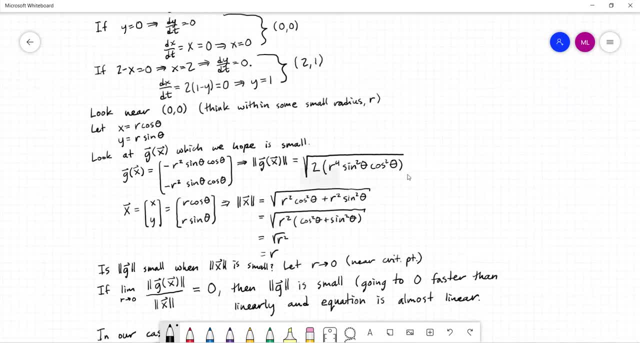 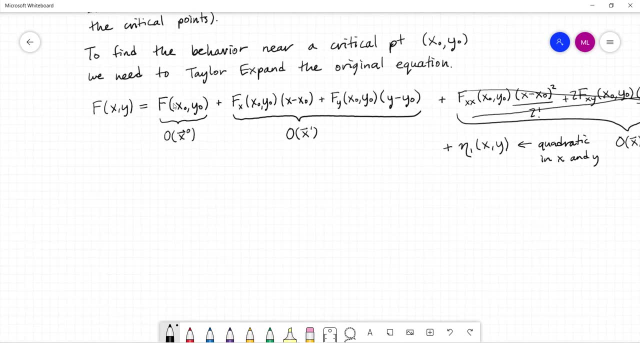 So once we've done this for f- remember we don't just have f, we also have g. So let's do the identical thing in g. Let me just write that down real quickly: g of x- y will look very similar. Oops, It will look like this And it will have: 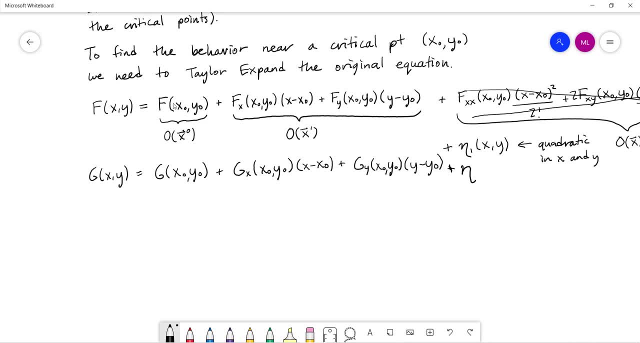 some we'll just call it some eta two terms. So it will also have all these higher order terms that are a function of x and y. they're both quadratic. So this piece just reminds you that eta one went with the first one, eta two is with the bottom one. So at this, 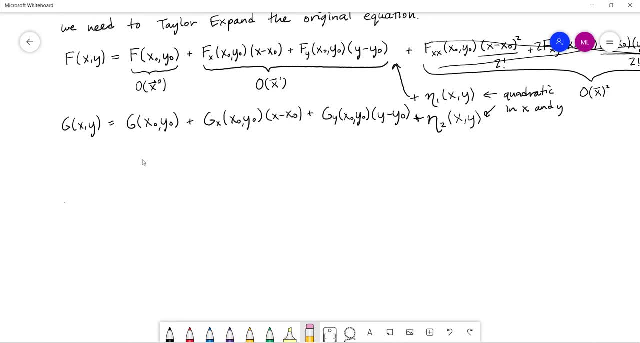 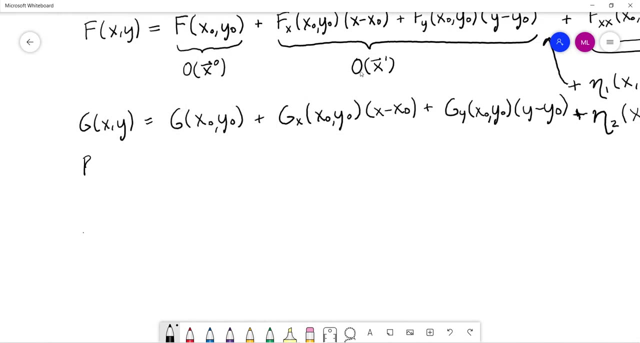 point. we want to replace the f and g in the original system of differential equations with their linear approximation. So what we're going to do is replace- oh, my hand right here is getting bad there- Okay, Replace f and g in the original system with this term. 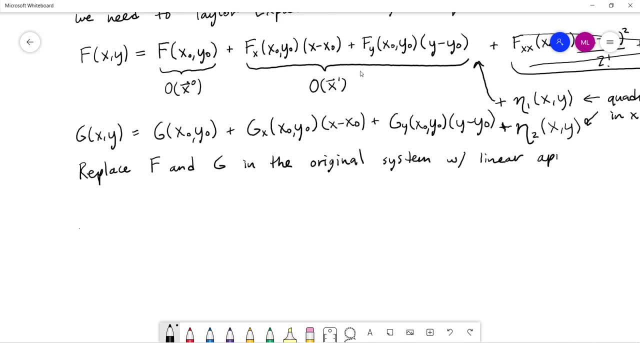 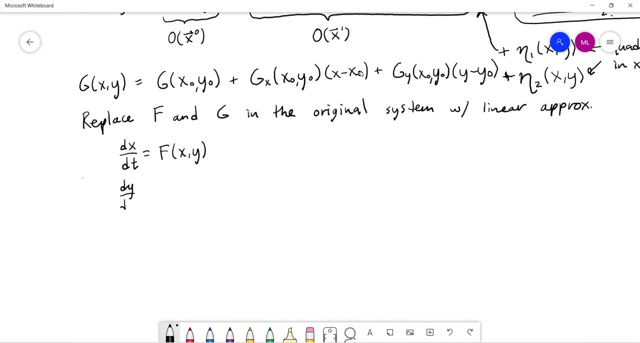 that we've now found to be the linear approximation, basically with this Taylor series that we just found. So the original differential equation, you'll recall, was that dx- dt was equal to f of x- y and similarly, dy dt equals g of x and y. And I'm arguing that we're going. 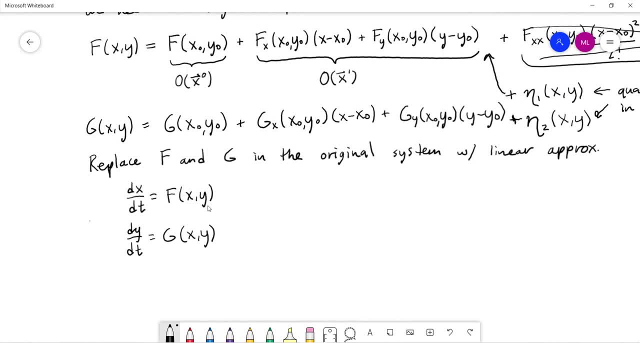 to go replace these with their linear approximation. So the f is going to become so this equation will become: dx. dt equals f of x zero, comma y zero plus f. sub x of x zero y zero times x minus x, not plus f. sub y of x- zero, y zero times y minus y, not, and technically plus. 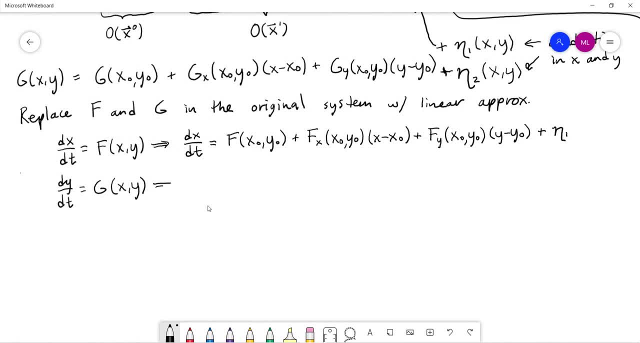 that eta one terms, those non-linear terms that come afterwards for the other one we get: dy dt is equal- sorry, not f. dy dt equals g of x, not y, not plus f of x minus x. And once again, this kid just called this original system of differential equations and put it. 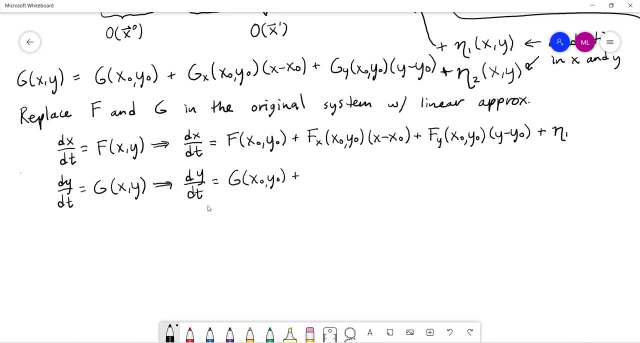 correctly, we got dy dt. so this is the Minneapolis phenomenon, And then of course we had toümüz that one too. So there are general expressions that just specify something like x minus x, y0 plus g sub x of x0, y0 times x minus x0 plus g sub y of x0, y0 times y minus y0 plus. 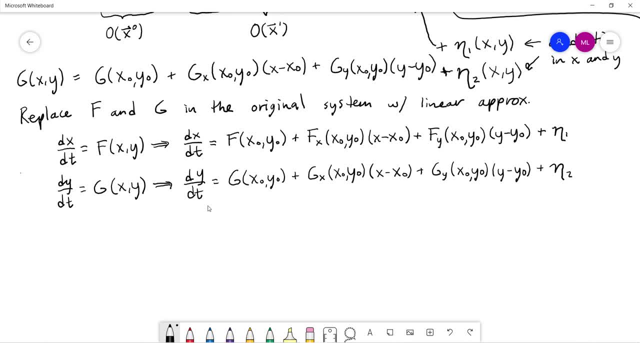 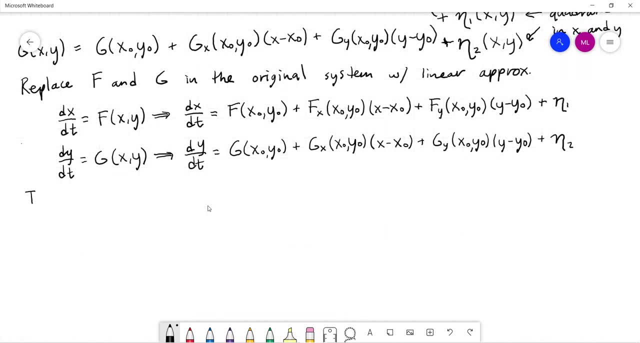 eta2.. It's associated to nonlinear terms And I want to think about a couple of things. So, number one: if the point x0, y0 is a critical point, then basically, which is what we're arguing here? then f of x0 and g of x0, y0, I should say 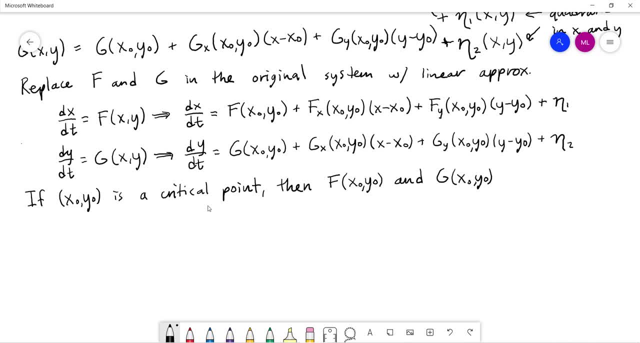 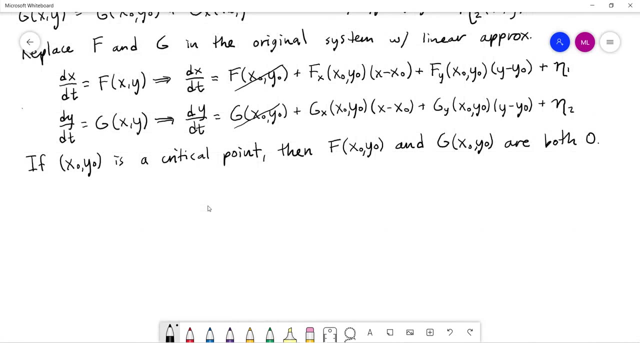 So f evaluated at that point and g evaluated at that point are critical points, Both zero. So basically I'm arguing we can knock those two terms off. The next thing I want to do is make a substitution. If we define so, let's introduce some two new variables. Let's let u be equal to x minus x0.. 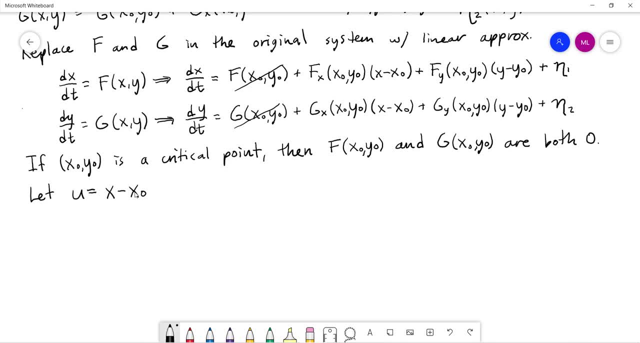 So basically, if the old point x0, y0 was the equilibrium point, we're essentially recentering our coordinate system. So basically we're making, we're changing where the origin is. So we're going to let u be equal to x minus x0,, v equals y minus y0.. And basically now, when you go to the 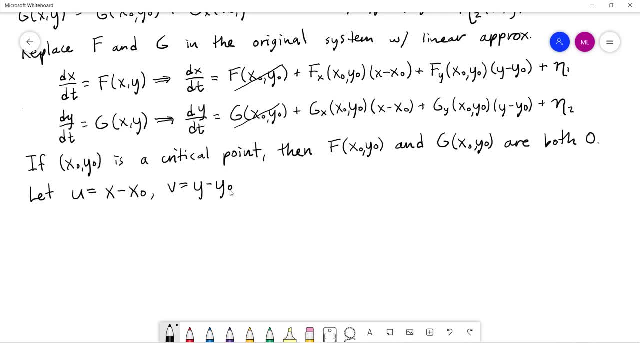 point x, y, that's on top of our critical point x0, y0, in terms of u and v. it puts you at the origin in terms of u and v. So the point zero, zero. So basically we've. 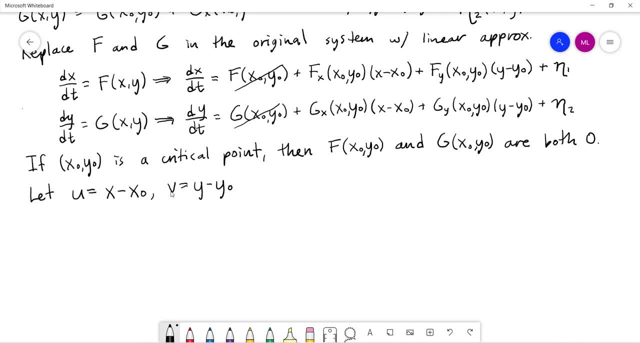 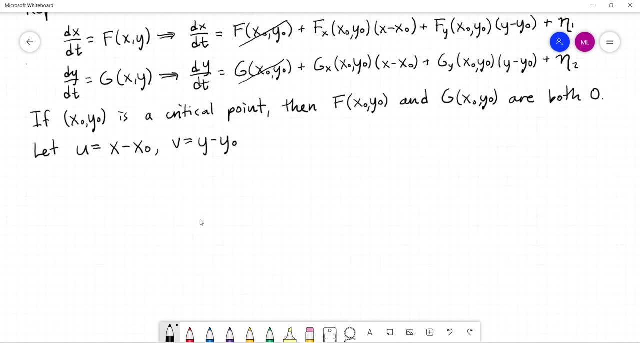 recentered our coordinate system around the critical point. So the critical point is now the origin in terms of u and v. The nice thing about doing this is it doesn't affect the derivatives, So, like du dt, for example, is going to be the same as dx dt, right, Because this is a constant. So the 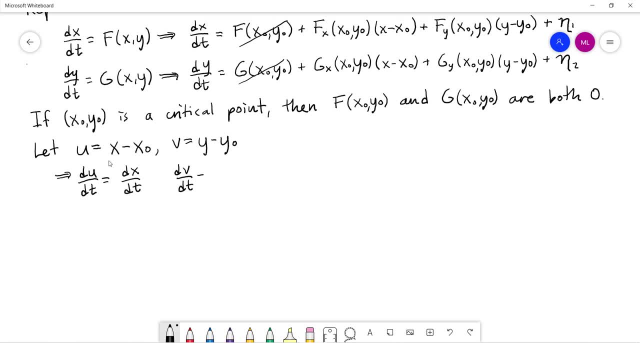 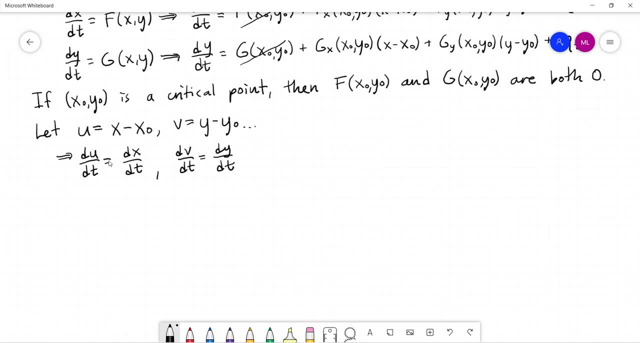 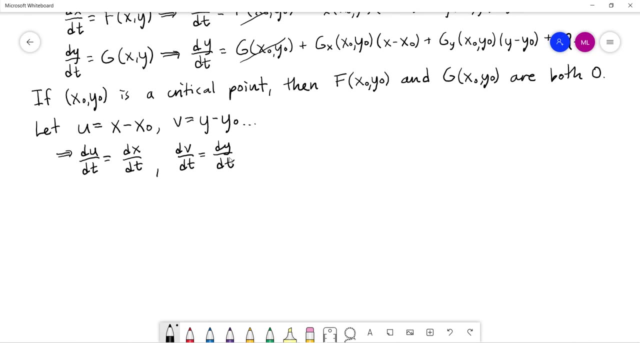 two derivatives are the same And similarly, dv dt is equal to dy dt. right, So we've let those two variables change. Their derivatives are equivalent. du dt is equal to dx dt and dv dt is equal to dy dt, And we can now actually go back and simplify. 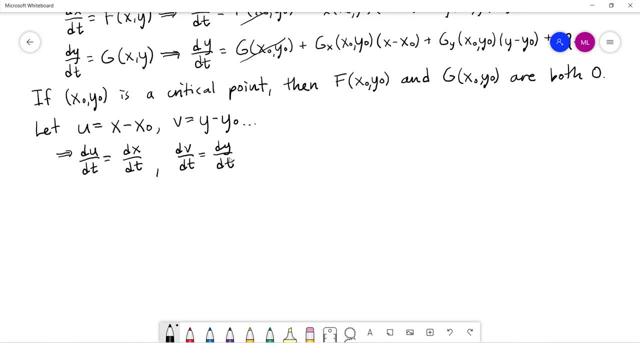 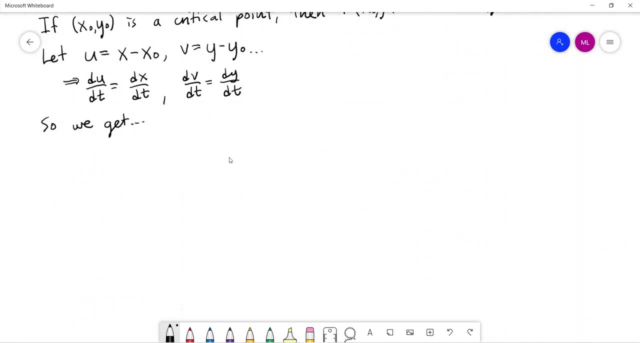 the way that everything looks, Our differential equation becomes, or our system of differential equations becomes, the following: That dx dt we are going to replace with du dt because, as we just showed, they're equivalent, du dt is now going to be the same as dx dt, So 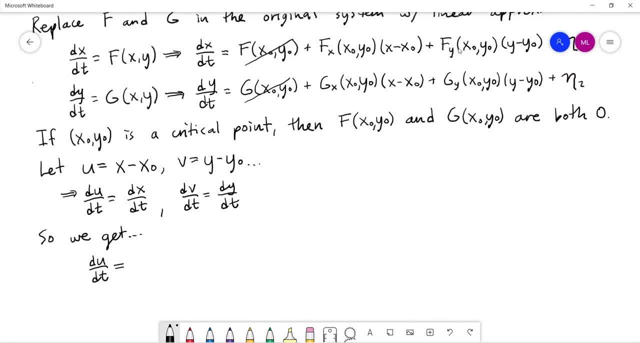 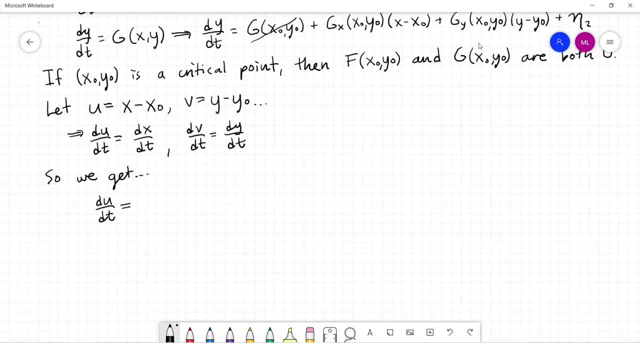 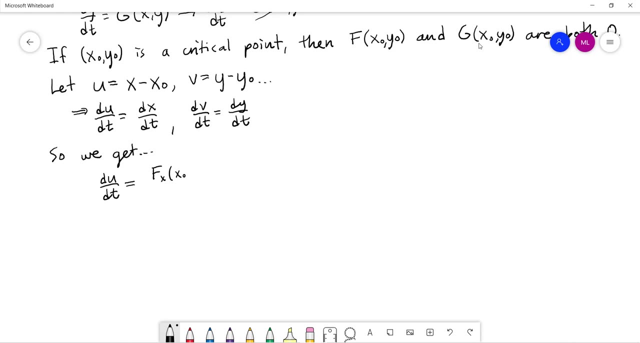 dx, dt is going to be equal to these remaining terms. So it's basically f sub x and f sub y, evaluated at the critical point And in terms of this. so let's write it out, Let me just write them all. So f sub x, x naught, y naught, And that was times you'll recall. 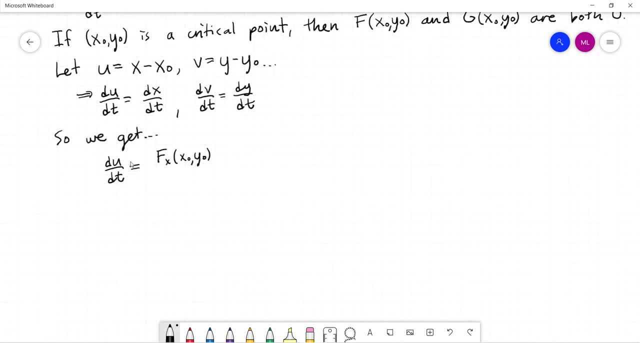 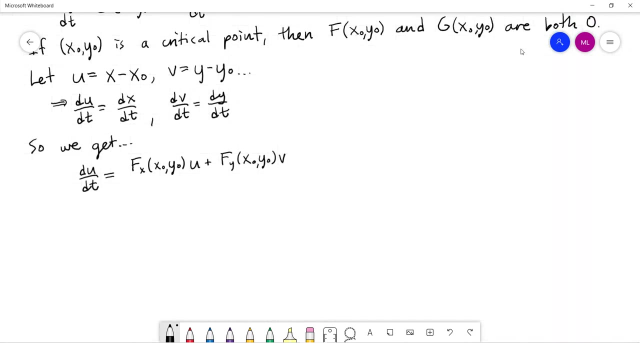 that was times x minus x naught. but we've just defined that to be u plus f sub y, evaluated at that same point, times v, because it was being multiplied by y minus y naught. And for the other equation, dv- dt, we're going to get g sub x of x naught, y naught times. 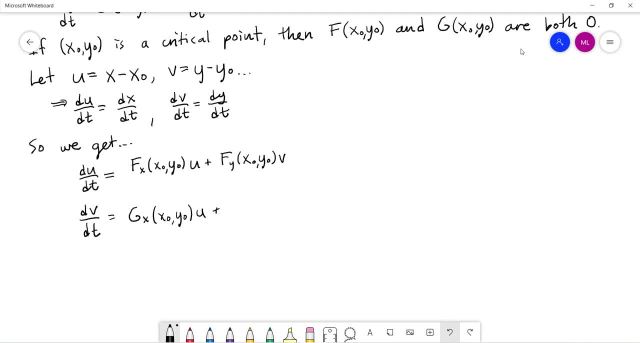 u plus f, sorry, g, sub y of x naught y, naught times v, And we're going to basically drop the nonlinear terms. So this is our linear approximation. So we're dropping eta 1 and eta 2, which are small, to get a linear approximation. So this: 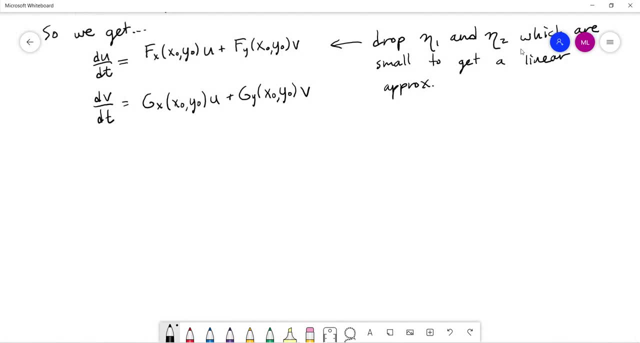 is our linear approximation, And the nice thing about it is that we're going to get a linear approximation, So we're going to write it into the vector form. So what we're going to do is we can clean it up a little bit and basically write it in sort of our vector form. We could think of this: 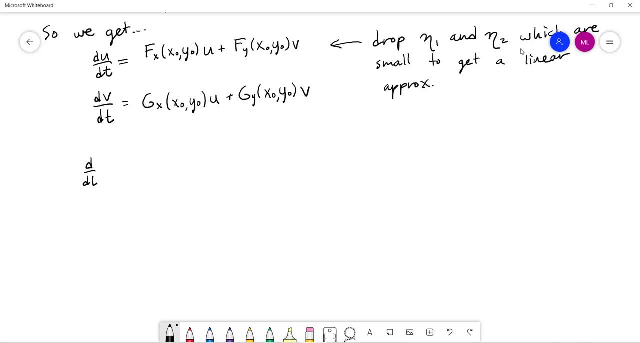 as d dt of the vector u and v equals some matrix times u and v, because, notice, that's exactly what is multiplying, And so the matrix that I need to hit it with is f sub x times u, so this needs to be the f sub x. 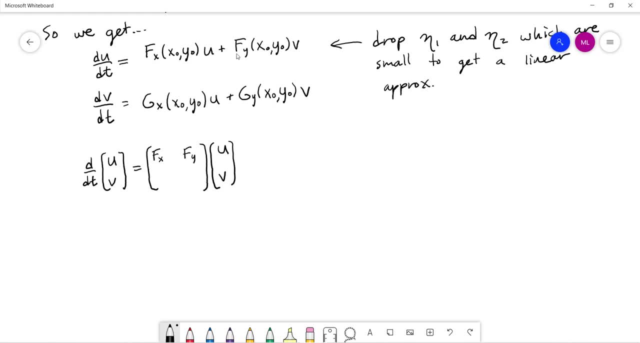 Then f sub y, then g sub x and g sub y, and note that we are evaluating this at the point x naught, y naught. right, each of those terms is evaluated at x naught and y naught. this matrix right here is called the jacobian. 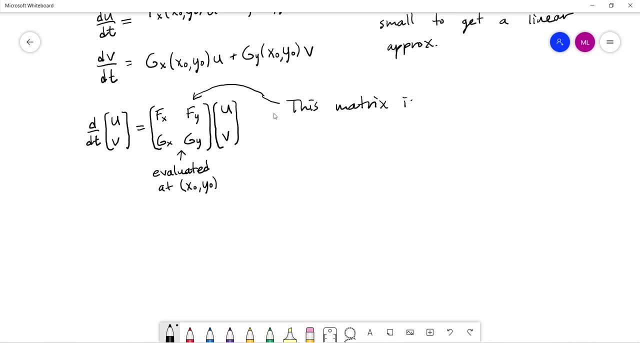 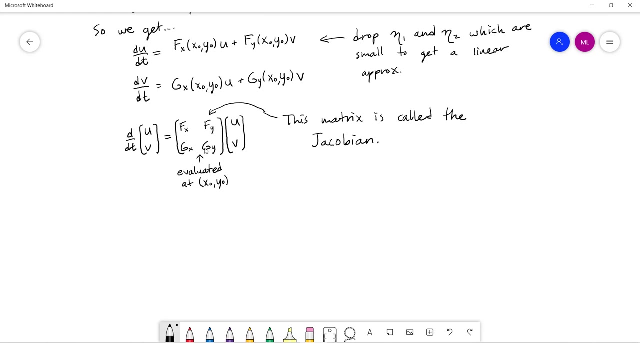 the jacobian and essentially what we're doing. if you think about a higher dimensional taylor approximation, if you think about sort of this existing on the surface, we're finding a tangent plane and all of these are essentially the slopes in the x and y directions of these. 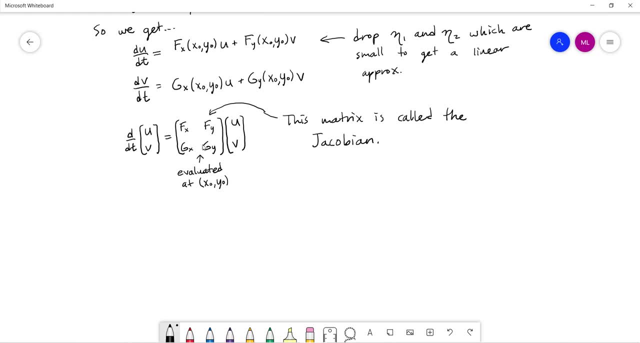 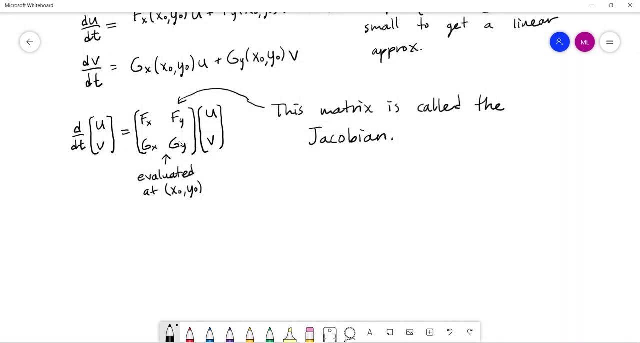 two different functions, that that we're using to prescribe the, the surface of the equation, and so we're going to do that, and we're going to do that and we're going that we're dealing with in a sense, so the jacobian is the name of this matrix. 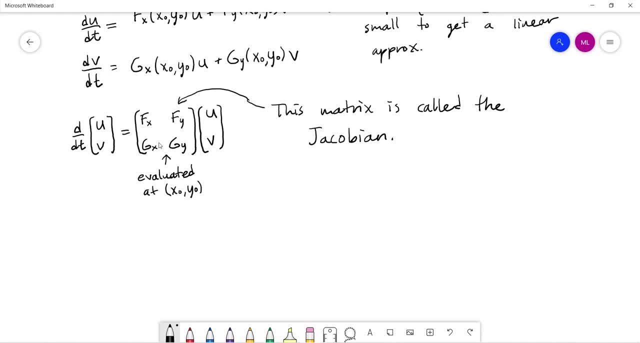 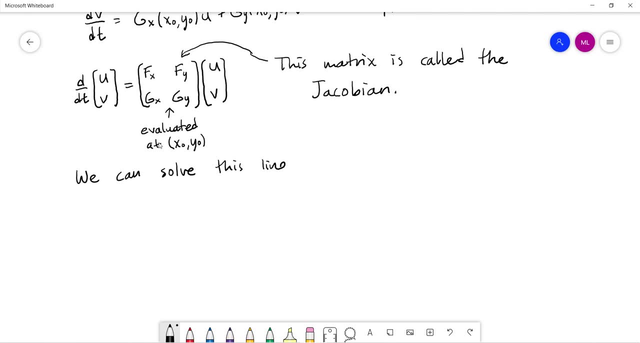 and this gives us a linear system. we can solve this linear system for the behavior near the point of interest, so near x naught, y naught to get an approximation of the non-linear system in that same neighborhood, so in that same region. so let me do um. 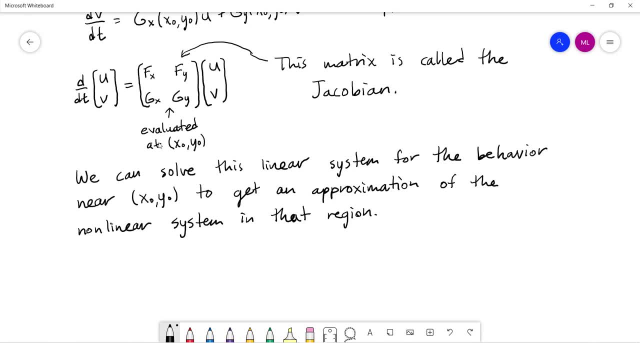 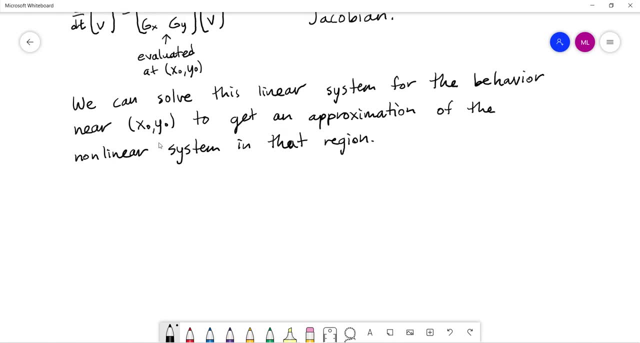 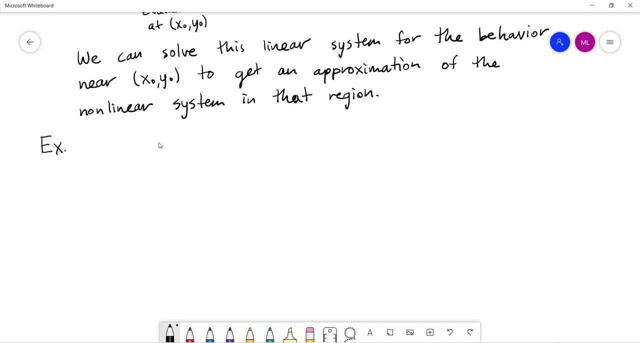 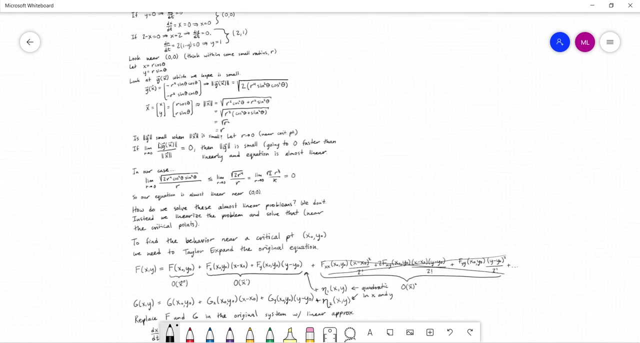 a quick example to see kind of how we can put this to use. um- and it's bear with me, because it's kind of- uh, these examples tend to be kind of nasty- um, let's actually you know what, let's just go ahead and do the one that we just started with up here. 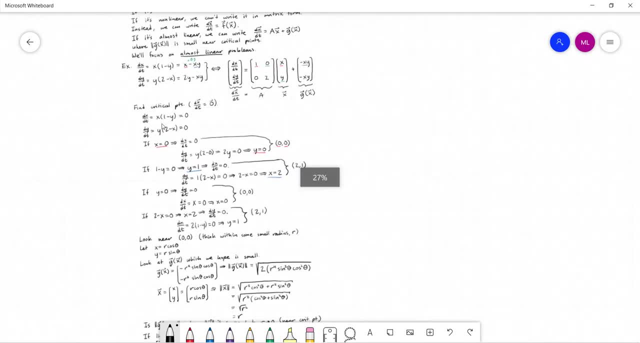 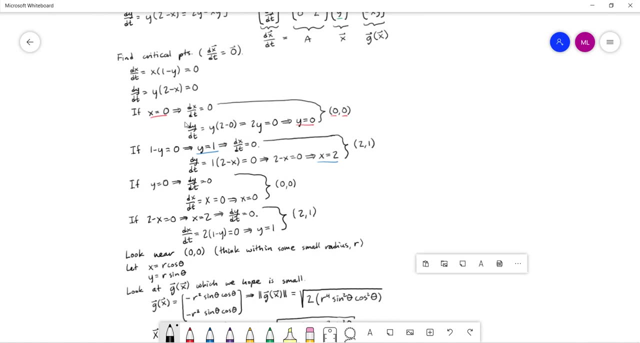 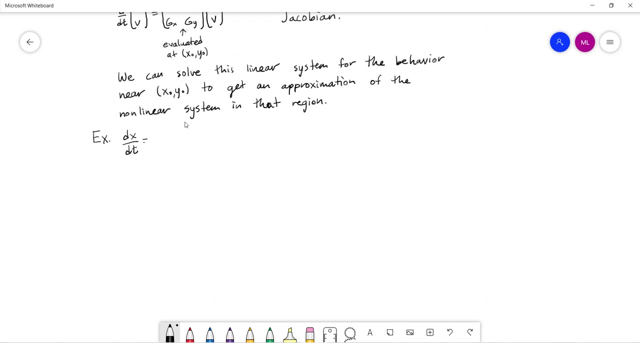 so let's do this one, since we've already done a bunch of the work on it. let's actually get a little bit more information. so let's do. what is this? dx dt, dy dt equals okay. so it is: dx dt was equal to x times 1 minus y and dy dt was equal to y times 2 minus x. 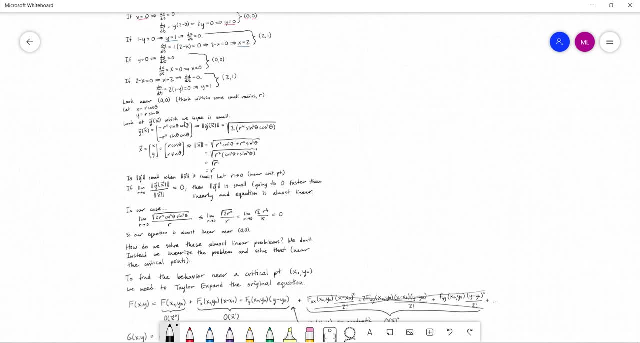 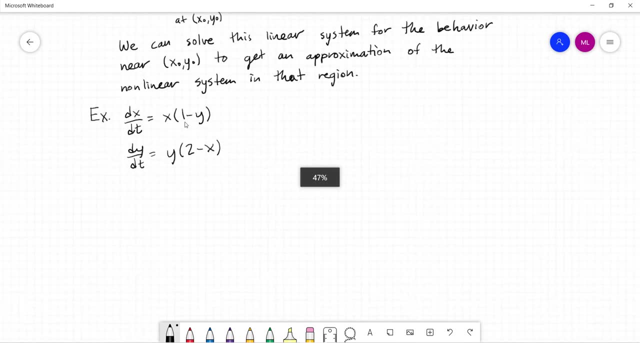 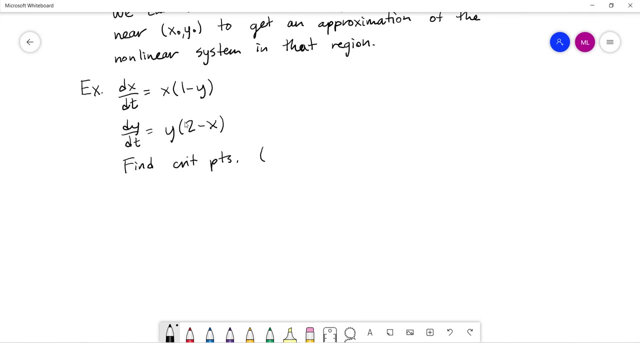 let me just make sure that i copied that down correctly: y times t minus x, x times 1 minus y. okay, we already found the critical points. they happen to be 0, 0 and 2- 1, and so what we need to do is linearize this equation around each of those two points. so let's start with um. 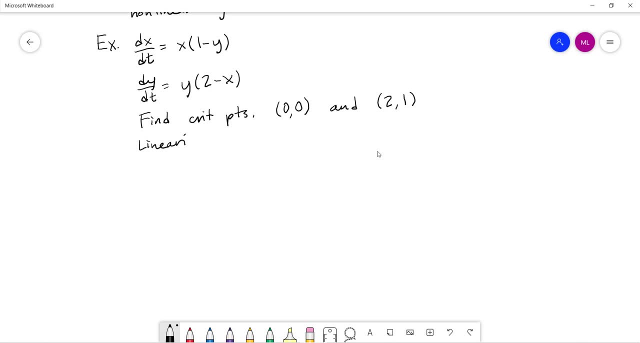 so let's linearize, linearize. come on here each point. so let's start at 0: 0, so at 0: 0. this will be the first point that we look at. so the first thing i need is basically to decide if i need to shift my variables. in this case, i'm going to let u be equal to. 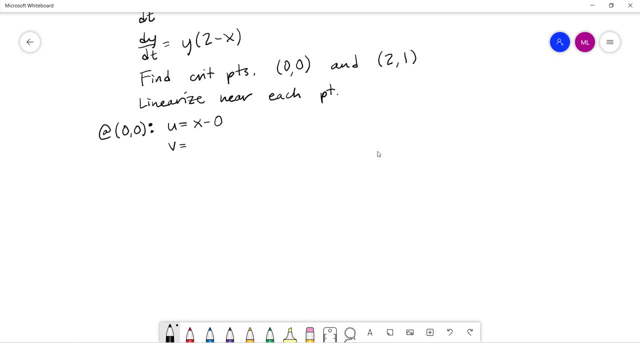 x minus the appropriate x naught, which is zero. v equals y minus zero. the zero and zero that got picked out are because those were the points um, where our critical point is actually located. so if we wanted, in this case we could have totally just stuck with the original variables x and y. 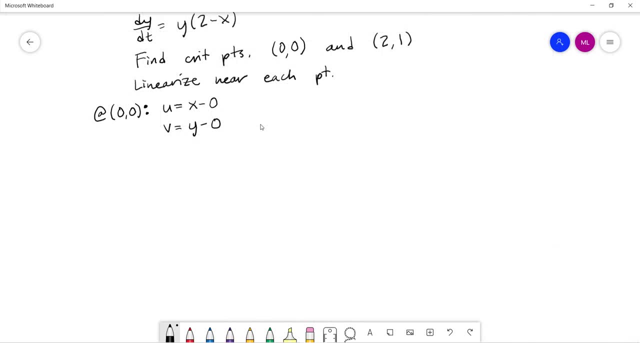 but in general, we're going to switch to these new variables u and v, so we need those and we also need the jacobian, evaluated at 0, 0.. 0, 0 and the jacobian is just the original variable. x and y, the original variables were called房x. 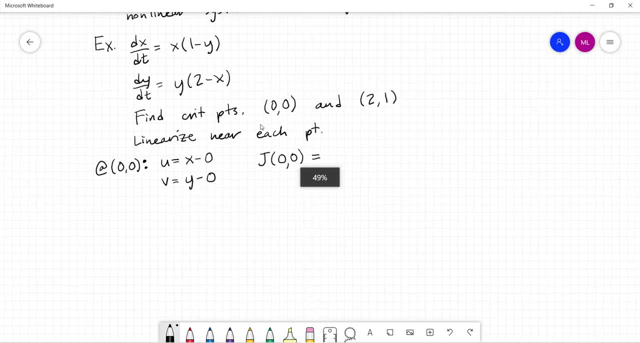 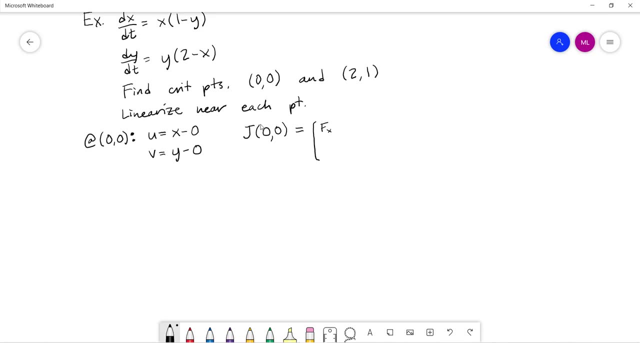 at 0,. 0 is all we need. So again, let me remind you. coming back to the whole thing, it is f sub x, f sub y, g sub x, g sub y, where this top term is our f and this bottom term is our g. 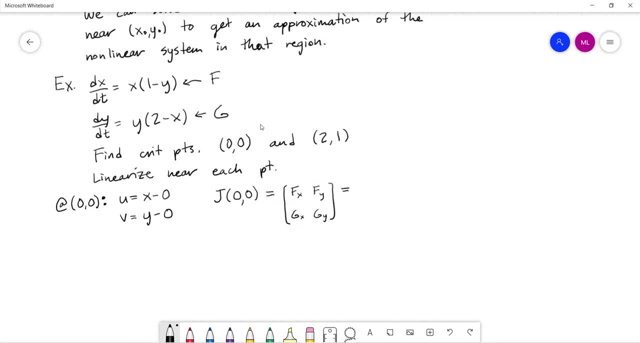 And so for us it's good to, in general, maybe we can find the general, Let's find the general Jacobian up here. Our general Jacobian at a point x, y of our choosing is going to be the x derivative of this, which you'll recall. 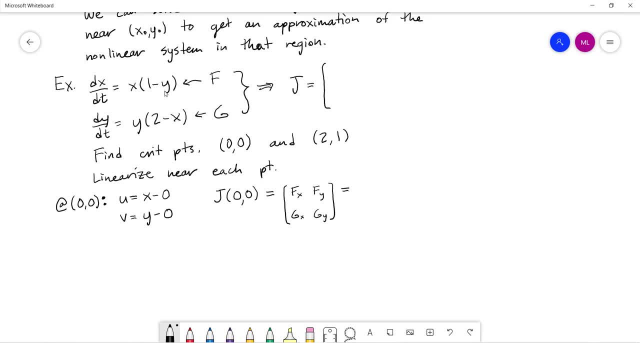 you can either do it in this factored form or you can distribute through and find that. But the derivative of this with respect to x is going to be easy, Because We're just treating y as though it were a constant and the coefficient of x is 1 minus y. 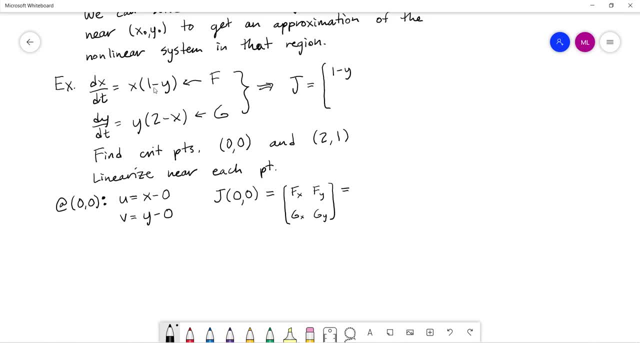 So we're just going to get 1 minus y for the derivative of this with respect to x. For the derivative of this with respect to y. it might be easier to actually distribute through. So really, this is x minus xy. What's the derivative of x minus xy with respect to y? 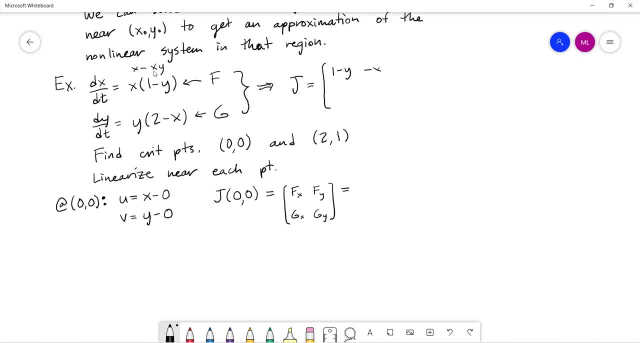 It's going to be a negative x, So we'll get negative x here. Do the same thing down here. We need g of x and g of y. So what is the x derivative of this? That might be easier if we FOIL this out. 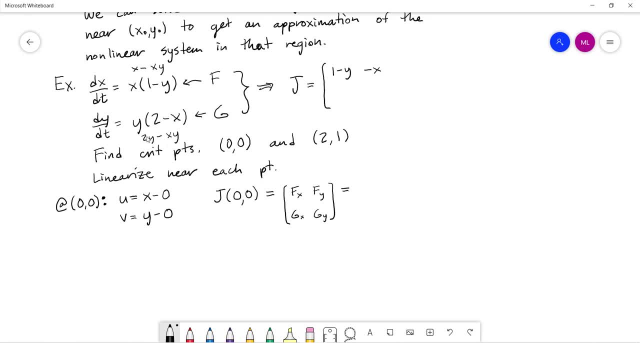 What's the derivative with respect to x? Well, this term has no x's, so the derivative is 0.. But this term the coefficient of the x is a negative y, So we're going to get a negative y down there. 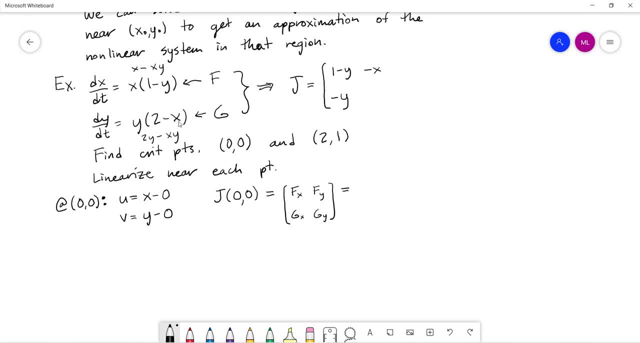 And then, lastly, we need g sub y, So the y derivative of this whole thing, which is going to be 2 minus x. So here's the Jacobian in general. It's just made up of those four derivatives, partial derivatives. 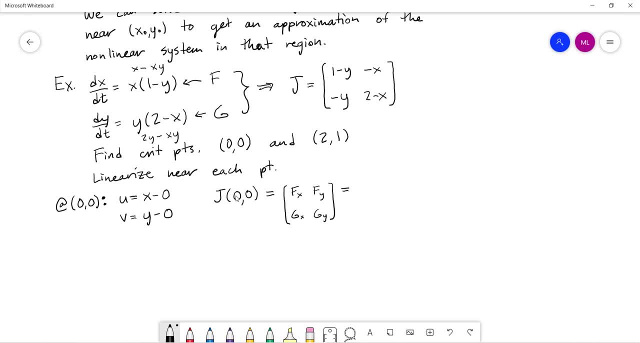 of these pieces that we've got over here, And now we're just going to evaluate it at the point 0, 0.. So for us, if I plug in 0 for x and 0 for y, I'm going to get 1, 0, 0, 2.. 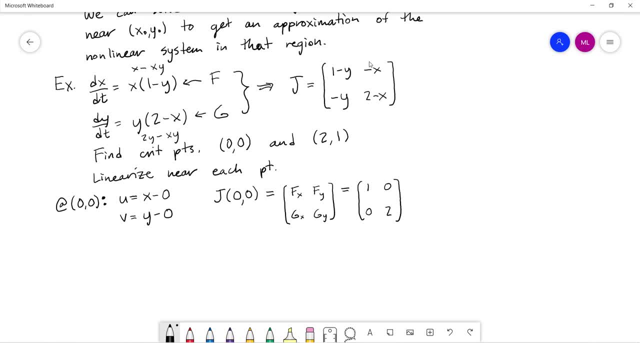 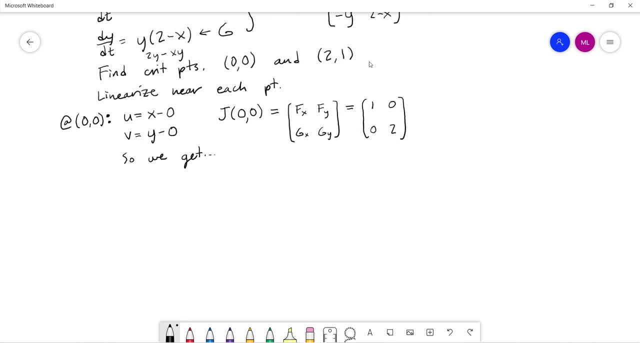 So there's what the Jacobian looks like near the origin, And so our system, Our linearized system near that point is basically: we have something that looks like this: We have du, dt, dv, dt. Let's do it like this, it'll be easier. 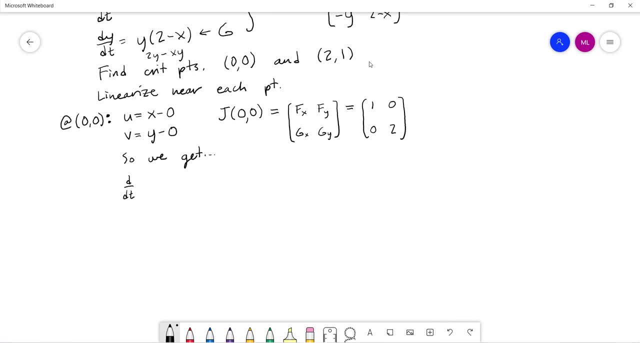 That's right. Oops, So let's write it as d dt of u and v equals 1, 0, 0, 2 times u and v, And so here's our linear system that we need to solve. All we need to do, as you'll recall, is find the eigenvalues. 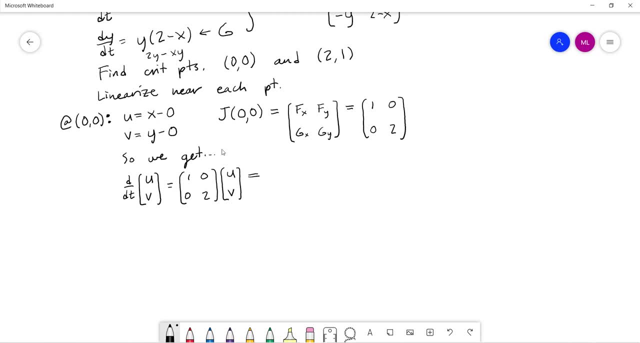 The eigenvalues will tell us what the behavior looks like. So in this case, I can tell right off the bat. just looking at this. the eigenvalues that I'm going to find are going to be equal to 1 and 2.. 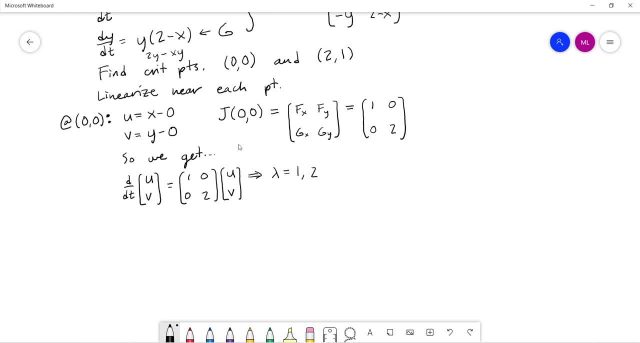 They literally are going to be these values sitting right here. Alternatively, we could actually go ahead and write that out if we wanted to, So We could be trying to find the determinant of a minus lambda i and setting it equal to 0.. 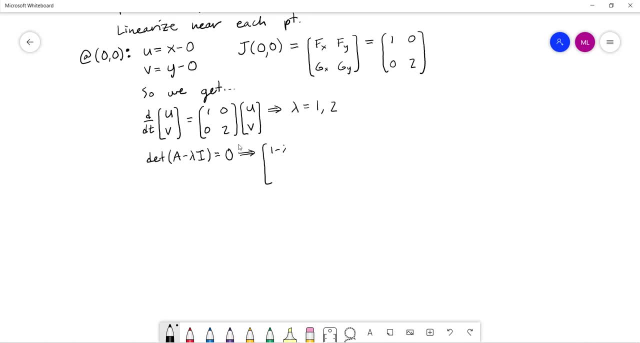 So we would get in this case right: 1 minus lambda, 0, 0, 2 minus lambda, And in fact let's write it like this: We're trying to find the determinant. Let me do the determinant symbols instead. 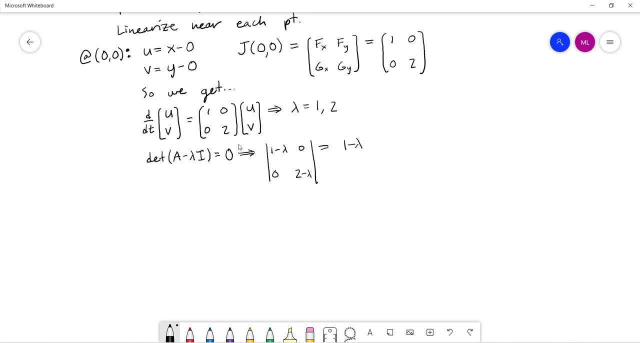 So I want the determinant, which will be equal to a 1 minus lambda. times 2 minus lambda is equal to 0.. So it's already factored And that's where we get the lambda equals 1 and 2 that I got up here. 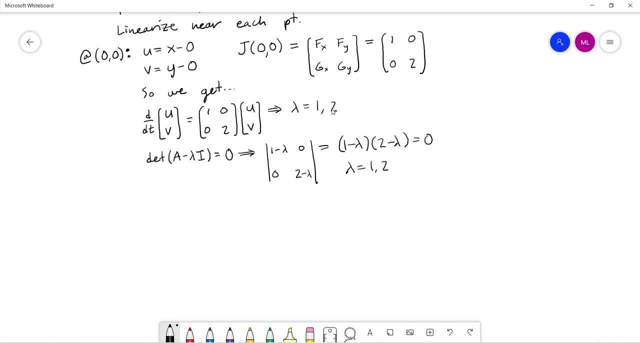 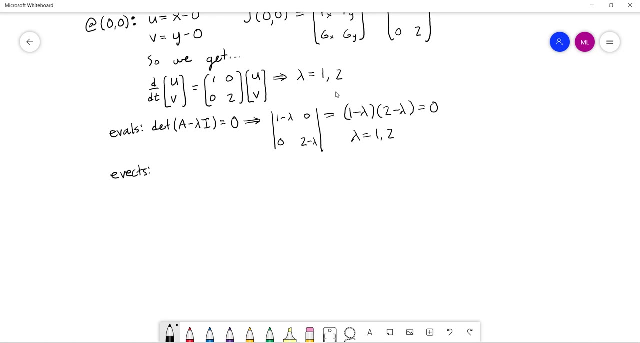 In this case, they are real and they are distinct, And so we'll want to find the associated eigenvectors, associated with these. So we find the eigenvalues. Now let's find the eigenvectors, Just abbreviate them like that. 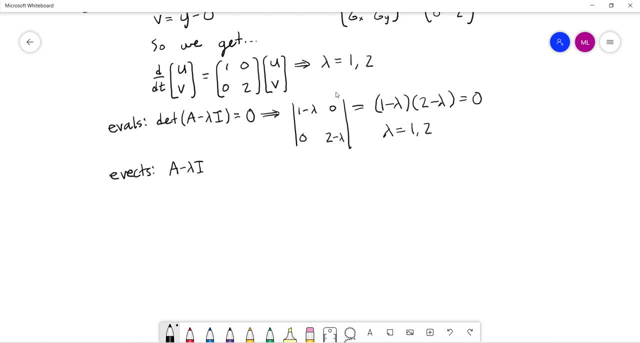 To find the eigenvectors. we want a minus lambda. i times e to the power of 1 minus lambda, So that's where we get the lambda equals 1 and 2 that I got up here. In this case they are real and they are distinct. 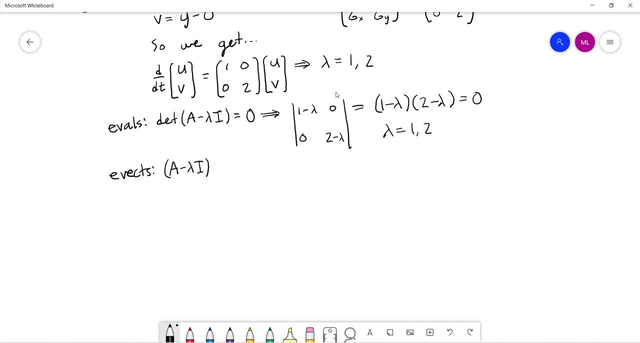 So we're going to find the eigenvalues, So we're going to find the eigenvalues of these. So the eigenvalues of these are going to be x v u, whatever you want to call it- x v u, whatever we want to call it k. I think we've done in the past. 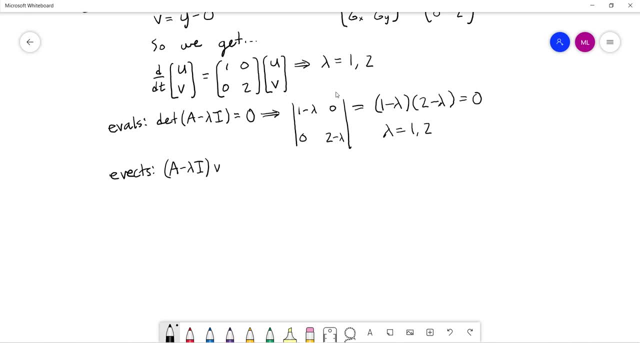 Let's just call it v. I've already used v, Let's do whatever k. k equals the 0 vector. So what happens if I were to plug in lambda equals 1?? What does the lambda equals 1 case look like? 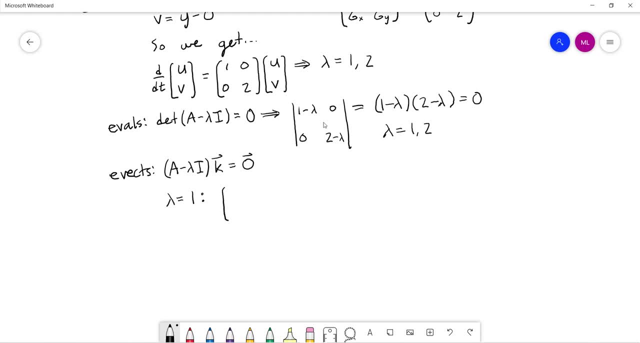 1. 2. 3.. Well, our system: when lambda is equal to 1,, I'll plug in 1 in these two locations and I will get 0, 0, 0, 1 times k1 and k2.. 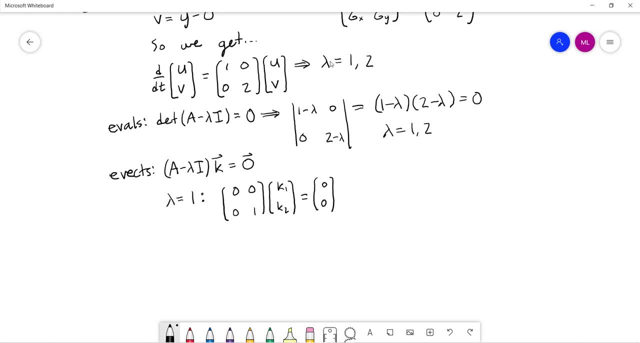 The two entries of the vector I'm trying to find is equal to 0, 0.. And in this case it looks like the only thing that's required, right? the first equation: 0 times k1,, 0 times k2, they're both 0.. 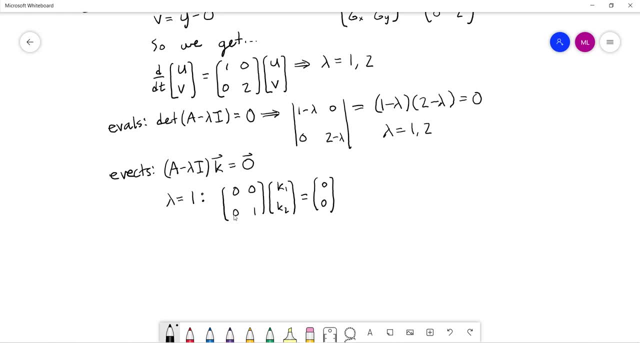 It doesn't give me any restrictions, But on the bottom it looks like all I need is 0 times k1 plus 1 times k2 to be 0. That means k1 can be anything because it's getting hit with a 0, but k2 has to be 0. 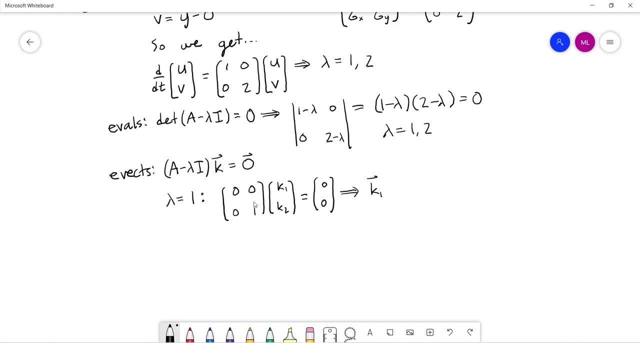 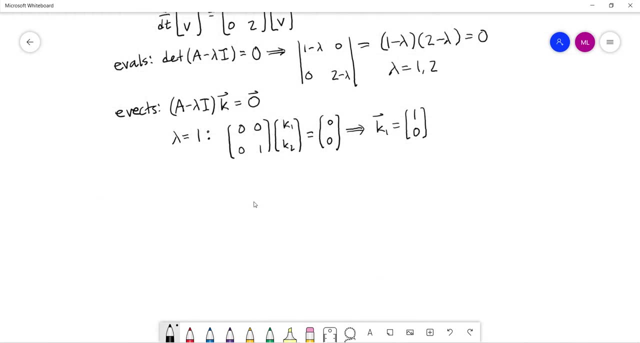 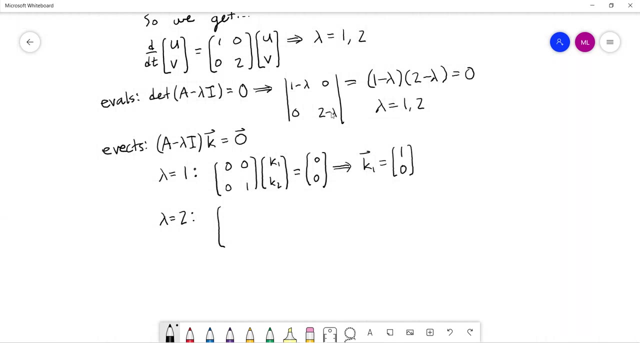 So the easiest way to pick out our eigenvector k is to pick something like 1, 0. That would be a simple one to pick. If we look at the other eigenvalue and plug that in, 1 minus 2 will give me a negative 1.. 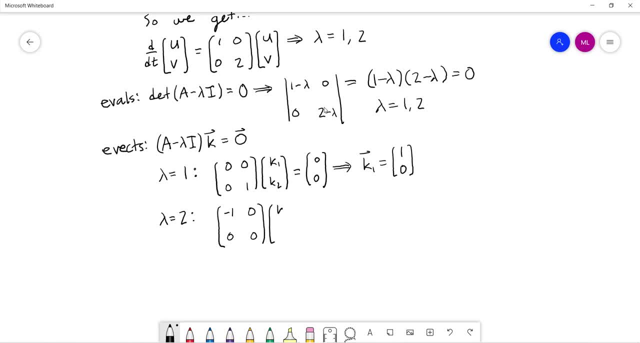 I'll have 0, 0, and 0. in those locations, times, its vector is supposed to be equal to 0, 0.. And so we get for our second eigenvector, same thing. In this case, the second equation gives us no restrictions. 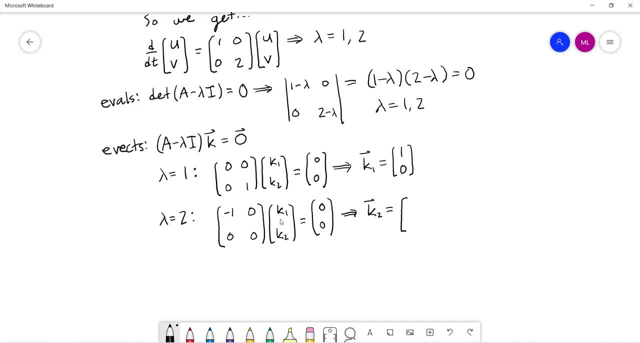 because both coefficients will be 0 times the k1 and the k2.. But the top equation tells us negative 1 times k1 plus 0 times k2 has to be equal to 0. So that means k1.. k2 can be anything, but k1 needs to be a 0 because it's getting hit with this negative 1.. 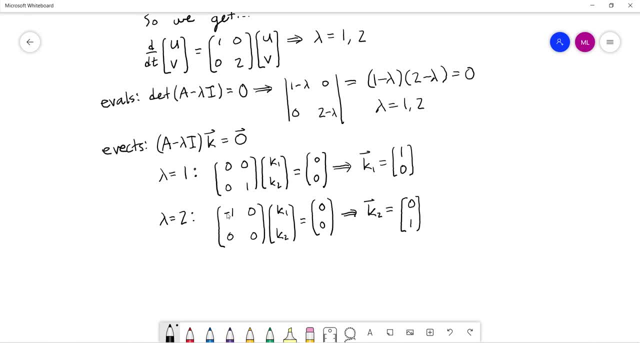 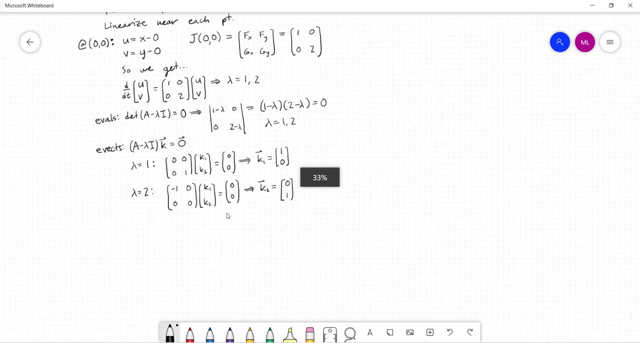 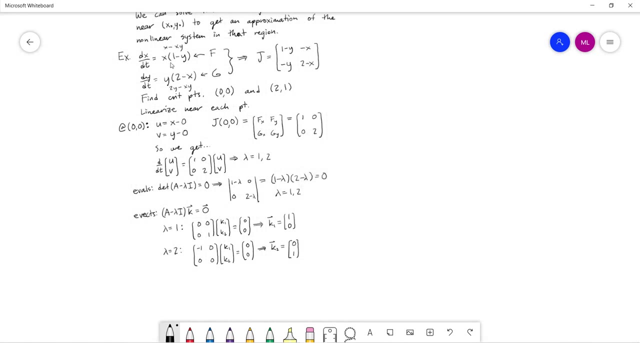 So 0 and 1 would be an easy one to pick, And so these are my two associated eigenvectors If we want to start drawing our solution. so I want to figure out the behavior of this system by looking at its phase diagram. 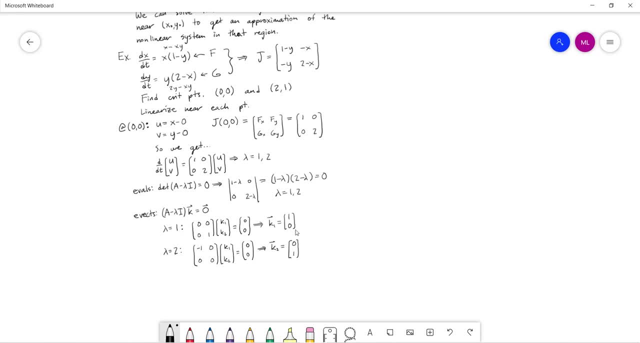 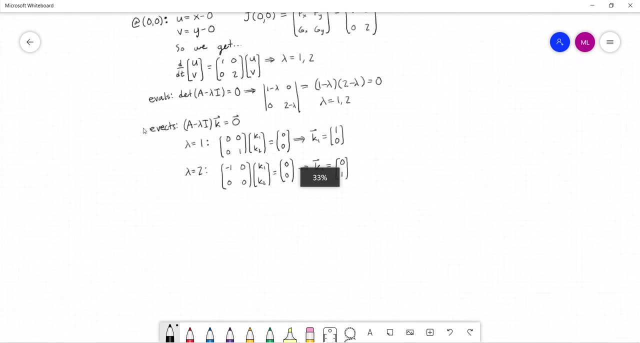 So that's what we're going to do And so far I have information. I have information about what the behavior looks like near, in this case, the origin. So let's do the other point. The other critical value was the point 2, 1.. 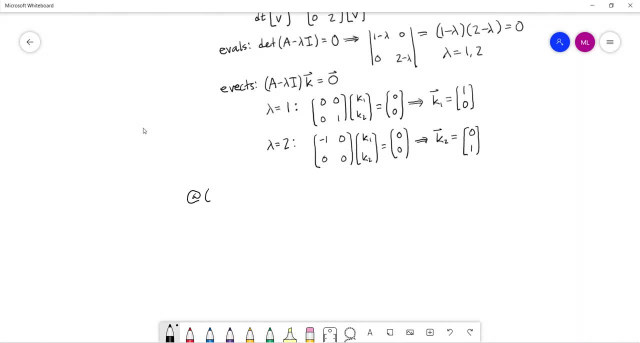 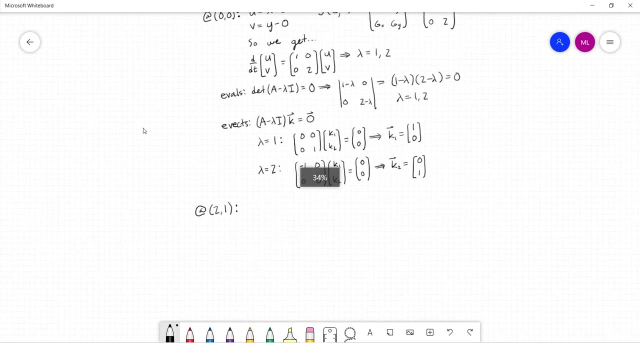 So at that point 2, 1,, what's going on? So at 2, 1.. So at the point 2, 1, again, I need to change my variables. u is going to be now x minus 2, and v will be equal to y minus 1.. 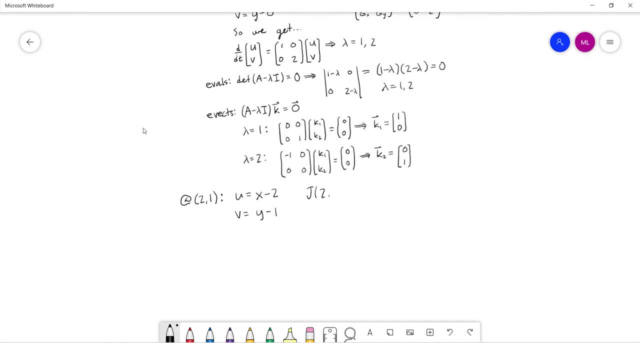 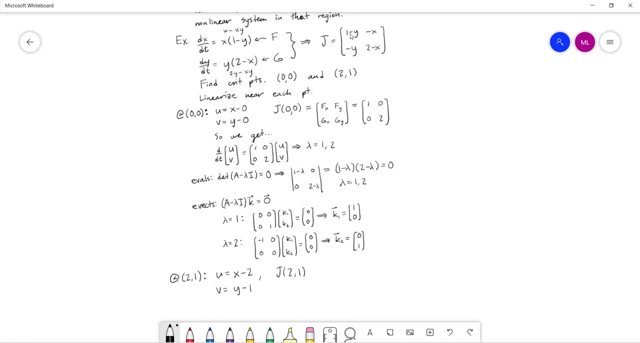 And the Jacobian At that point, the Jacobian at the point 2, 1 helps to have it all on the same screen if possible. So it's right here, right: 1 minus y. negative x. negative y 2 minus x. 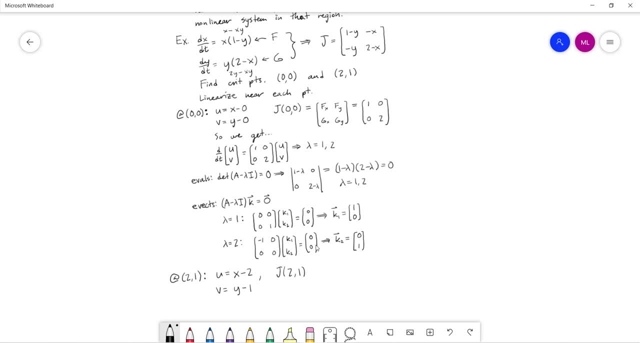 But we're plugging in these two points for x and y now, So that Jacobian is going to be equal to. Let's see, So y was equal to 1.. So this is going to be 1 minus 1.. That's a 0.. 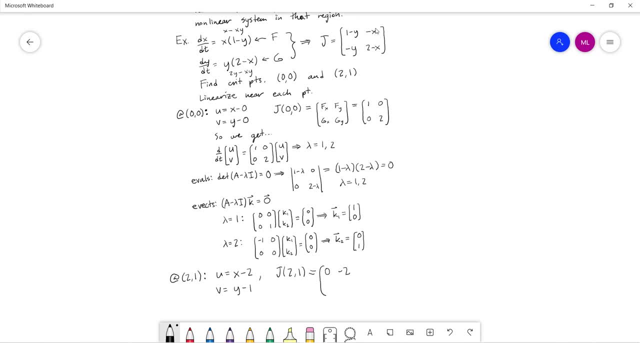 Negative x- x was 2.. So that's a negative 2.. Negative y- y was 1.. So that's negative 1.. And then 2 minus x- x was 2.. So that is a 0 there. 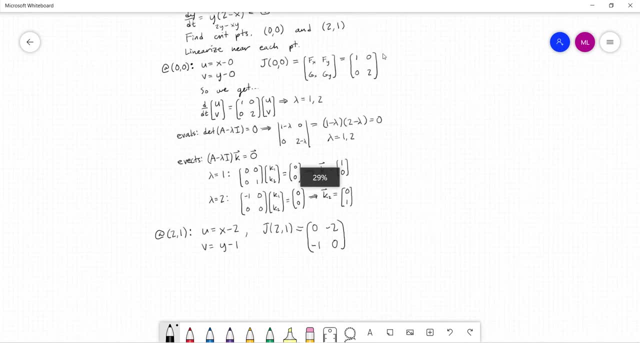 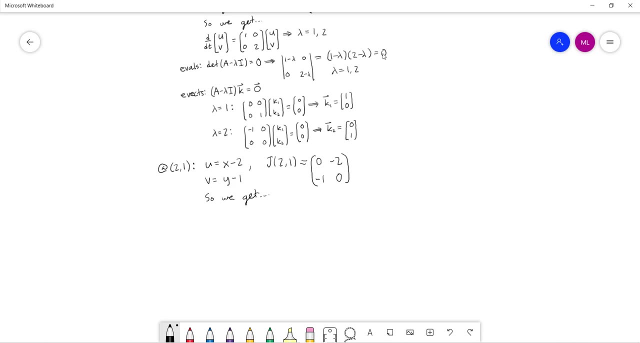 So there's what that Jacobian looks like And our linearized system. So we get d: dt of u times v is now equal to this matrix, So 0, negative 2, negative 1, 0.. times u and v. 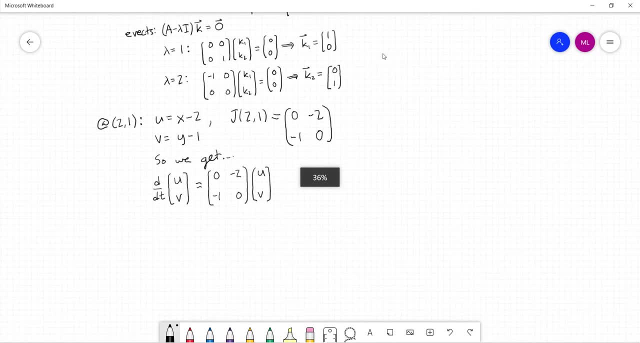 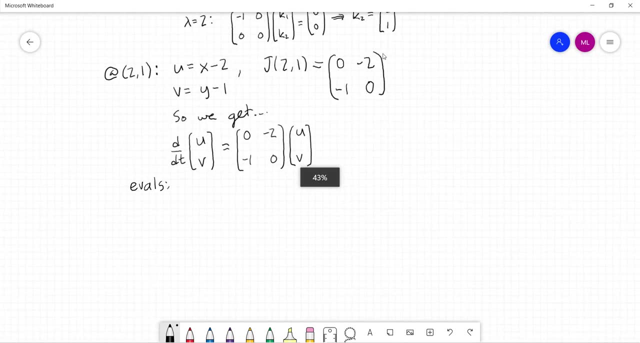 And this is the linear system that we're now trying to solve. So I need to find its eigenvalues. We'll do it the same way as before. The eigenvalues mean that I want the determinant of a minus lambda i equal to 0.. 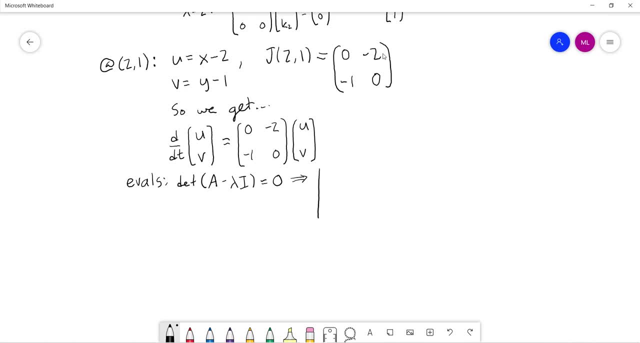 So for us that determinant is going to be a negative lambda. We're just subtracting lambda from the two diagonals. We've got a negative 2, a negative 1, and another negative lambda, And that's got to be set equal to 0.. 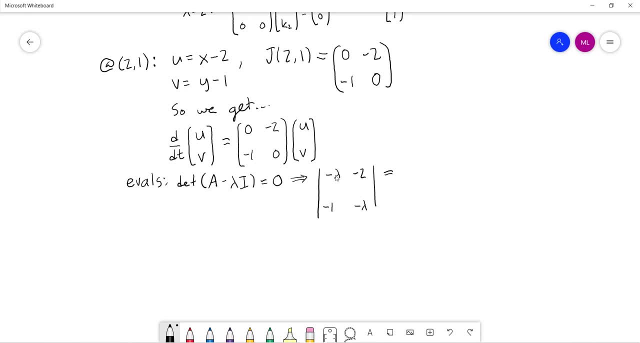 So when we take this determinant, it'll be this times this minus, this times this. So I'll get lambda squared minus, in this case 2 times 1.. So minus 2 equals 0. And in this case it looks like we get lambda 1 to be. 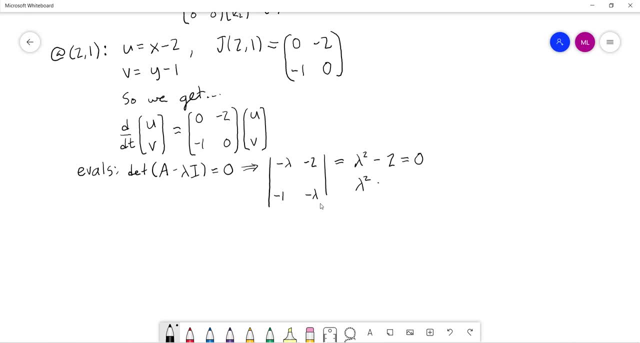 So basically, we subtract or add 2 over to the other side And we get that lambda is equal to plus or minus the square root of 2. Or so it appears. Okay, so we've got our two eigenvalues. We need the associated eigenvectors. 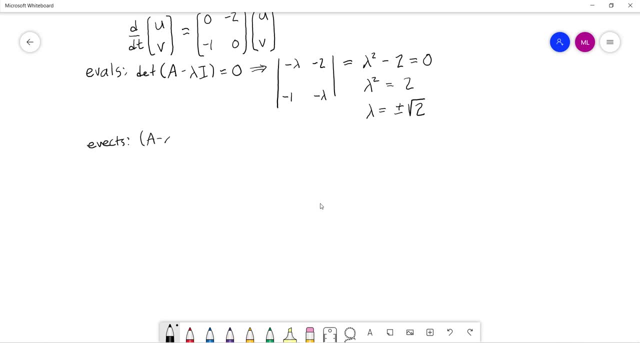 Which, again for the eigenvectors, we solve a minus lambda i times some unknown eigenvector. It has to be equal to the 0 vector And we start with the lambda equals positive root 2 case When lambda is equal to positive root 2,. 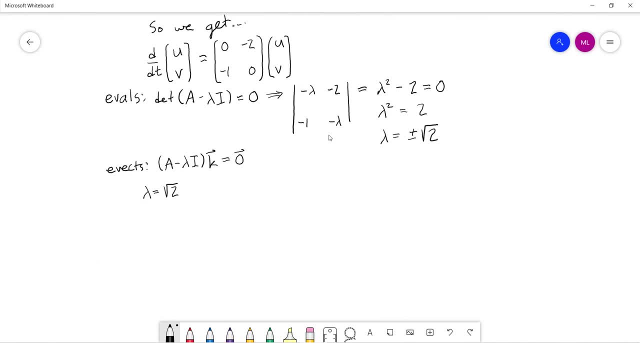 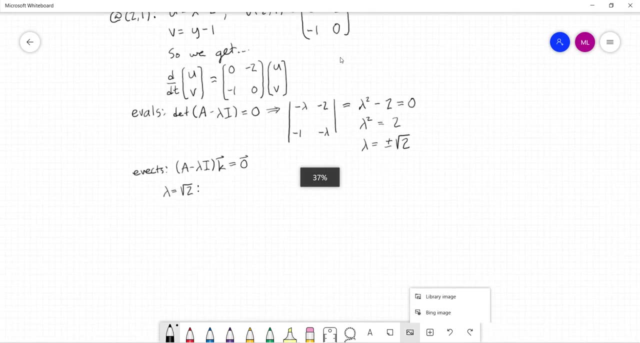 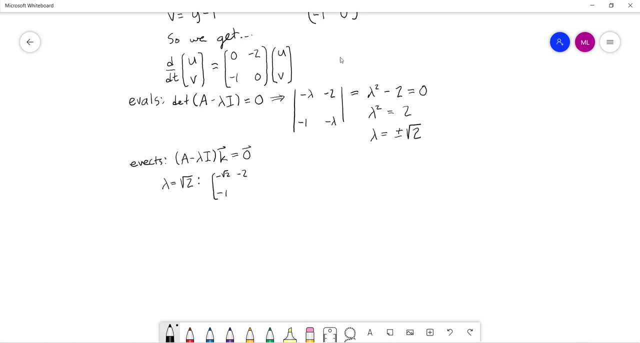 and I plug it into our a minus lambda i form of the matrix I will get. Let's see here. Let's make sure my formatting is kind of matching what I was doing before. Good, I will get negative root 2.. Negative 2, negative 1, negative root 2.. 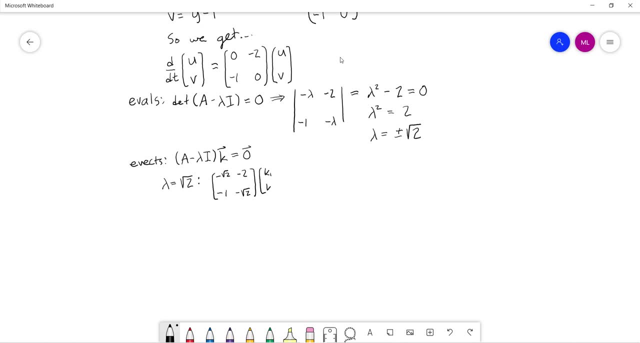 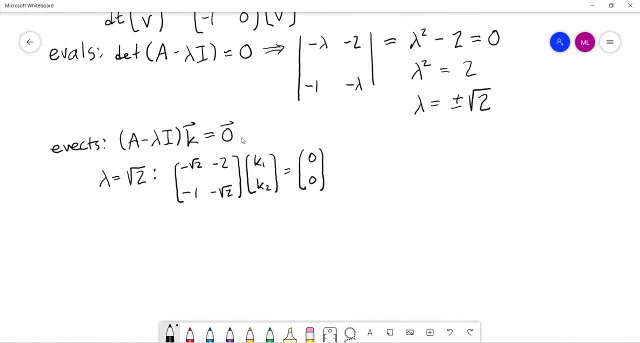 Times the unknown k1 and k2 has to be equal to 0, 0.. Okay, It may not look like it, but these two rows are in fact proportional to one another, right? This matrix is what we call singular. These two rows are not linearly independent. 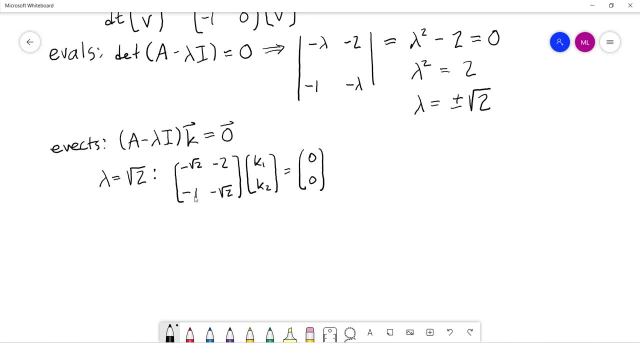 If I were to multiply the bottom row by the square root of 2,, then the negative 1 would become a negative square root of 2, and the negative square root of 2 would simply become a negative 2.. So if I multiply the bottom row by root 2,, 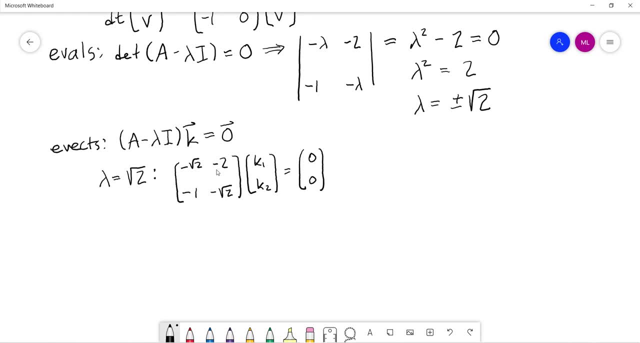 I get the top row, So I can use either one. We can pick and choose and find that the eigenvector associated with this is going to be: Let's see here. Let's pick this one because it's simpler. Remember, you just switched the order. 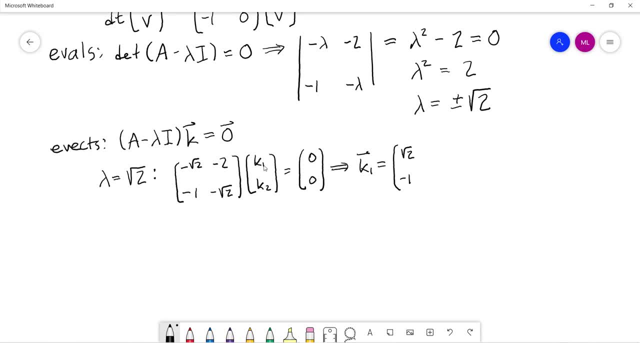 So I'm going to do a root 2 on top and a negative 1 on the bottom. So there's my eigenvector, right. I switched the two positions- First, second, Now it's second, then first- And I flipped one of the two sides. 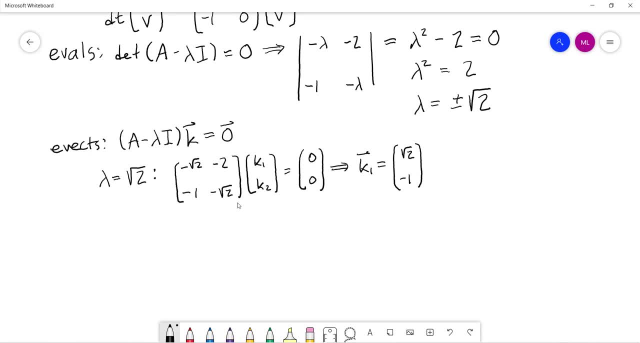 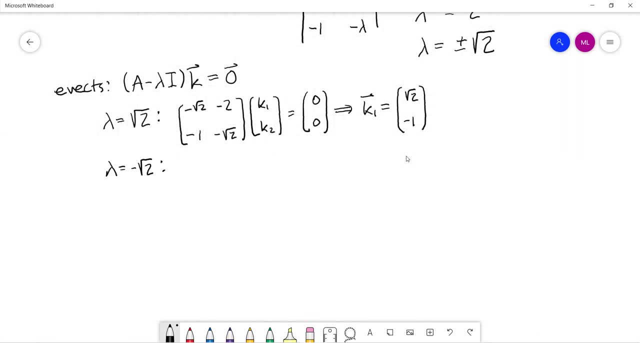 In this case, I chose to flip the root 2 from a negative to a positive. If we do the other one, we will now get positive root 2, negative 2, negative 1, negative root 2, times k1 and k2 is equal to 0, 0. 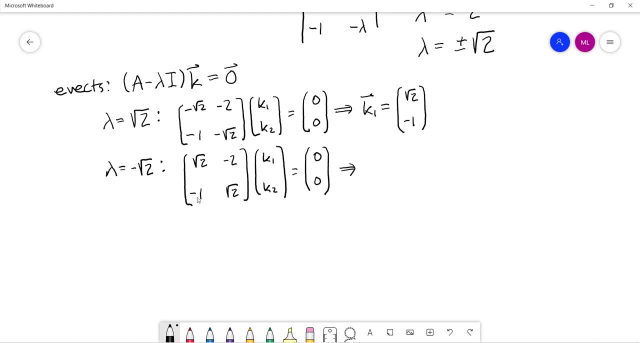 And again same argument. Now, if I multiply this one by negative square root of 2, I would get root 2.. And if I multiply this by negative square root of 2, I would get this. And so same thing, the bottom one. 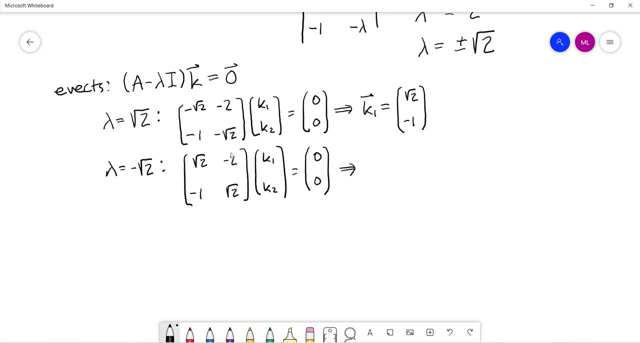 if I multiply the bottom by the negative square root of 2, I get the top, And that tells me that my second eigenvector is going to be negative square root of 2.. I can pick either of those two rows to use. 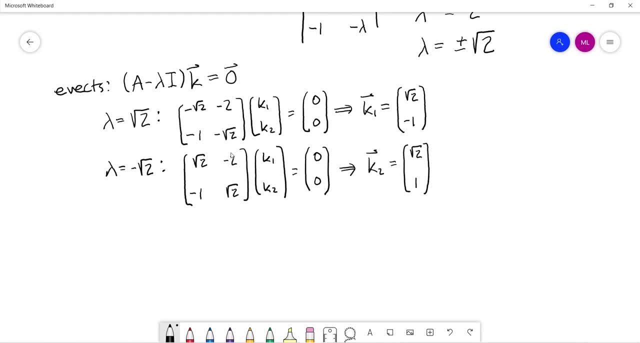 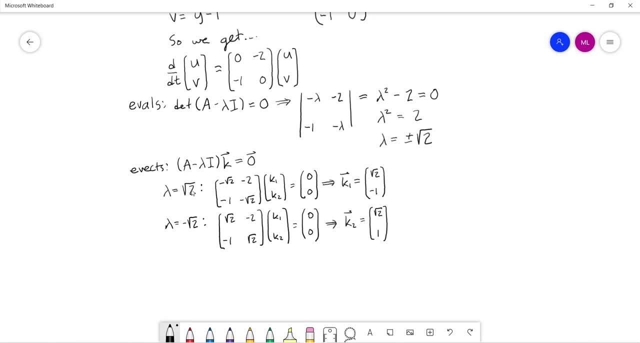 I'm going to do the same one, root 2, and now a positive one down there, And so we can write out the individual solutions. but those solutions aren't valid universally, right, We could solve for what the solution looks like here. 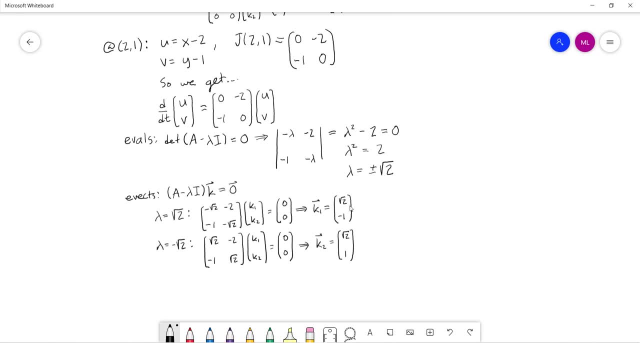 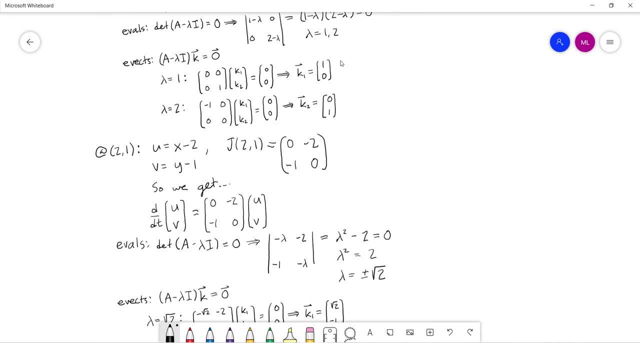 It's going to be an exponential with one positive exponential, one negative. decaying exponential times, these particular vectors. similar thing over here, these two positive exponentials, But it doesn't give me the big picture. It only tells me the picture immediately in the vicinity of 2, 1. 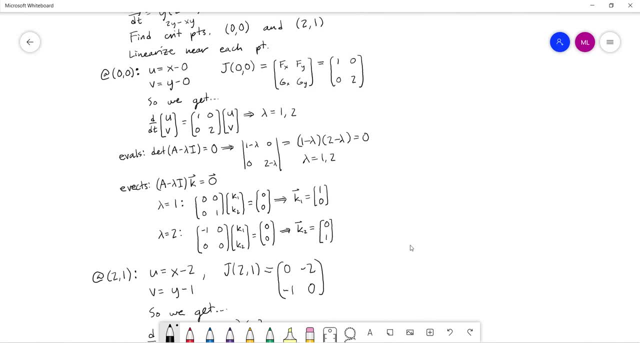 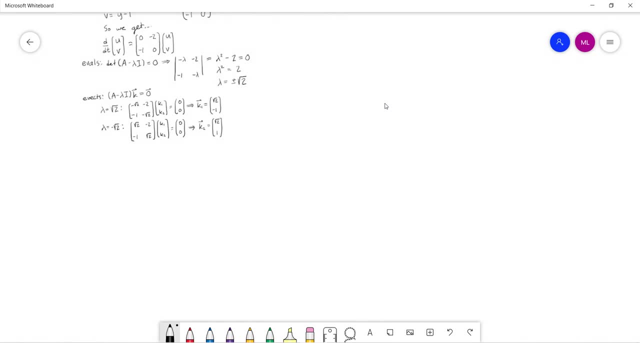 or immediately in the vicinity of 0, 0 in the two cases respectively. We want to get a sense of what the whole thing looks like, So let's put these together, Let's draw the phase diagram or the phase portrait, And so the easiest way to draw the phase portrait? 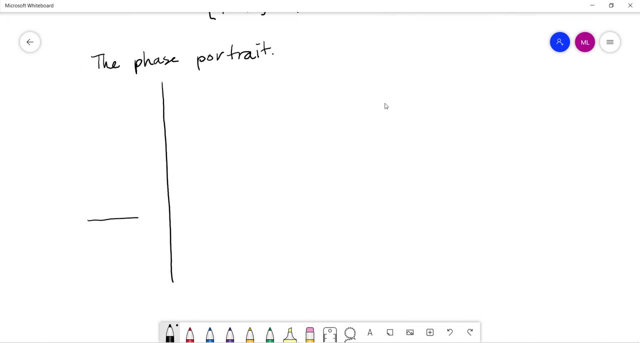 is start off. remember, we are trying to plot, in this case x versus y, And we found two critical points. One was at the origin, So I'm going to draw that one in, And the other one was at the point 2, 1.. 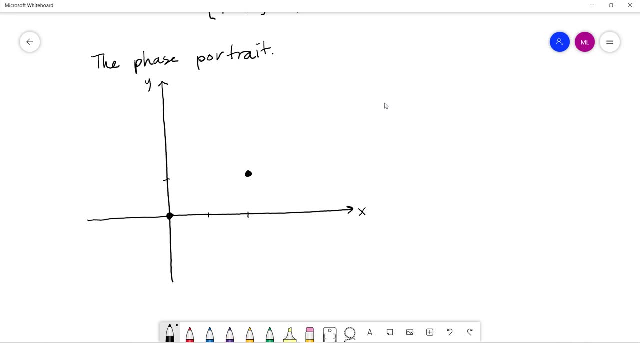 So it's right here. Here are our two critical points And I basically want to, at each of these two points, draw the phase portrait associated with the solutions that we found. So let's start with the one near the origin, near 0, 0.. 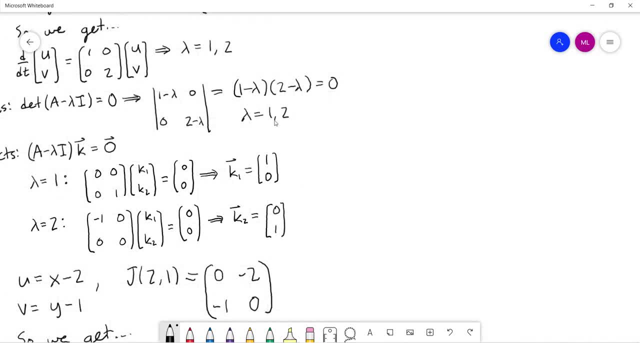 The phase portrait, for this is going to be a node. It's an unstable node because my eigenvalues are both positive and it has these two eigenvectors, So 1, 0 and 0, 1.. So my two eigenvectors in this neighborhood. 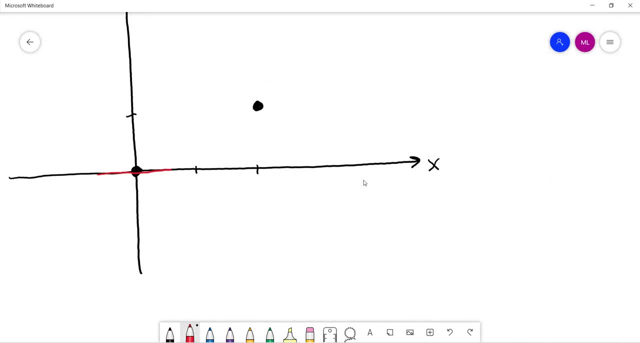 let me draw them in color. One goes in this direction and one goes in this direction. Oops, Let's not erase that. So the two eigenvectors are: one goes in the 1, 0 direction, the other one goes in the 0, 1 direction. 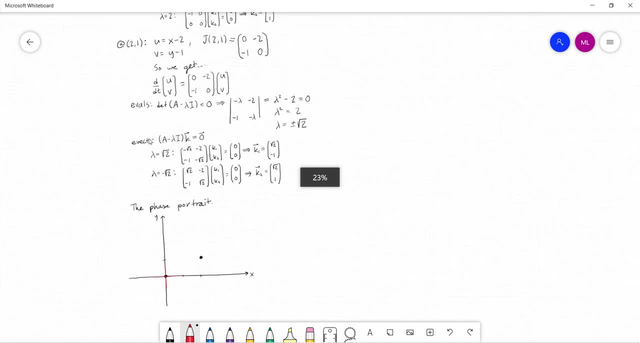 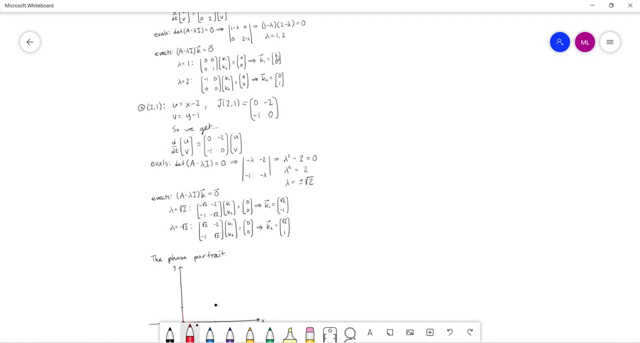 Which was which. So again, sorry to have to scroll up and down. so much The 1, 0,. so the horizontal one, the one that went in the direction of the x-axis, that's associated with an eigenvalue of positive 1.. 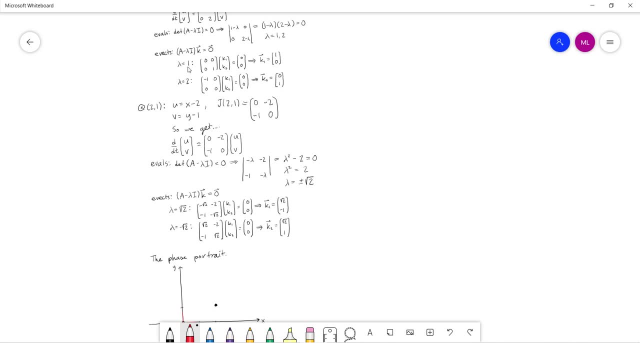 And so for large negative values of t. basically, if we go to negative values of t, we're going to start off parallel to this direction and we're eventually going to move to be parallel to this other direction. So we're going to start off basically with curves. 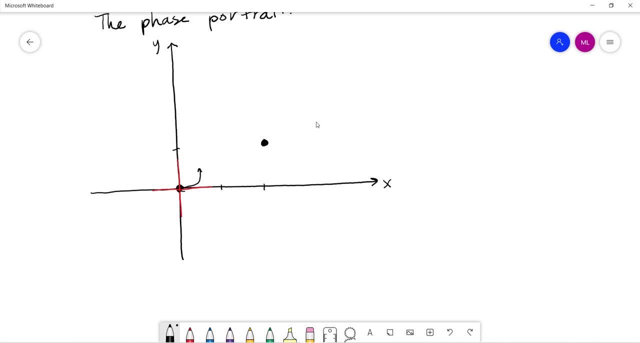 that kind of go out in this direction and eventually start to go kind of up in this direction And we're going to have similar types of curves out here. This is kind of the picture that we're getting in this neighborhood. This is an unstable node. 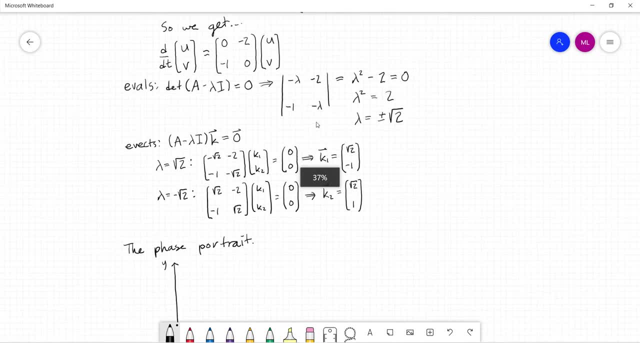 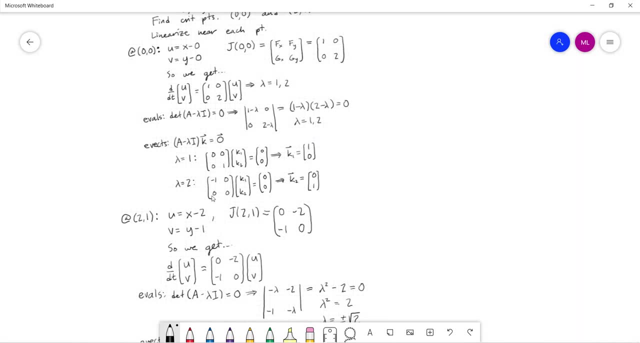 So basically, again, stuff is going out. It kind of starts more parallel to this vector and winds up parallel to this vector because of their association with the smaller and larger eigenvalue in this case. So that's what we're going to get there. 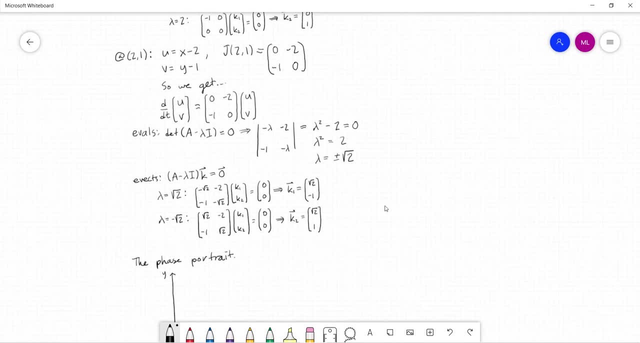 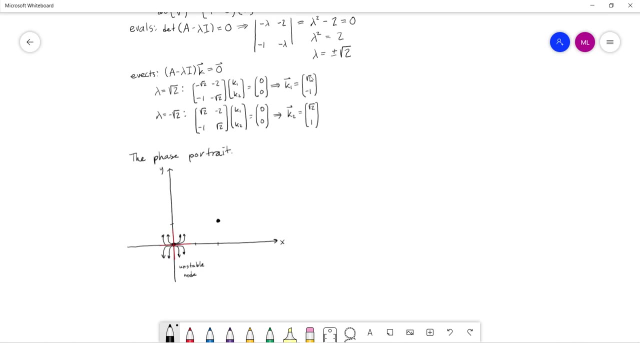 Now let's go look at the other one In the vicinity of this one. what do we have? We have a root 2, negative 1 vector and a root 2, positive 1 vector. So root 2 is about ballpark 1.7,. 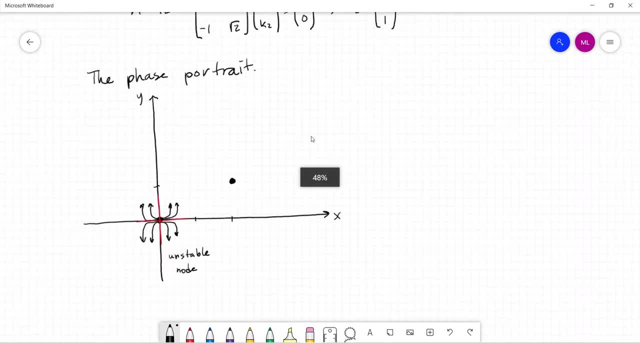 so it's certainly bigger than 1.. So it's saying: in the vicinity of this one I'm going to go over about 1.7, and in one case I'll go up 1.. So one vector is going to go kind of in this direction. 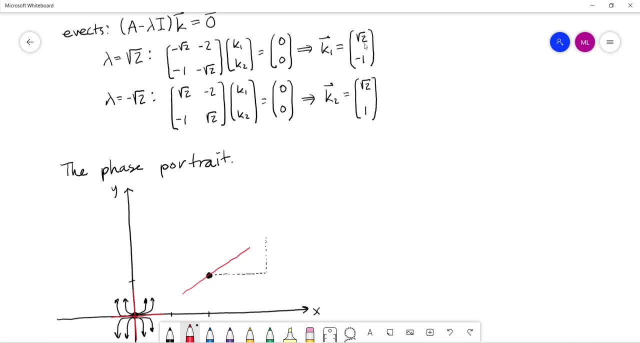 And then the other one is root 2.. So that's root 2, positive 1.. I've drawn that one. The other one is root 2, negative 1.. So the other one's going to go basically in the mirror image of this. 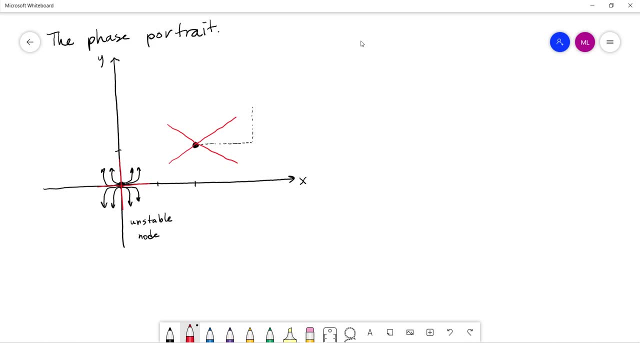 kind of downward in that direction. So those are kind of the eigenvector directions around. the second point- assuming I didn't screw anything up here- And in this point we also have one positive and one. So in this case we have one positive.